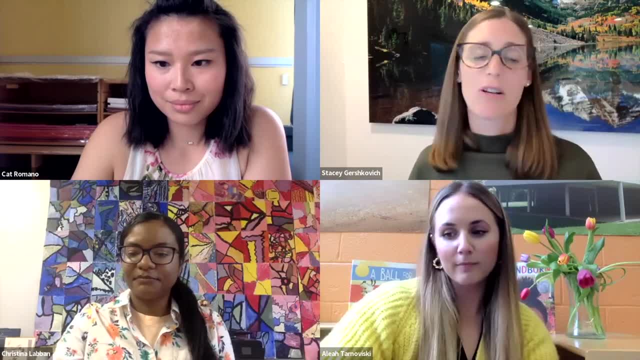 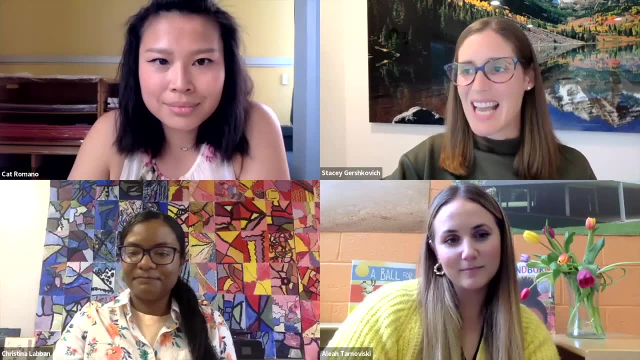 we've got our chat and we would love to hear who you are, where you're coming from and what you're doing. Thank you so much for joining us. What you are interested in talking about today. we have a lot of great info for you today. 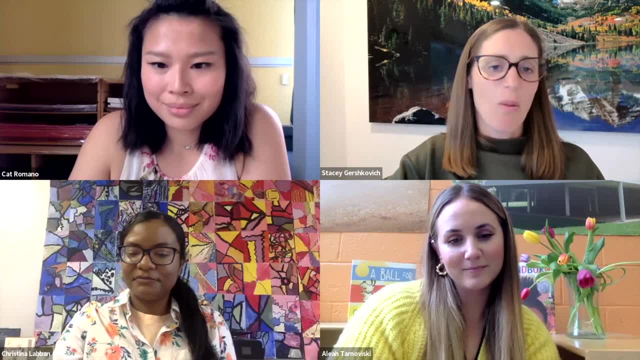 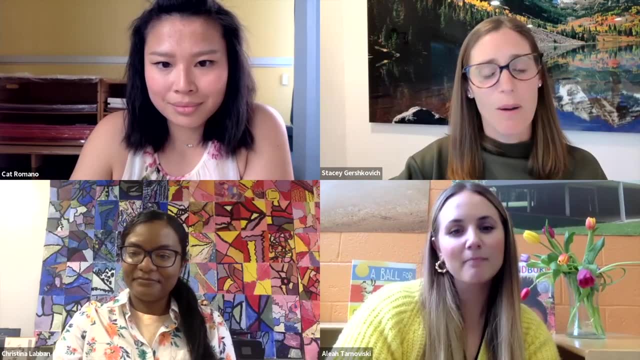 Hoping that you walk away from today's webinar feeling really excited about this kindergarten journey that you're about to embark on, as well as really confident that you are prepared and that your child is prepared, and that it's going to be a great year If you can get started by. 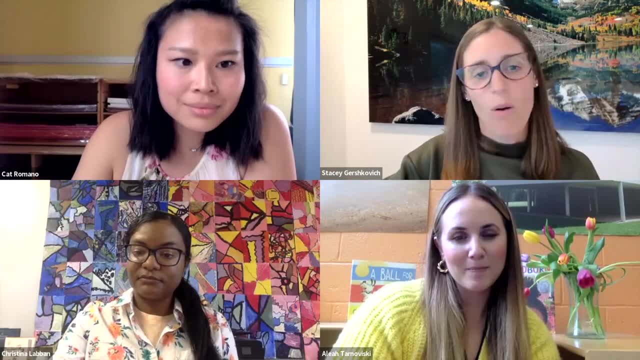 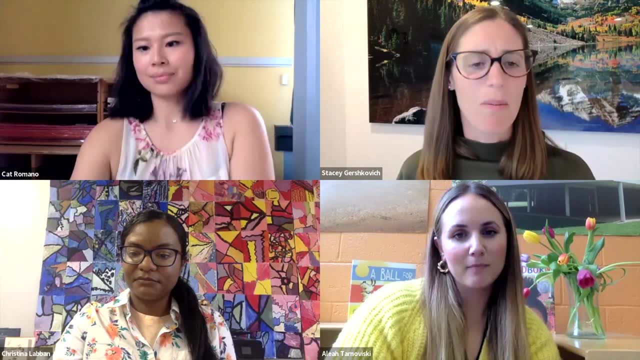 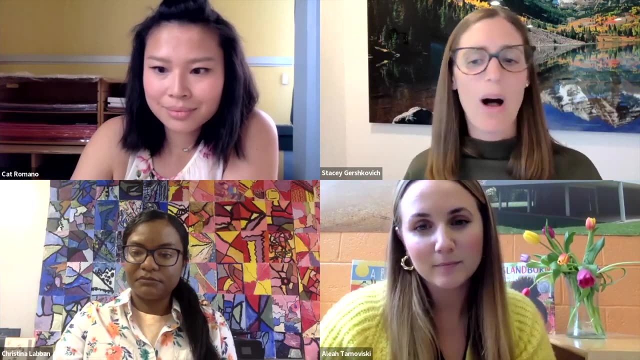 introducing yourself in the chat. what makes you most excited or nervous about sending your child to kindergarten and what do you think kids need to be able to do to be ready for kindergarten? What does kindergarten readiness mean for you While you're going ahead and 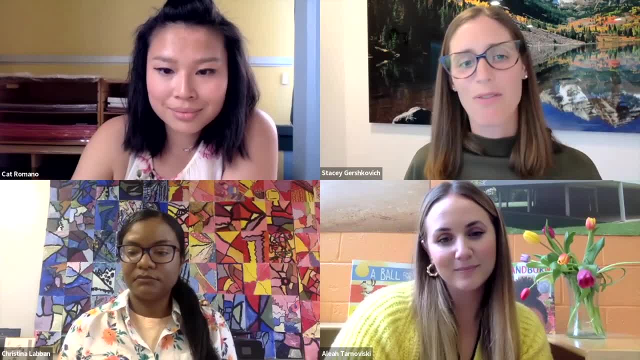 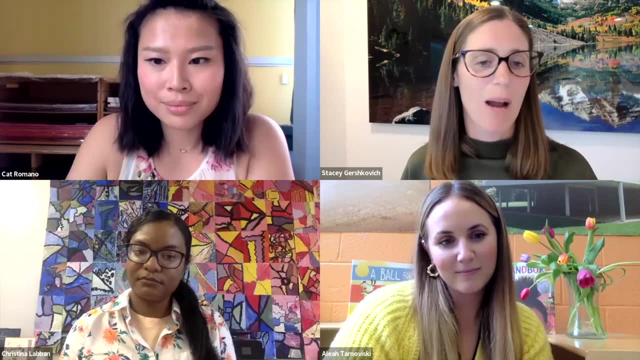 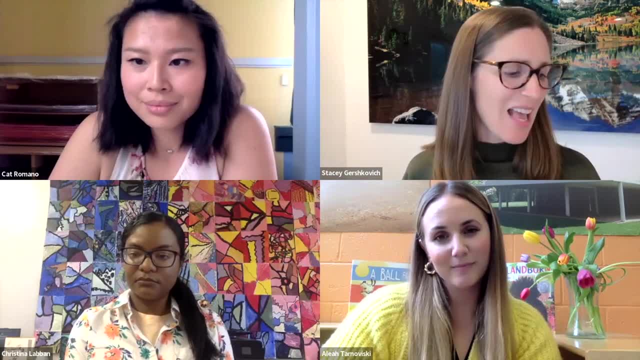 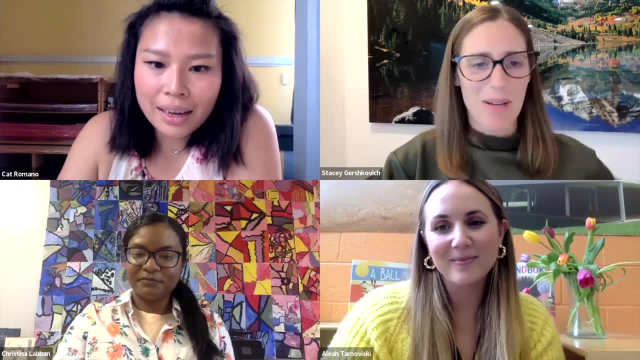 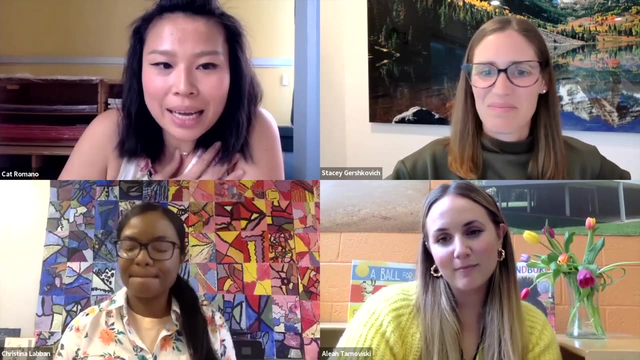 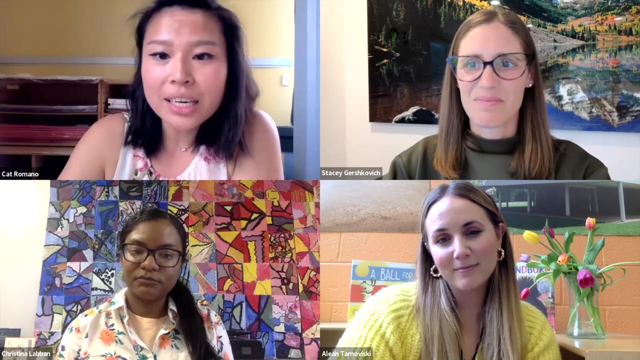 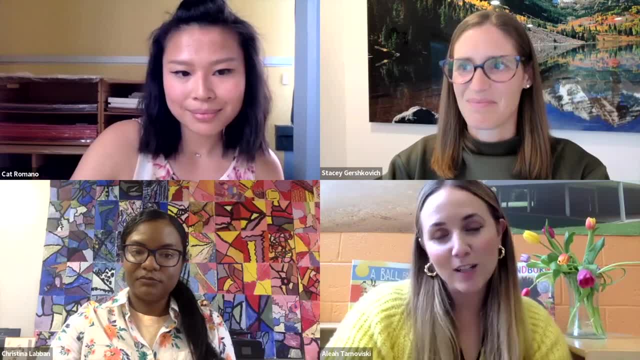 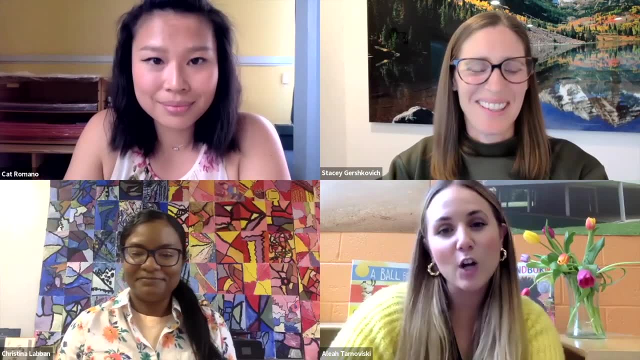 My name is Alia Tarnavisky. I've been a teacher at Success Academy for the past 10 years and I love teaching kindergarten, so I'm excited to talk about all the things that you can be really excited about for the upcoming school year for your child. 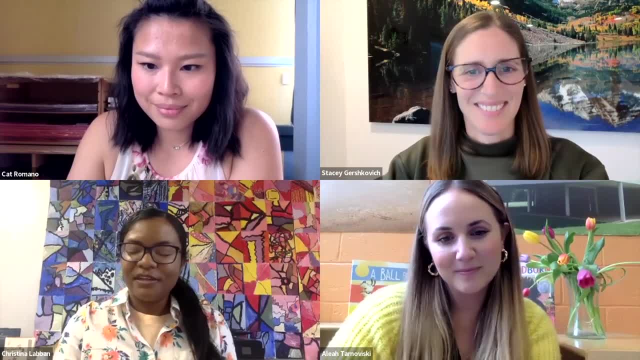 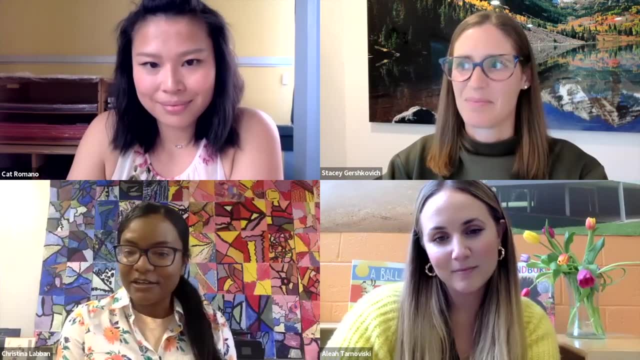 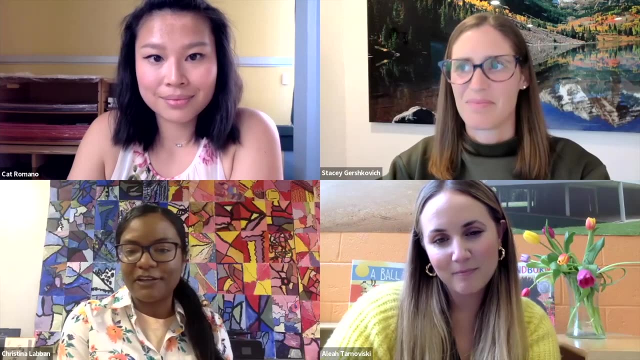 Hi, I'm Christina Laban. I work also at Success Academy at Springfield Gardens. I've worked there for six years. I've been in kindergarten for six years and I love it. I love seeing the kids be successful and just learning a lot. so really excited to join you guys today. 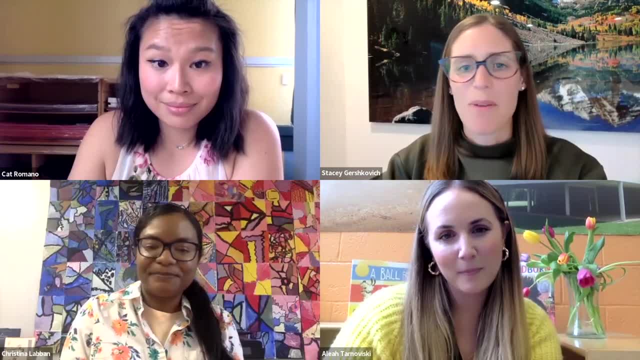 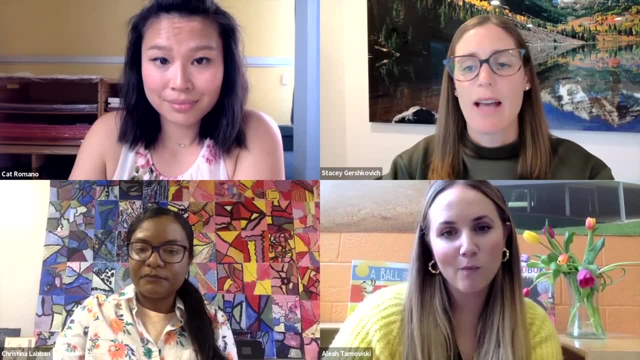 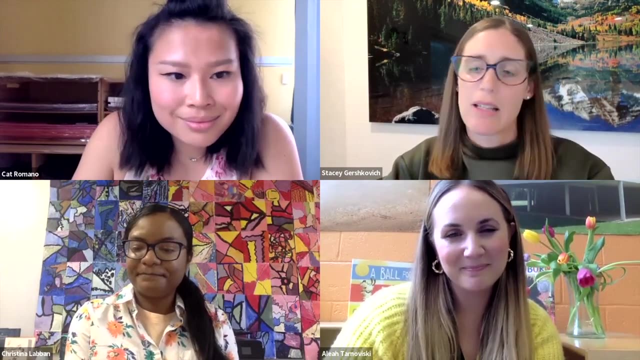 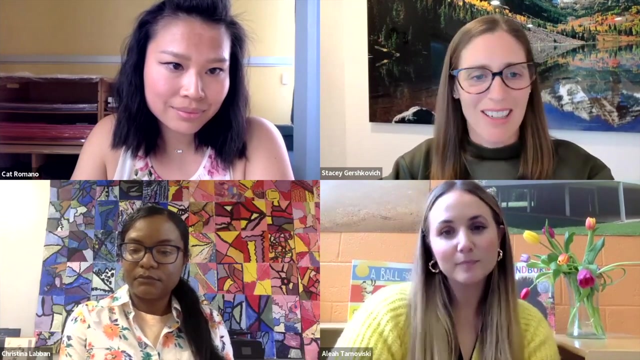 Great, I love that. you guys are jumping right into the chat, so please go ahead and do that. It is totally up to you. if you want, You have an option of sending your chat. You can send your chat to everyone- There's a little blue button on the bottom right- or you can just send your chat to the host and panelists. so that's up to you. whatever you feel comfortable with. I'd encourage you to send it to everyone, because we'd love to get a sense of who else is out here and who else is in a very similar position as you. 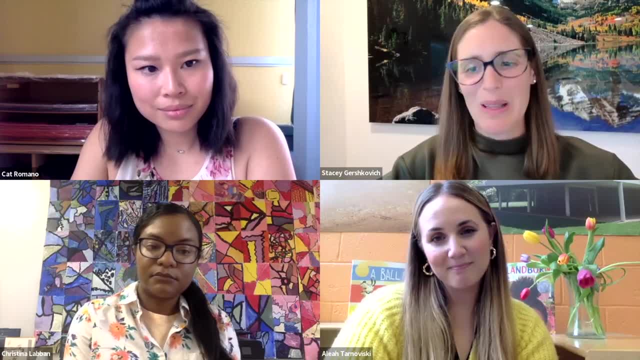 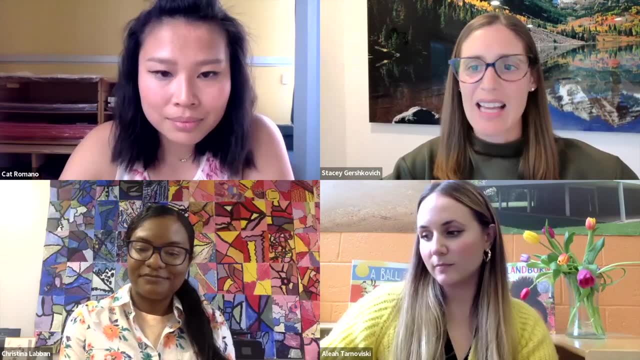 I think sometimes we feel just better, knowing that we are not alone in the way we are feeling and the thoughts we are having. but I'll leave that up to you. I see we have a lot of families who are joining us at Success Academies and we have a lot of families who are joining us at Success Academies, and we have a lot of families who are joining us at Success Academies. 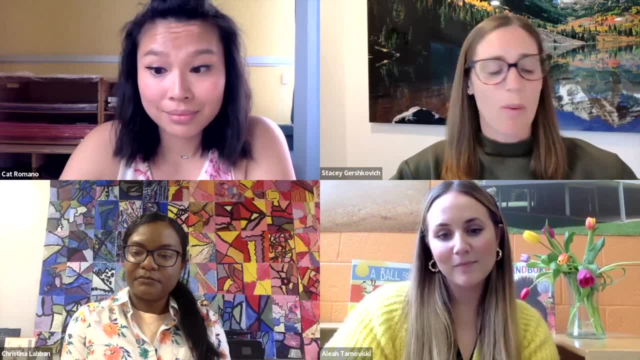 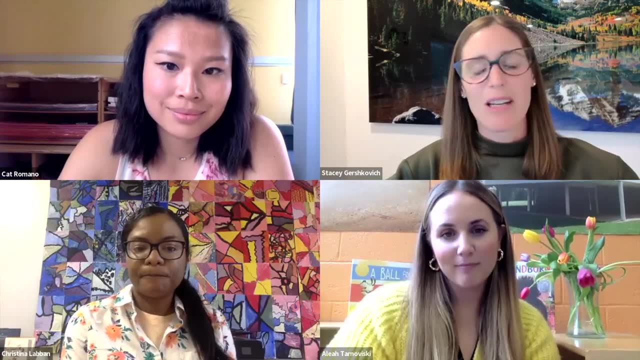 I see we have a lot of families who are joining us at Success Academies and I just want to make sure you know all of this content will be relevant, no matter where your child is going to school next year. We're super excited to have you, and I know we've got some educators on the call and some folks who are involved in education in other ways, so welcome all of you. 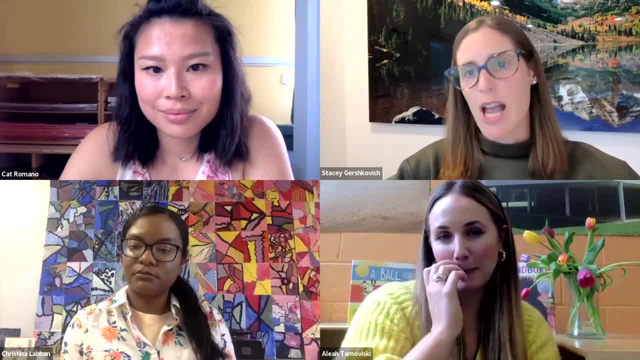 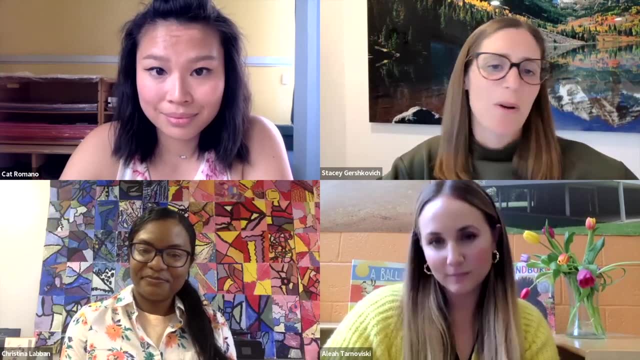 We really hope to make the most of this time. so again, use that chat, use that Q&A. So let's get started. Ladies, first of all, before we get into it, what is the purpose of kindergarten from your perspective? 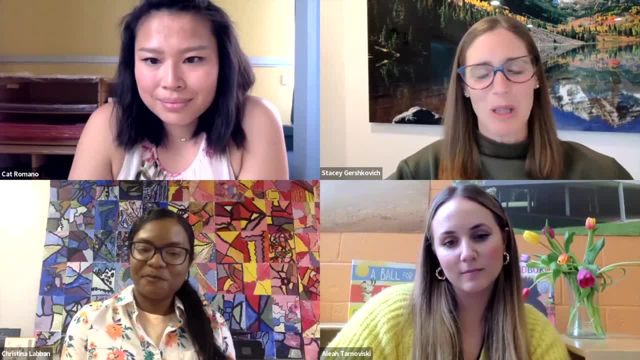 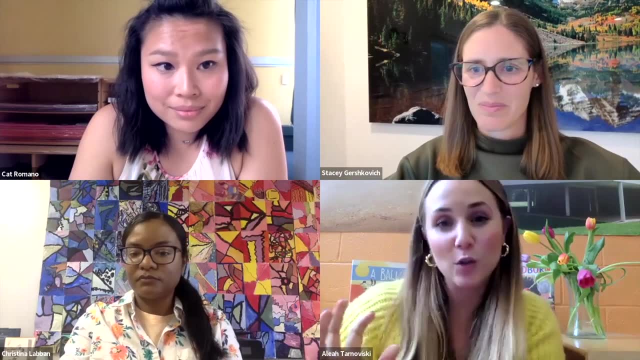 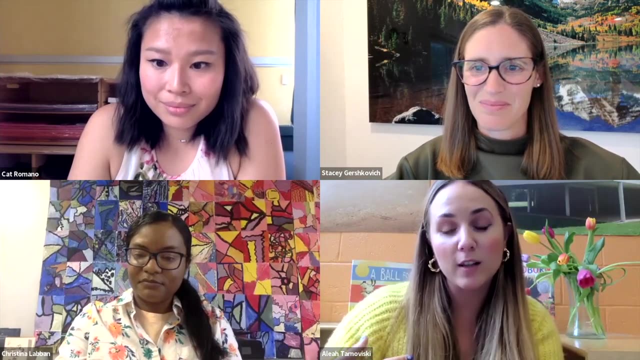 And I know it's a big question. so give us one or two thoughts. What is the purpose of kindergarten? I think the purpose of kindergarten is like to be introduced to the magic of school and the magic of learning, and I really think it's the place where kids fall in love with learning and with school. so it's that like first taste of it. 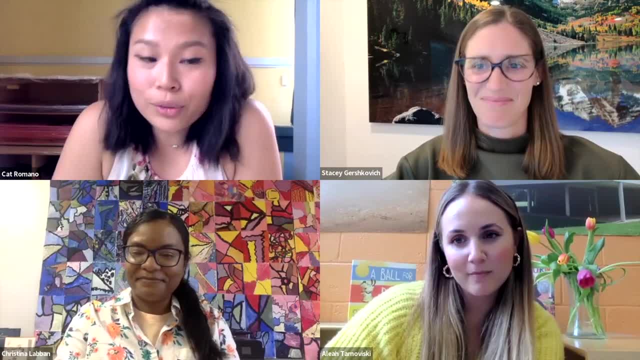 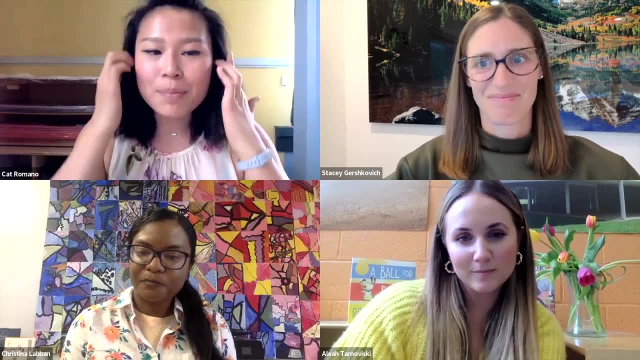 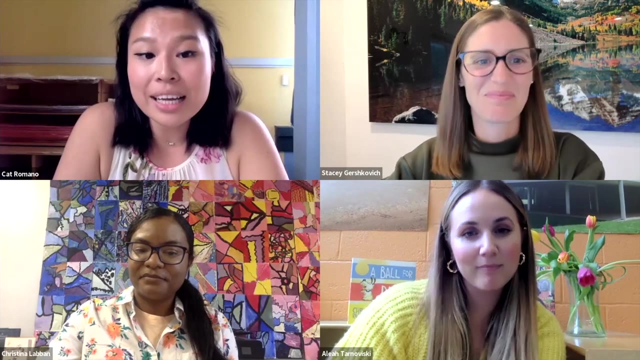 Yeah, I think you know, as I'm seeing in the chat, you're kind of just thinking about all these things like what does my kid need to know before they come? What should I be working on? But really just hyping up your child or, if you have twins, or going into kindergarten, just getting excited to learn and to be around other children. 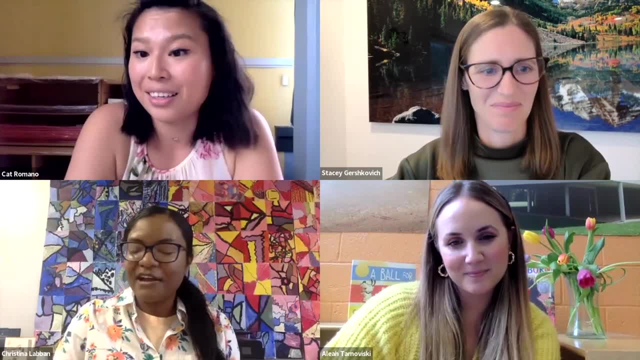 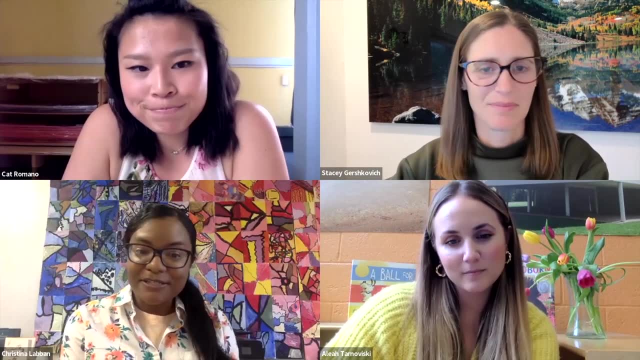 It's going to be a magical year. Yeah, to echo what the ladies have been saying, it's definitely setting the foundation for their learning journey. It helps them really get excited about going to school and they start to learn social skills. so it's really just setting the foundation. 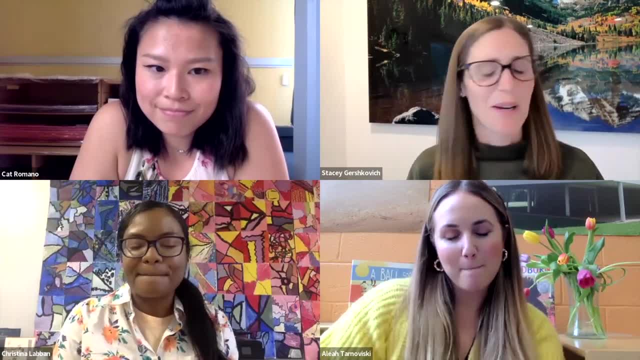 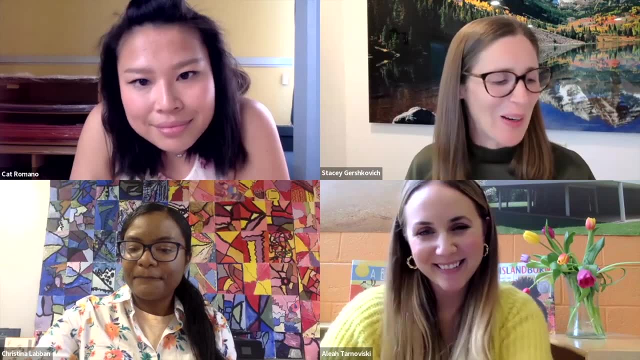 It's really just setting the foundation for the rest of their learning career. This is great. I'm so excited to dig in and I should mention my youngest of three is starting kindergarten this year, so this topic is near and dear to my heart. 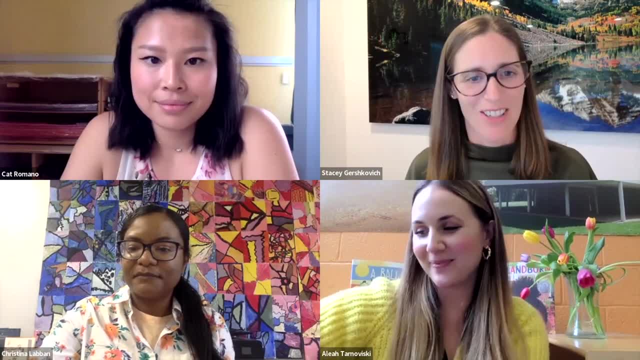 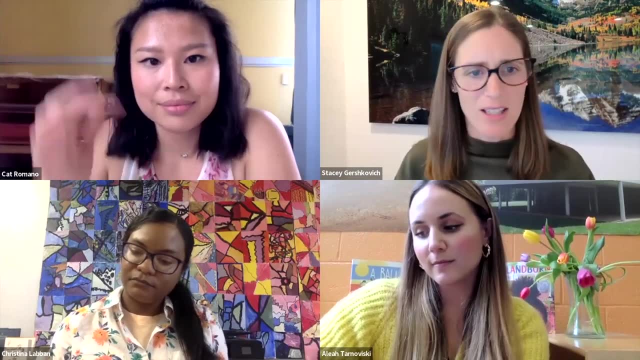 In fact, this is the time of year where all of my mom groups start kind of having this conversation of my child doesn't know how to do this yet. Should I be worried? My child can do this. Is this enough? Are they ready? What should I be doing? 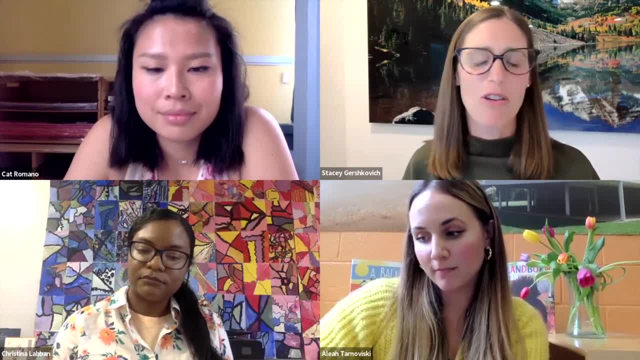 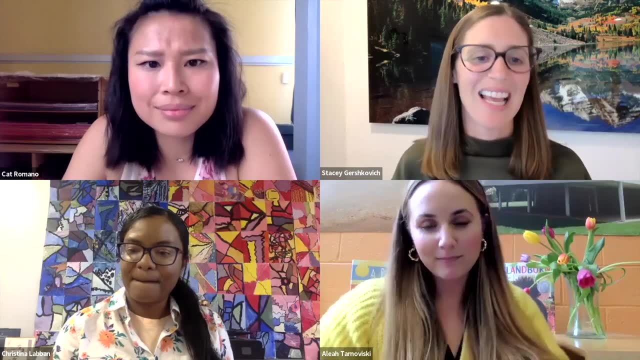 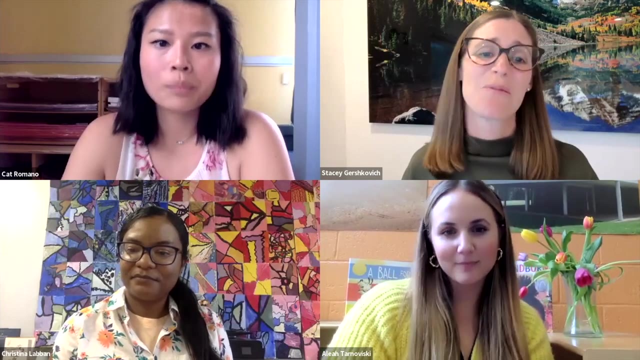 And so, again, the hope is today we'll be able to answer all of those questions and I'm so really confident that you are ready for kindergarten and your child is ready for kindergarten and get really excited. And again, that's the purpose of one of the purposes of kindergarten is just to get kids really excited about learning and the start of their school year. 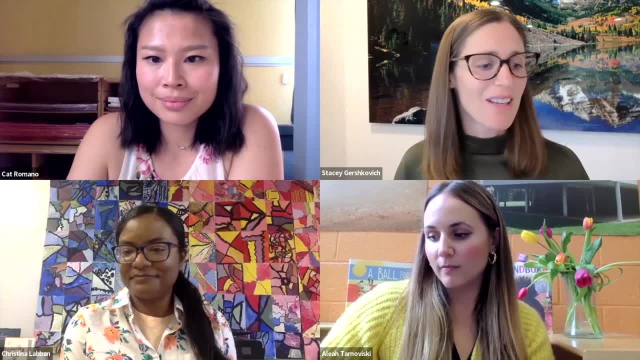 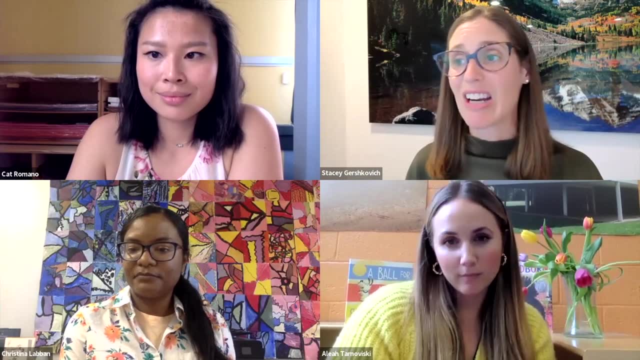 So one of the things that we're very aware of is that, particularly in this past two years, we haven't had the opportunity necessarily to be in the schools as much as we typically are, And so, before we go into that, I just want to say thank you so much for joining us. 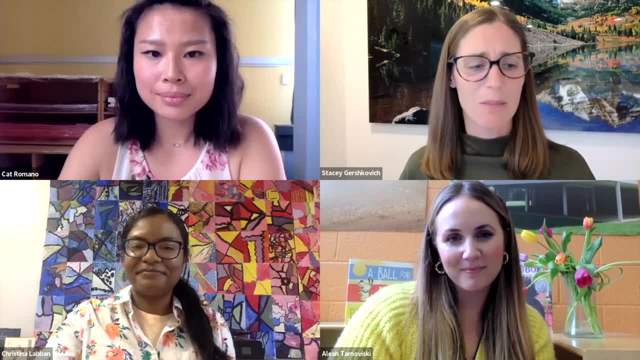 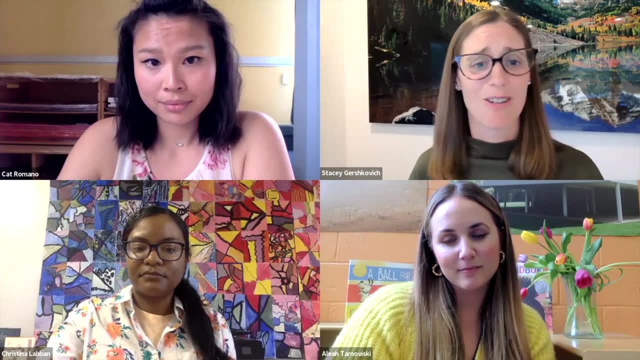 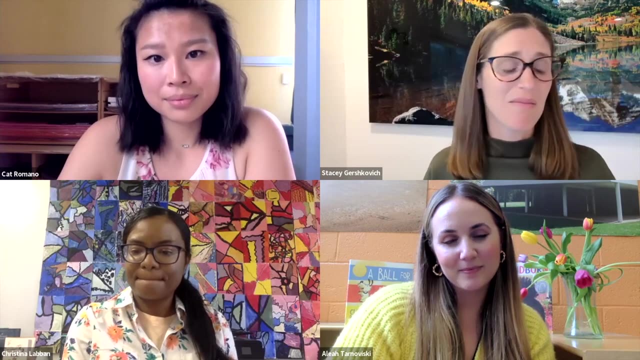 And I just want to say thank you so much for joining us. So, before we get started, we thought it was really important that we could all, as parents, get a little bit of a mind movie of what kindergarten even is like. Maybe some of us haven't been in a kindergarten classroom since we were kindergartners ourselves, or maybe it's been a couple of years, or maybe you just want to remind yourself of what kindergarten is like. 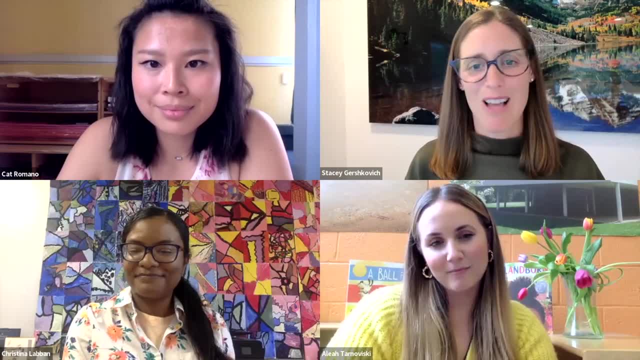 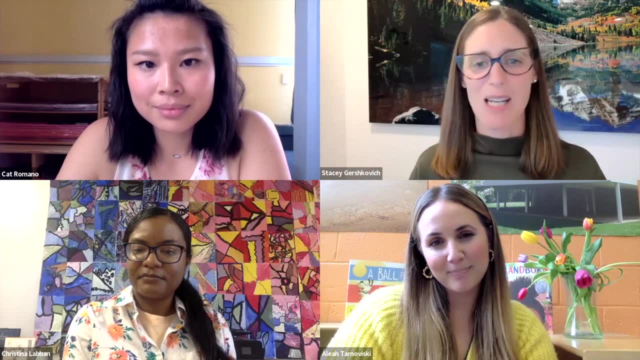 So these ladies- I want to thank them in advance- opened their classroom doors to us via video And in just a moment we're going to play that video And get a chance to make that mind movie of what it is like to be in kindergarten. 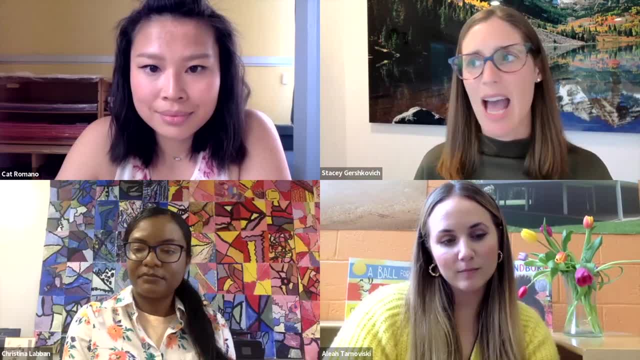 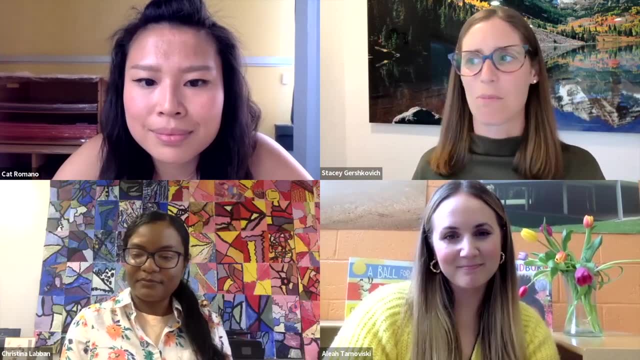 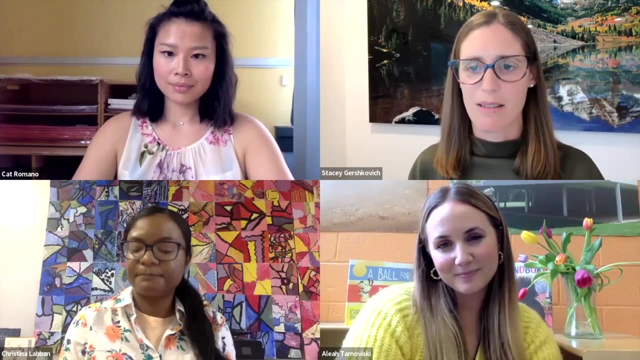 And while we do that, feel free to add to the chat- And I see you guys are in that chat, using it, so keep using it- Anything that excites you about what you see, anything that surprises you about what you see And, again, any questions that pop up, put them in the Q&A and we'll make sure we get those at the end. 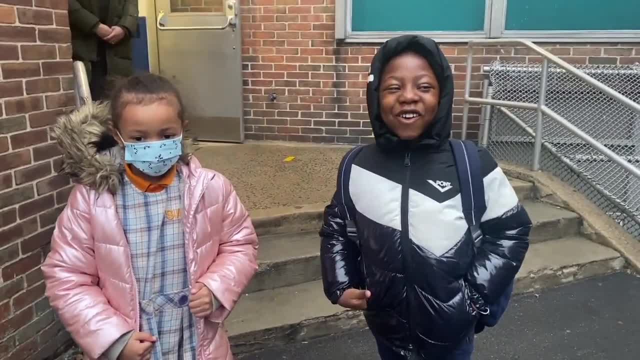 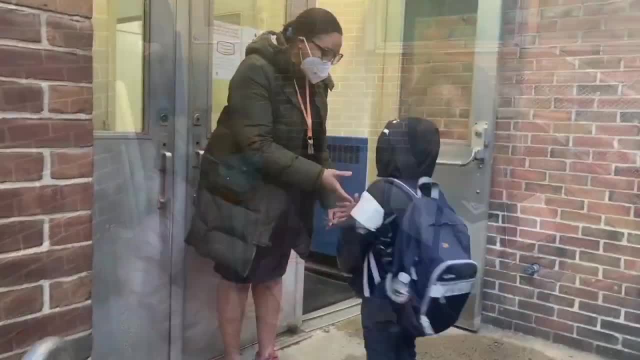 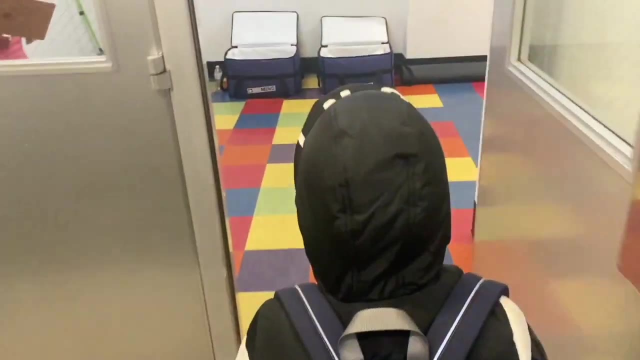 Action: Hey, I'm Apto. Welcome to kindergarten. Hi, I am. I'm going to kindergarten. Good morning, How are you? I'm good, Good, Have a good day. Okay, Where are we going next? What's up? 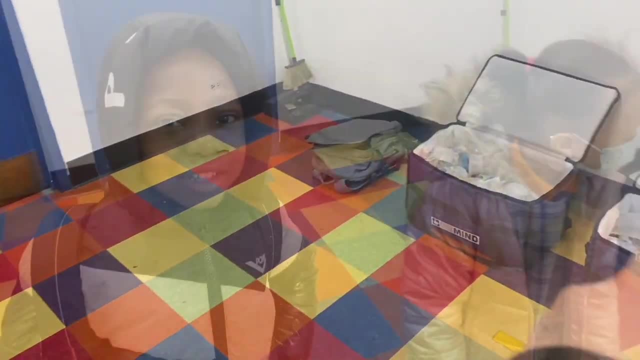 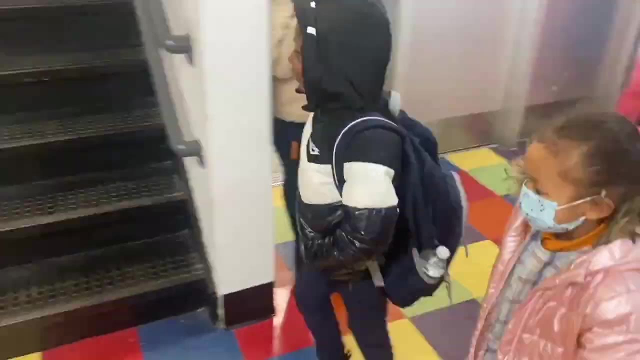 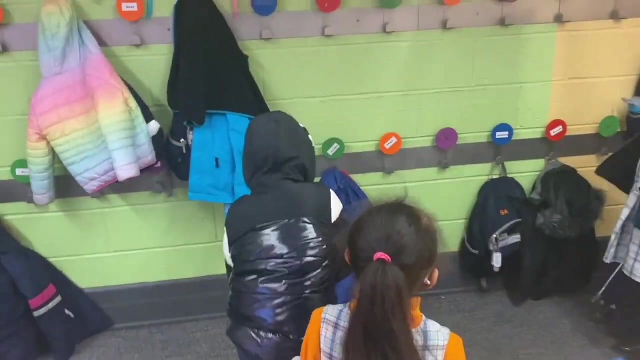 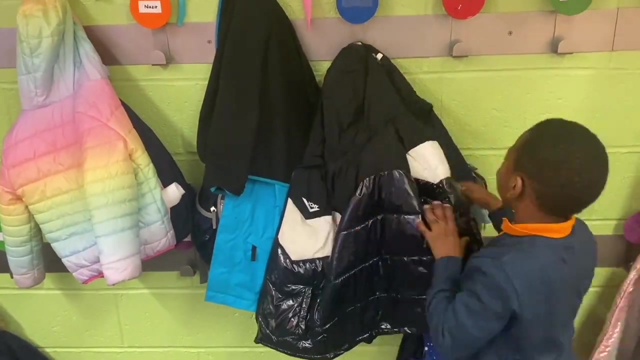 What's here, Abdul? What's here, Abdul? What's that? This is the breakfast we take this morning. Are you going to get breakfast today? No, Okay, This is our class, This is our morning work that we do each day. 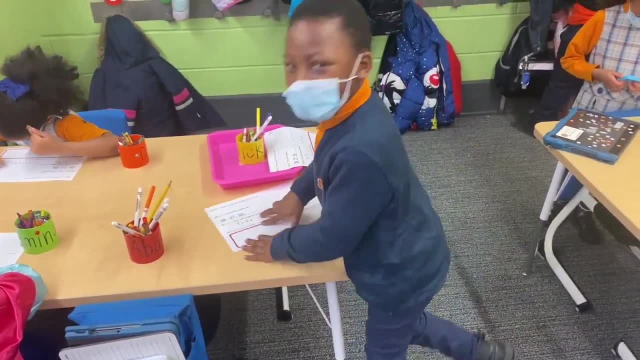 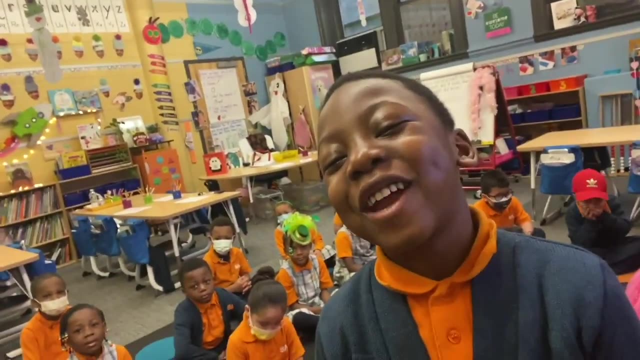 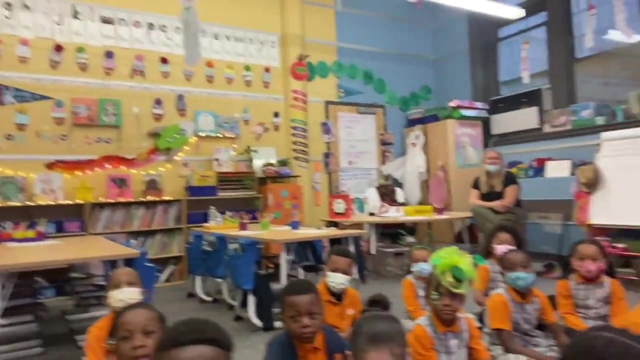 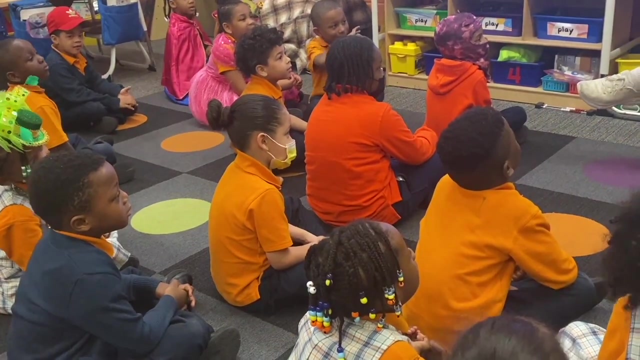 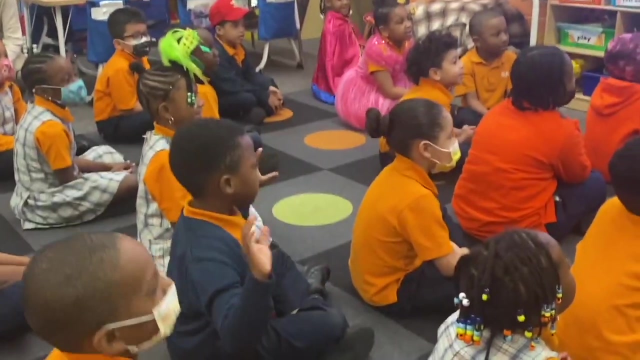 Okay, Good morning kindergarten. Good morning, Good morning. After our morning work we go to a morning meeting. Hi, Everyone say hi, Hi, Okay, Keep the beat today, Here we go. Here we go January, January, March, April, May, June, July and August, September, October, November, December. 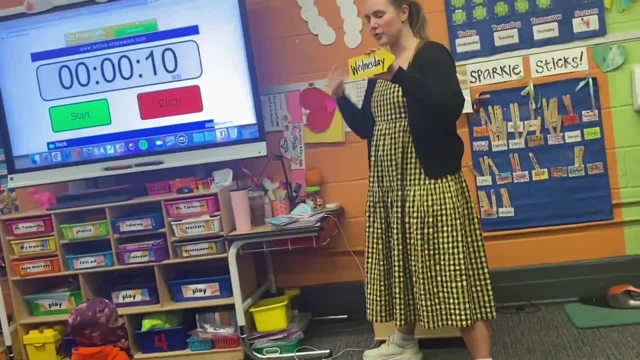 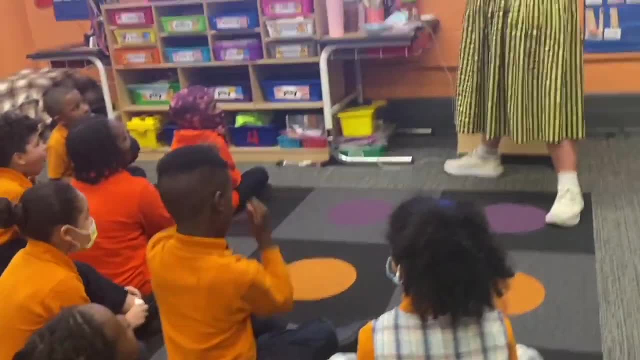 These are the months of the year. Say that in a full sentence: Yesterday, Monday, Wednesday. Let's try that again. Yesterday was Wednesday. Yes, Yesterday was Wednesday. Today is Thursday. Say that as a full sentence: Today is Thursday. 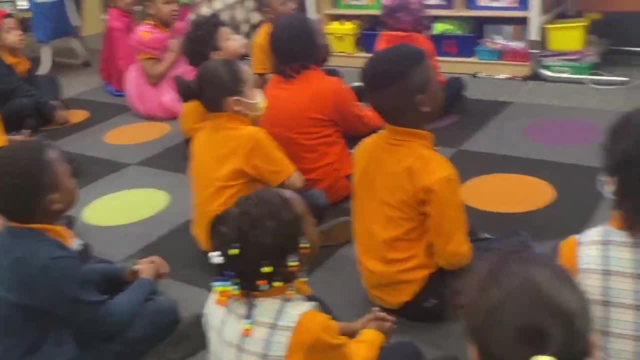 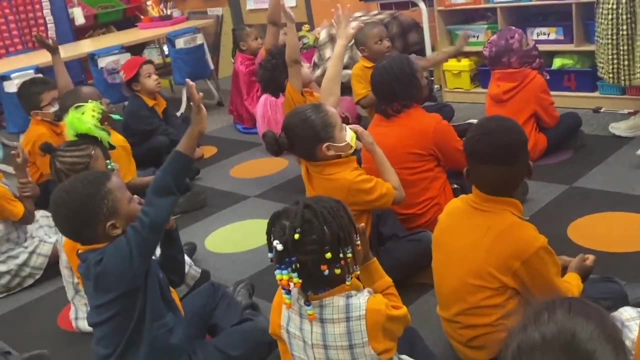 Today is Thursday. Today is Thursday. How do we know that this is Thursday and not Tuesday? Touch your nose if you have an idea. How do you know it's Thursday and not Tuesday, Alexis? Because I see a T and a H. 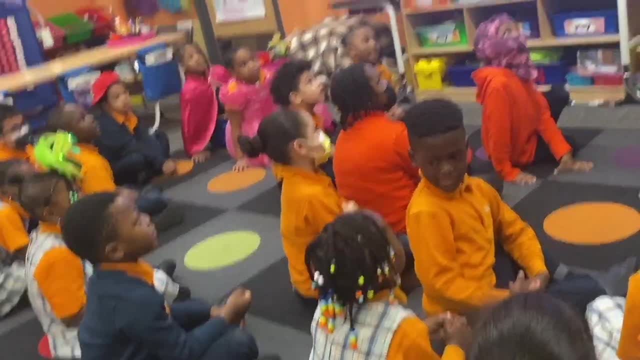 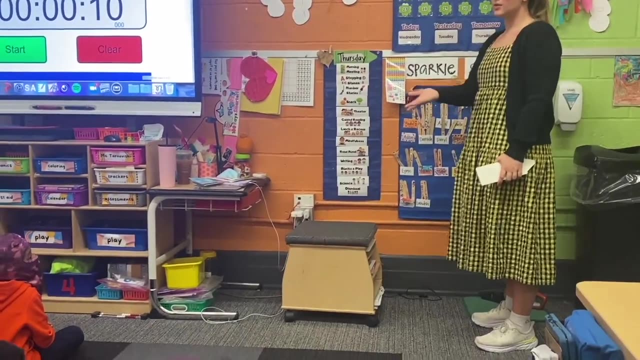 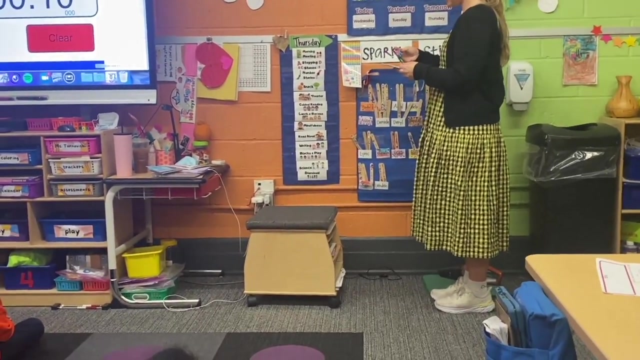 I see a T and a H. What sound does T-H make? Or it makes a V sound sometimes. Today is. Today is Thursday, Thursday March 17th March 17th March 17th 2022.. 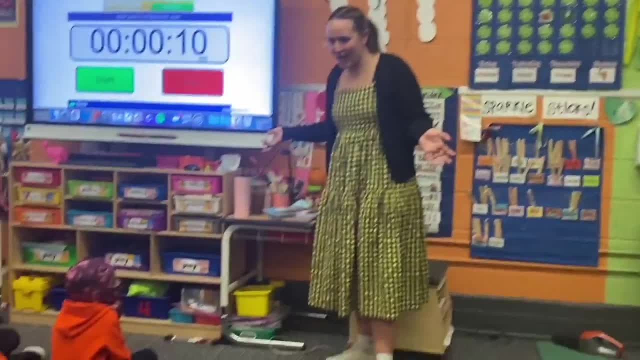 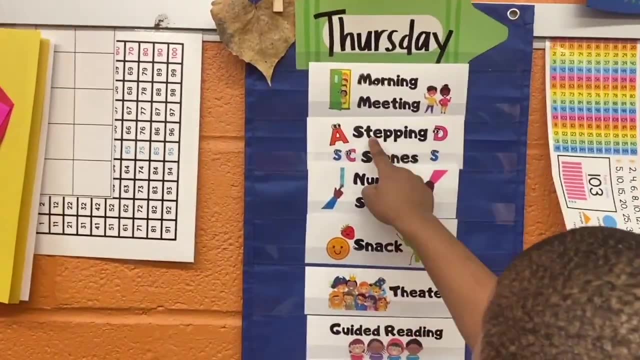 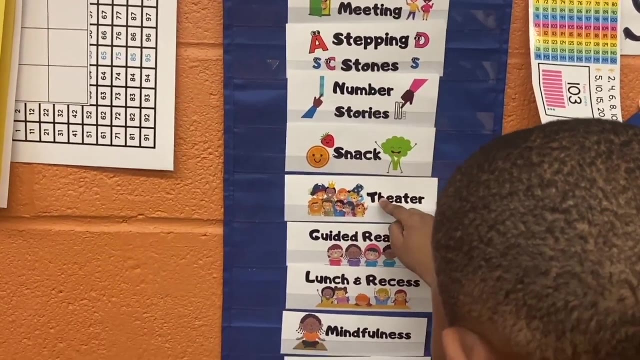 2022.. Everyone say Happy St Patrick's Day. Happy St Patrick's Day. Happy St Patrick's Day. We got. Stepping is down, Stomping stones, Number stories, Snack Theater, Guided reading. 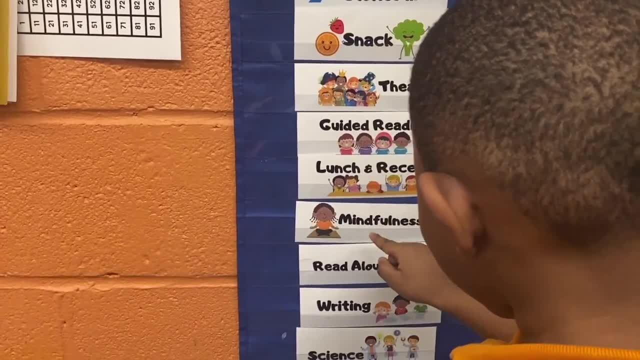 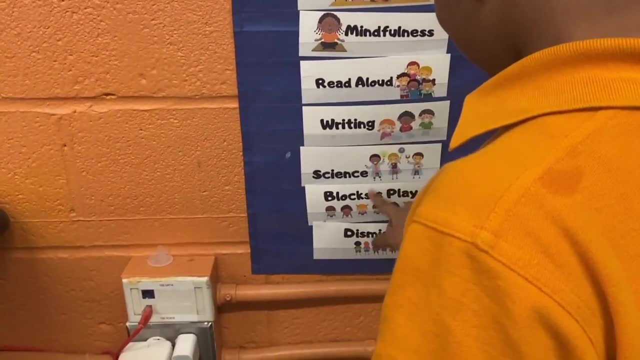 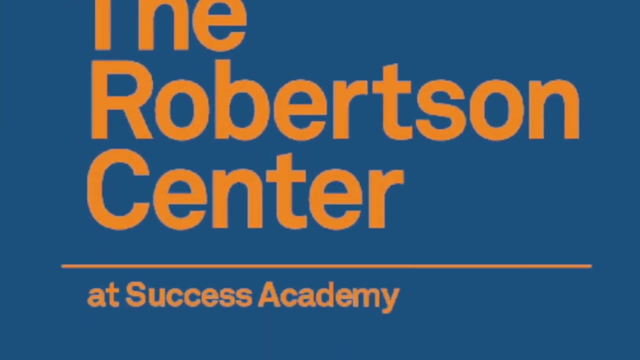 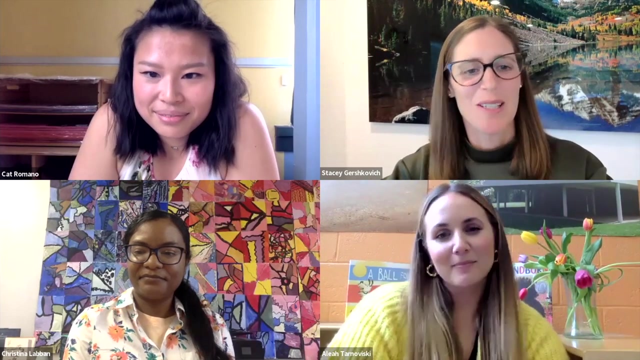 Guided reading: Mindfulness, Mindfulness. Read aloud Writing Science Vlogs and play Dismissal, Dismissal, Okay, Well, thank you, Aliyah. I hope you enjoyed the video. I think it was a little bit of a mind movie. 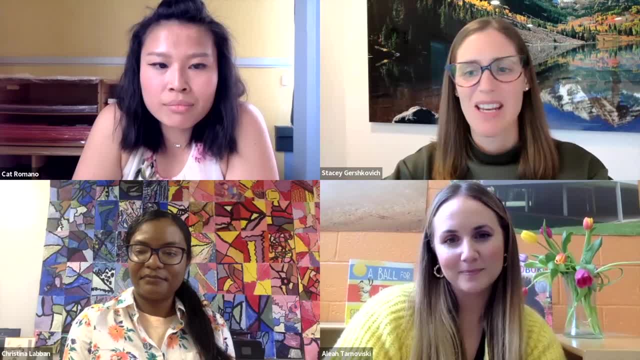 I think it was a little bit of a vision of what it is that it feels like to be in kindergarten. I will preface this by saying that video was taken a couple weeks ago, So that is not the first day of kindergarten. Those kids have worked really hard to get to the place that they are today. 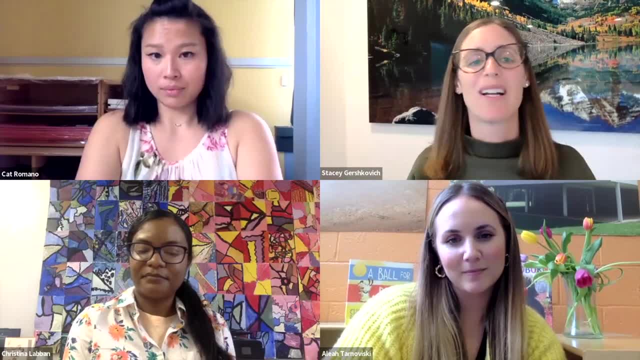 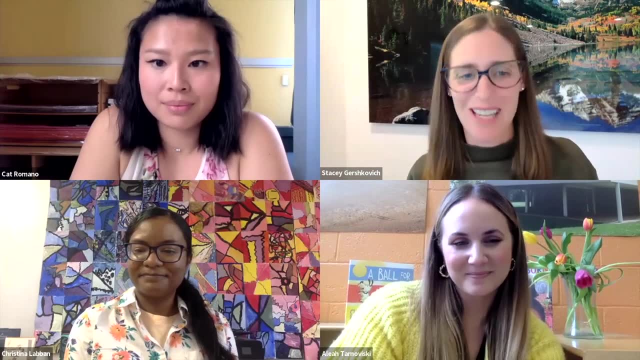 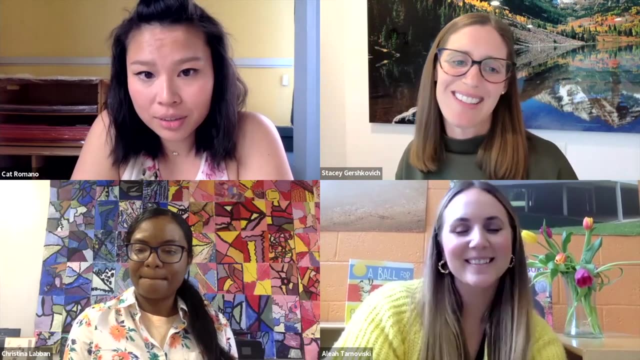 The T-H sounds and all of those fun things. So we're going to get started. So thank you so much for tuning in And we'll see you again in the next video. Bye, bye, Bye, bye, Bye, Bye, Bye. 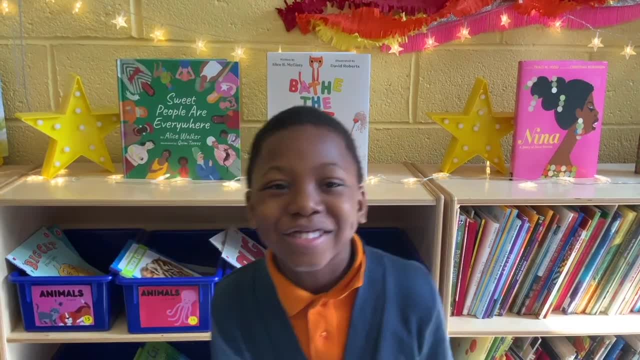 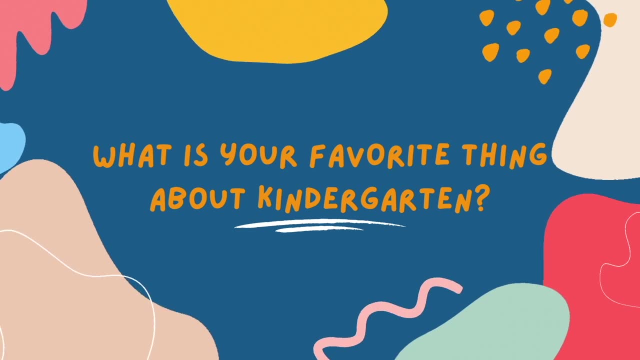 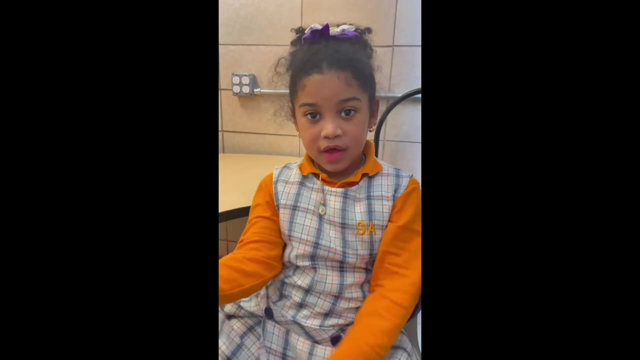 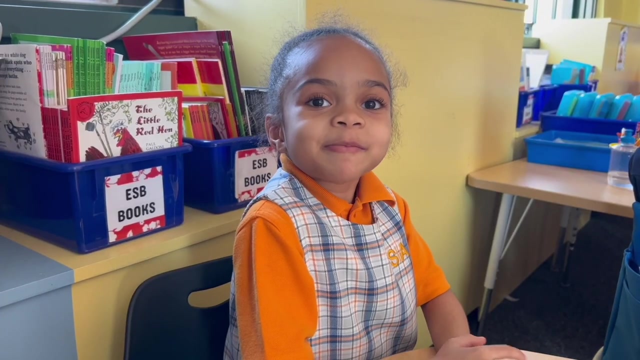 Action, Say action. I don't know what I said, Action. Well, my favorite part is when we learn the whole alphabet From A to Z Um dancing. My favorite part about kindergarten is eating ice cream when it's cold. 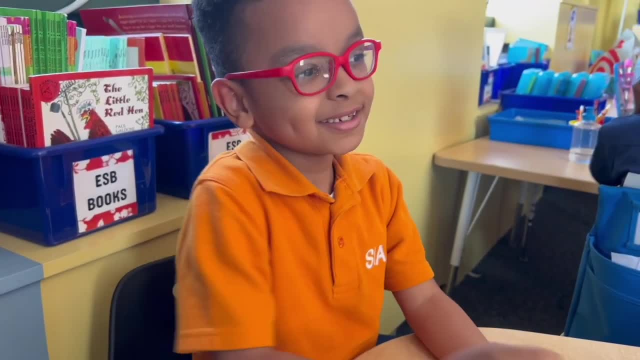 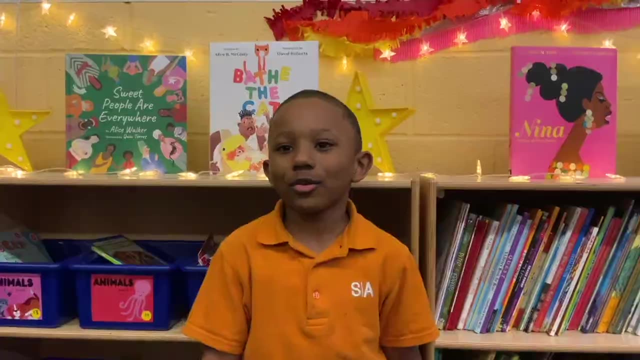 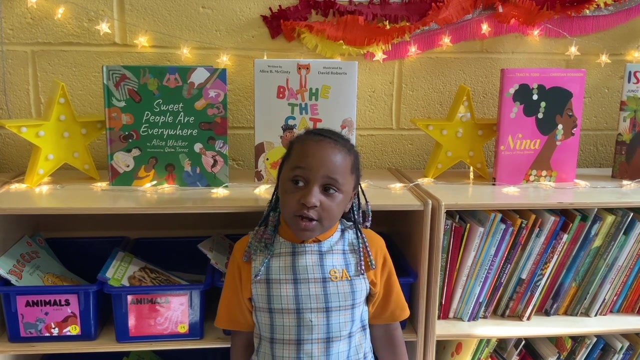 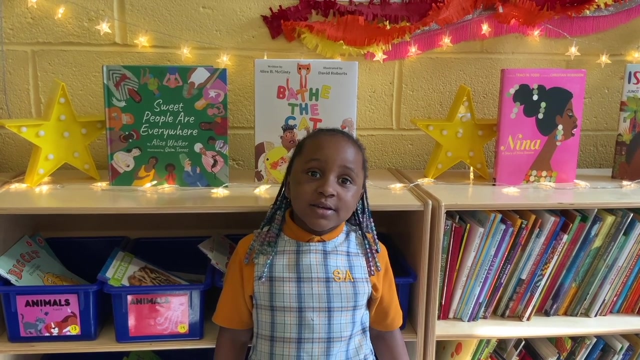 When it's ice cream party, Having lunch, and then it's lab time, Playing Science, Dismissal, Math. It's my favorite thing to learn because I learn everything And I know how to come all the way to infinity. You know how to count to infinity. 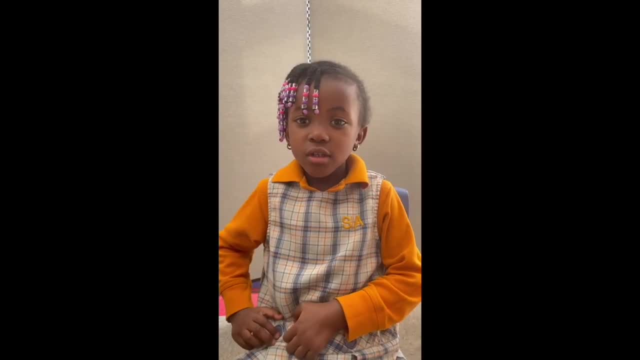 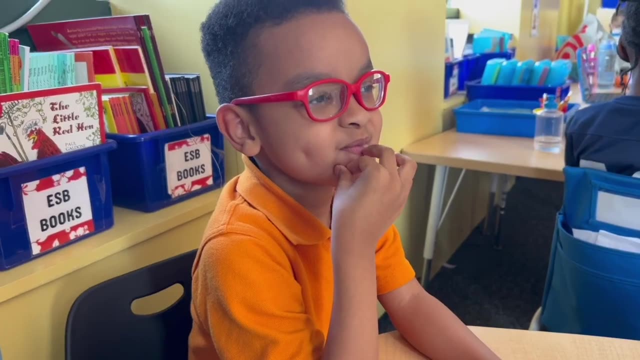 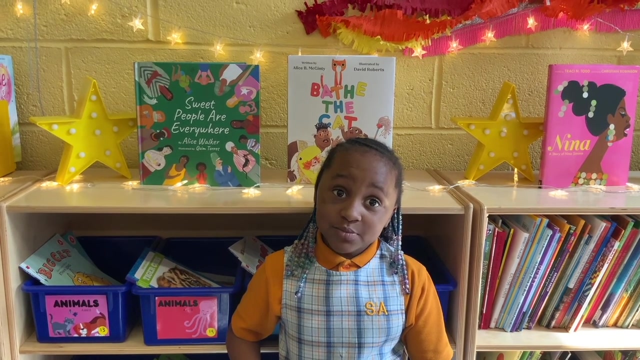 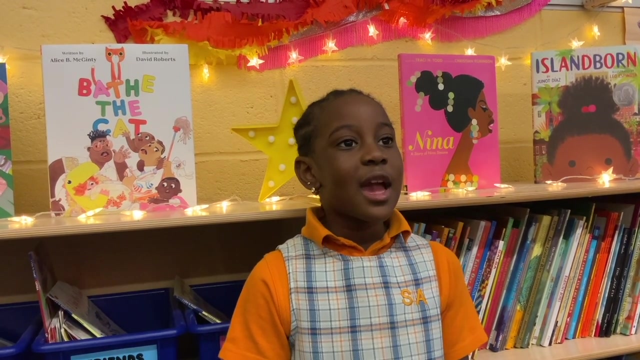 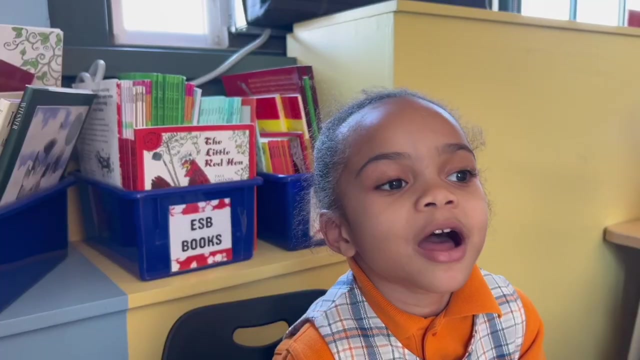 Wow, I learned to count by two. You can practice the name. Oh good, that's a good one I got you. They need to do the homework Every day And knows letters And numbers. I want a parent to know. 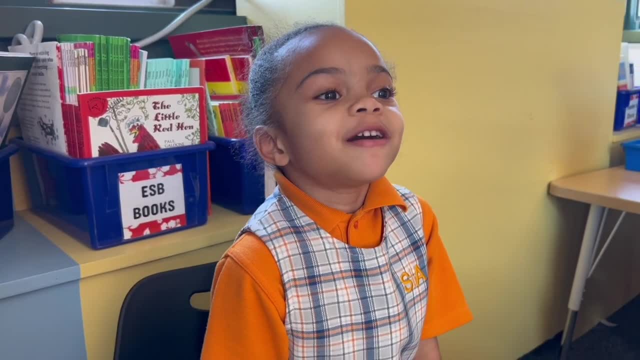 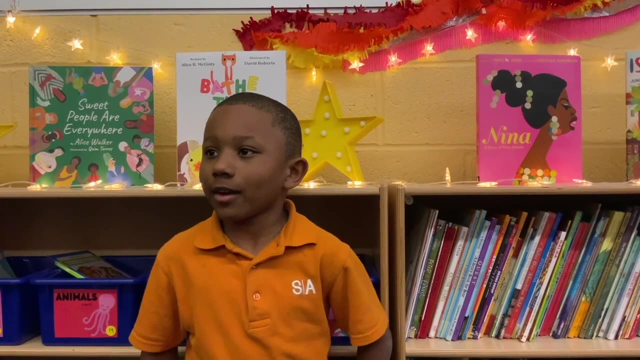 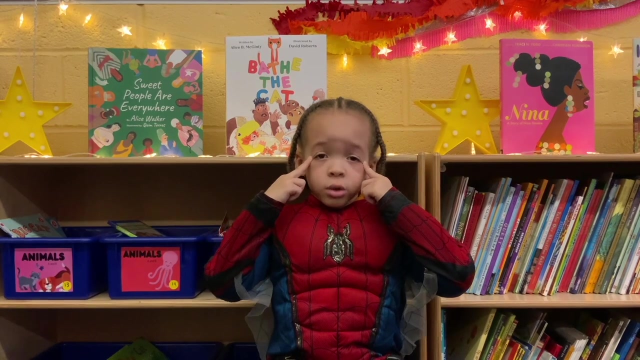 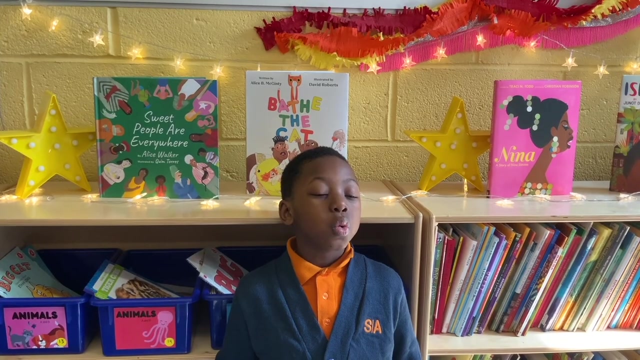 that you can pick some flowers in the grass, like these, like in your backyard. Be kind to your friends Zion Or Spiderman, sorry. So when your brain listens, that means you listen to your parents and your teachers. Read So you can get things. 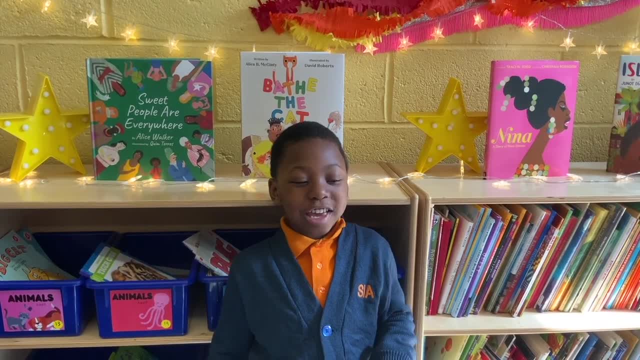 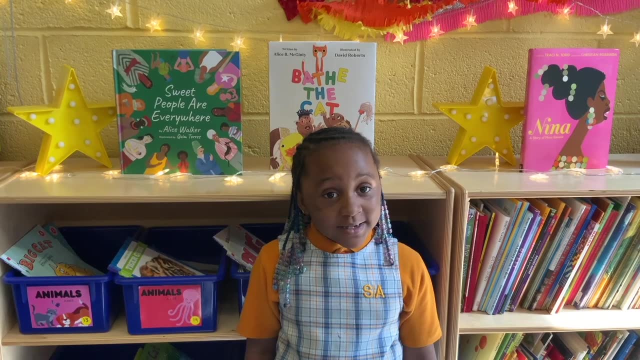 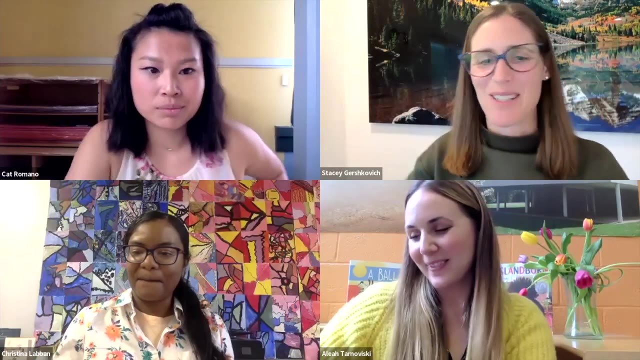 in your mind: There's no talking when the teacher is talking. Bye, Okay, bye Okay. I could watch them all day. We have some other clips that we have to get to, but we wanted to make sure we saw a little bit. 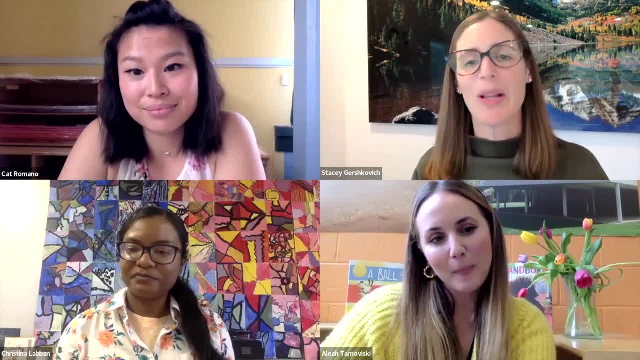 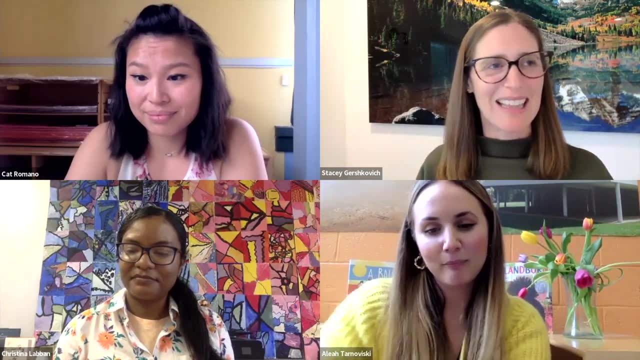 and I don't know about you guys, but when I was watching I could totally see my four year old- her name is Riley- in that video. She was saying some of these things And I think if you said that six months ago I would say, oh, no way. 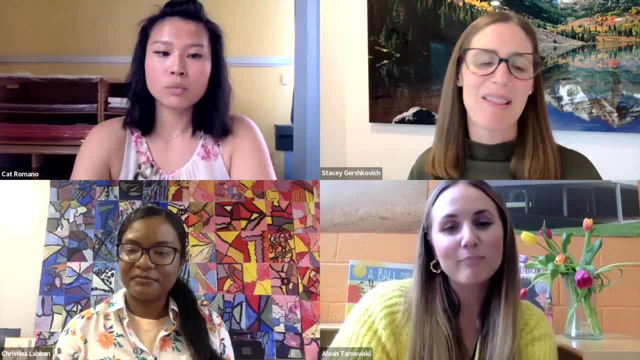 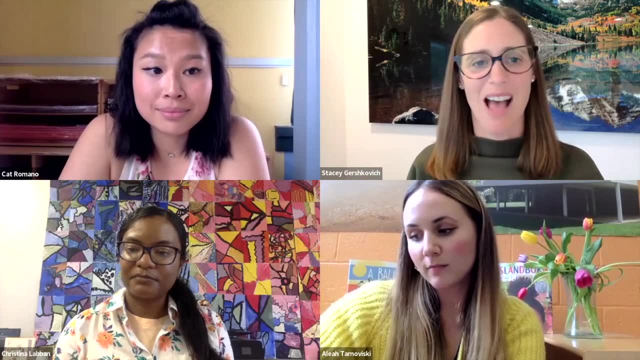 But she's getting to the point where I think in the last month they really have matured and this is why kindergarten does start at this age. So again, we're going to go and do some panel questions. We want to hear directly from the kindergarten teachers who know it best. 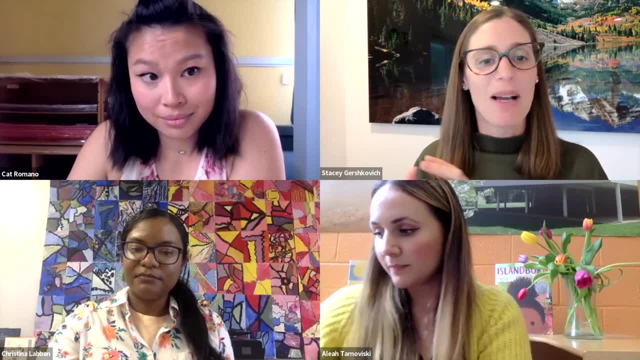 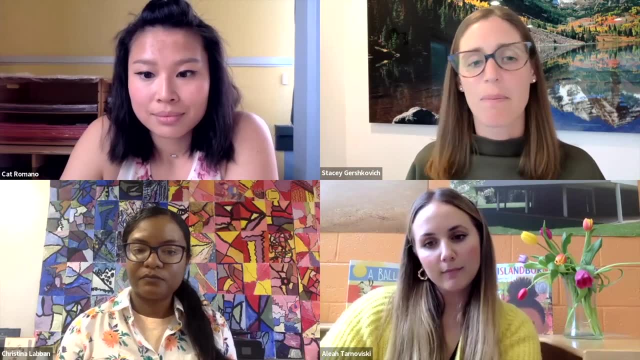 But why don't we get started Again? if there's questions that we don't get to, that you're curious about, that are coming in already in the chat and the Q&A. please go ahead and keep those coming. We'll get to as many as we can. 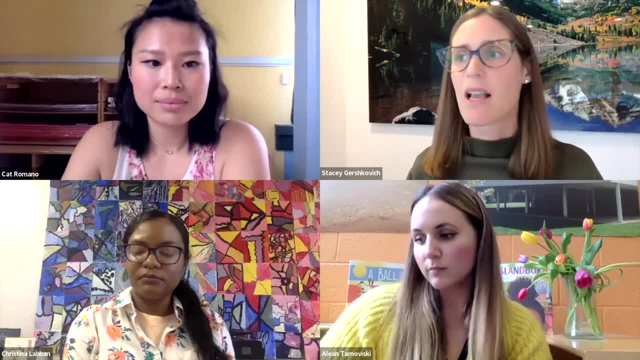 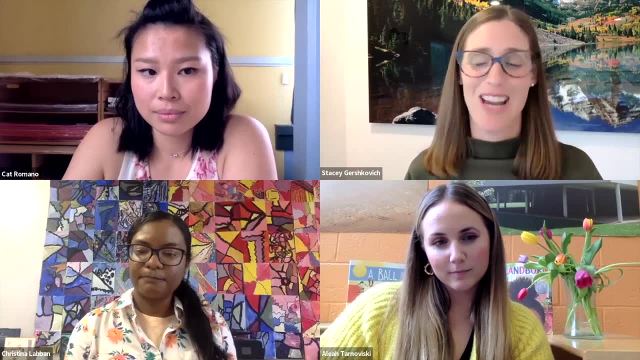 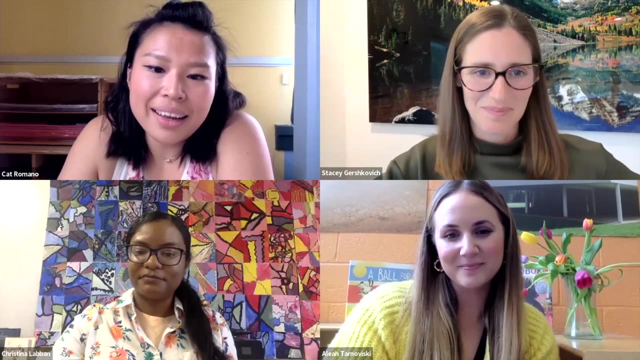 But let's get started with some questions that I know I've seen parents asking. I've had conversations with parents in the past. Ladies from your lens, what is the most exciting or challenging thing about being a kindergartner? I think in the beginning of the year. 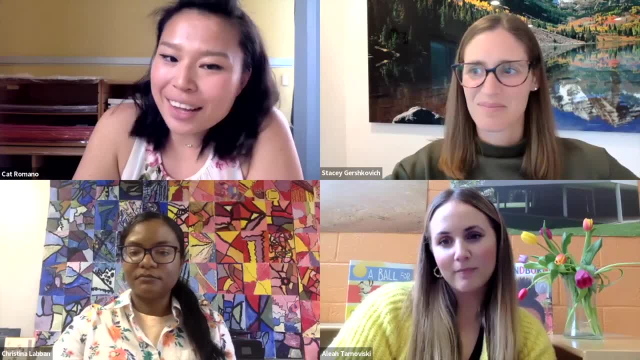 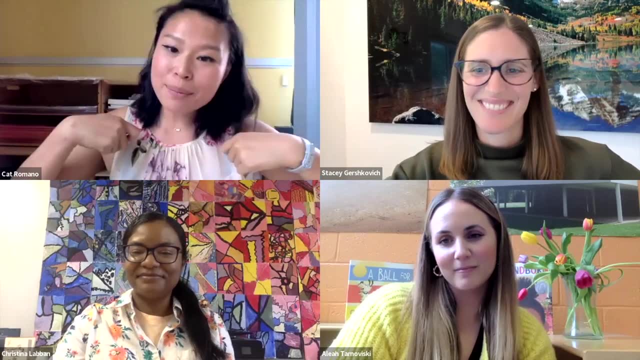 when everyone is coming to school, some really challenging things is just being able to walk Tripping over their shoelaces, or their shoe is coming off, Holding up their backpack, Holding their lunchbox- if they're coming with a lunchbox- And just understanding. 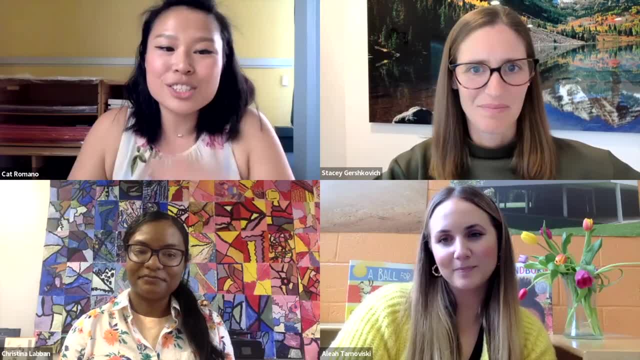 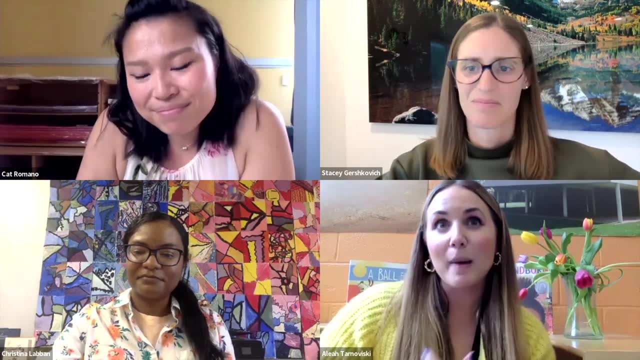 I unzip it in the morning. I've got to take my stuff out And just learning a little bit how to be independent when they come into school. I think independence is probably the most exciting thing to watch as a kindergarten teacher, but it's also the most challenging thing. 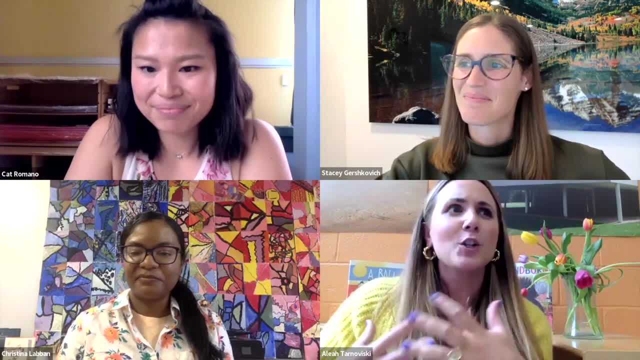 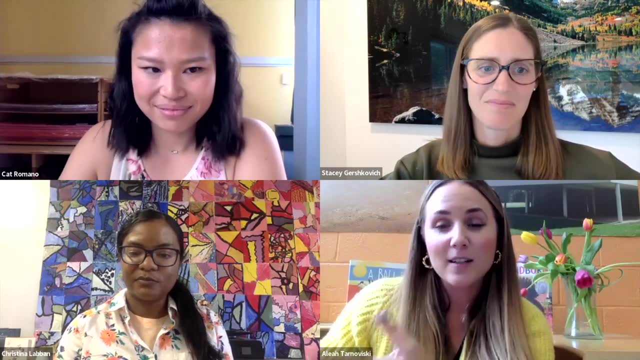 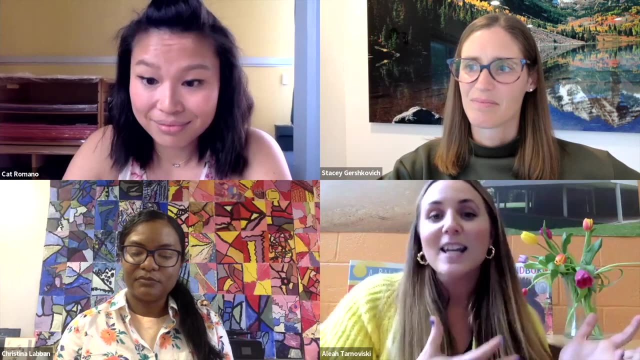 to build And I'm sure, as parents, they really have never. if they didn't go to preschool or their preschool experience was different, they might not have really had that independent experience. And while it's so important for kids to come in, just a little bit aware of themselves, 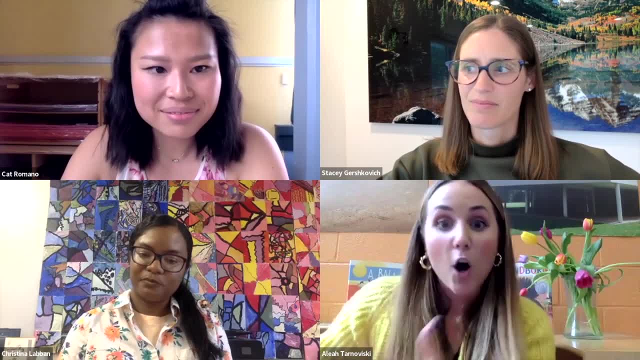 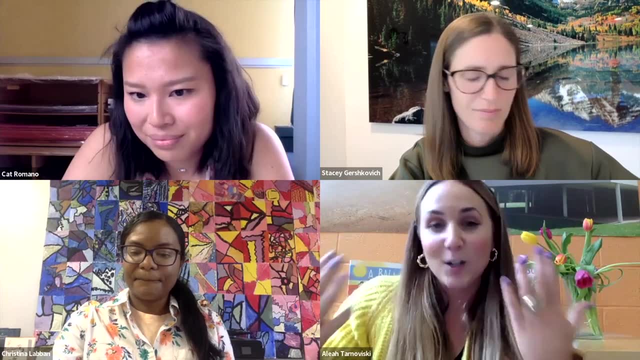 that independence is built in those beginning months when they're really on their own, when they have to carry their backpack in by themselves, when they have to grab their breakfast on their own. And we, as kindergarten teachers, spend so much time in the beginning of the year. 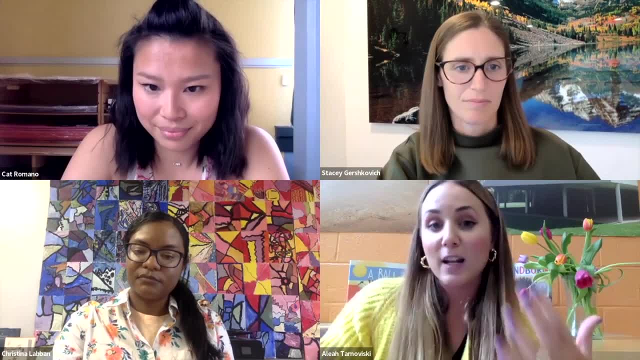 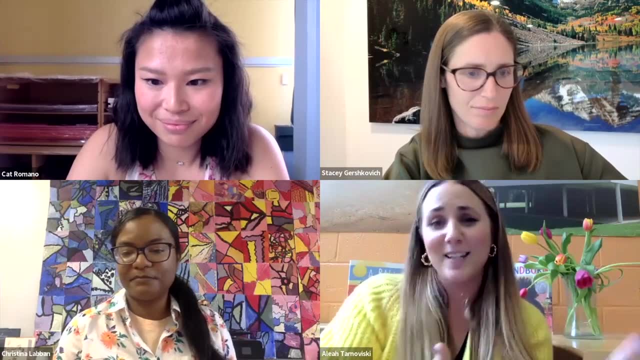 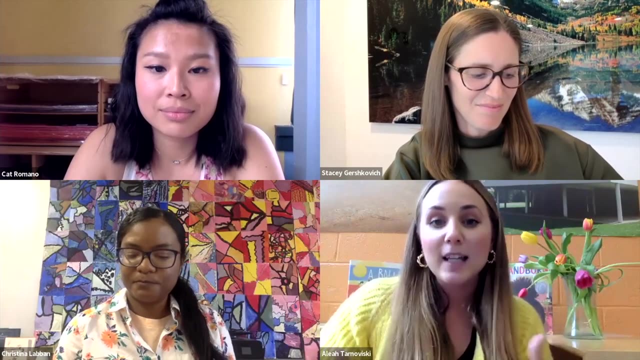 building those habits and building those routines in so that they can feel confident. You saw Abdul unpacking in the morning. That was filmed in March. He's been in school since August and it took us a long time. Thankfully, in kindergarten it's that same routine every day. 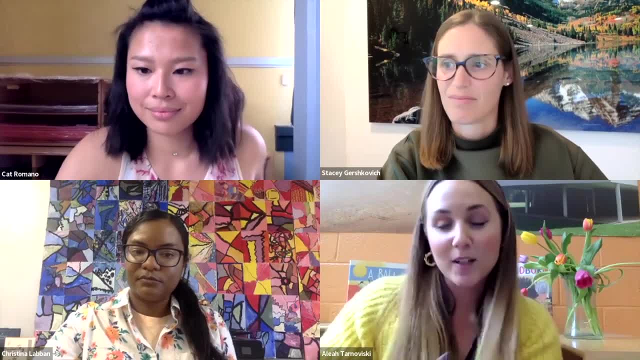 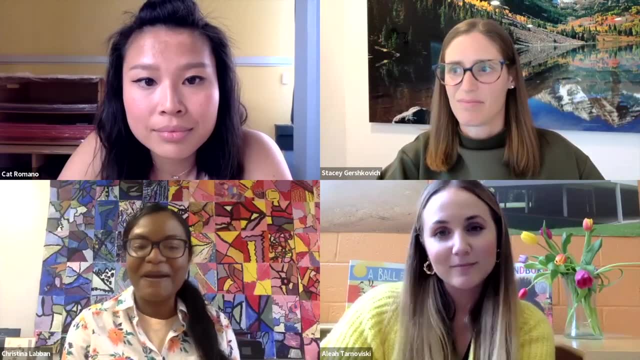 and so it really allows them to build that sense of confidence in their independence, because they know what to expect each day. Yeah, I agree, I think for most of them, gaining independence is the most challenging, but by the end of the year you're amazed with how much they've accomplished. 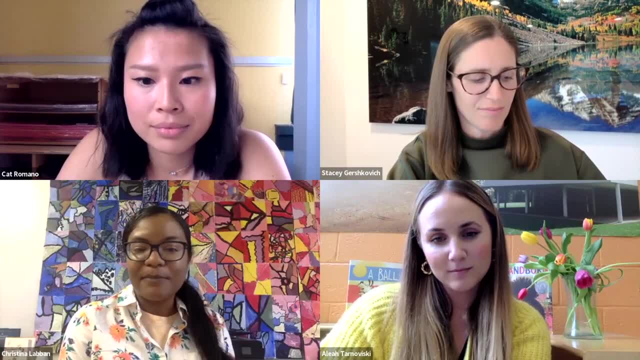 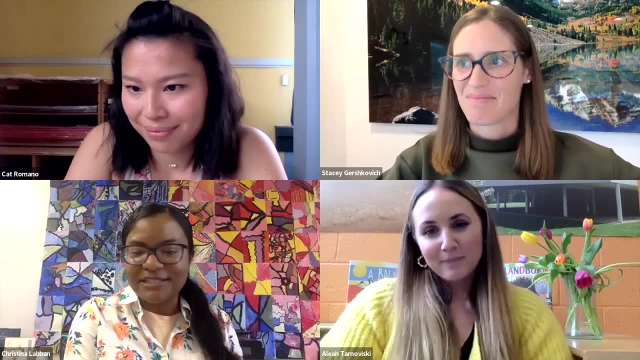 over just a few short months And I think the most exciting thing about kindergarten is them making new friends. They love to come in the morning they're unpacking, they're talking at lunchtime, snack time, anytime they get to chit chat with their friends. 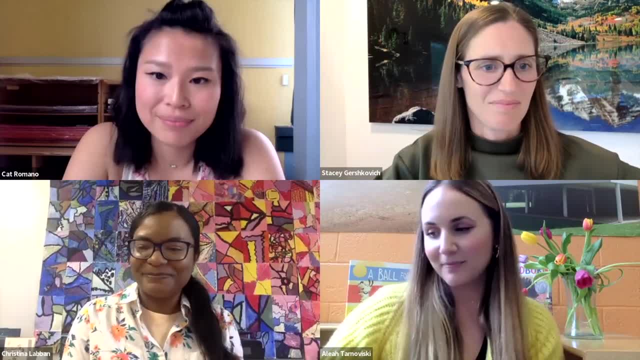 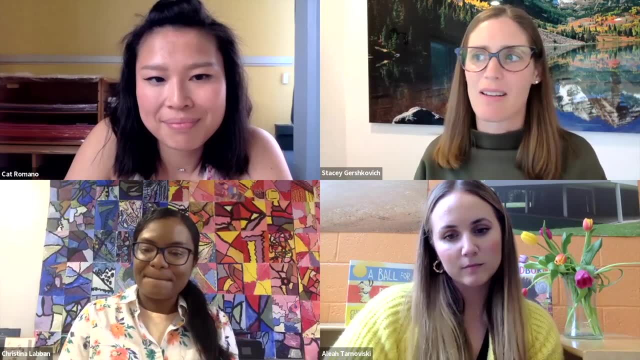 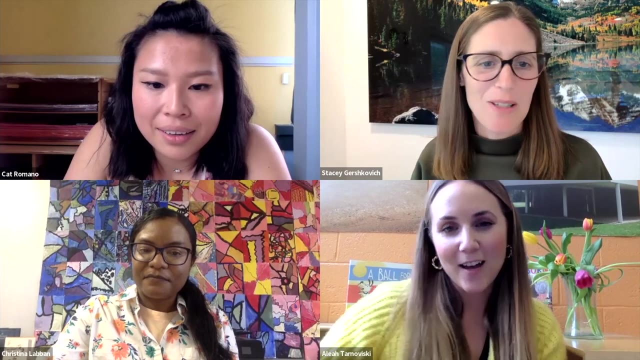 they love it, So they definitely look forward to building those social skills and getting to talk with their friends. Okay, What do kids actually need to be ready to do when they come to kindergarten? Like real talk, What do they really need? I think first and foremost. 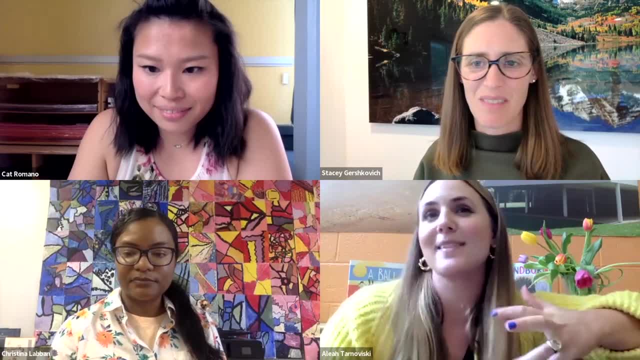 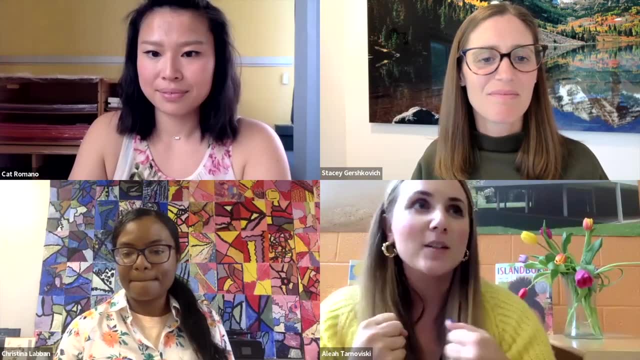 they've got. they have to, like have some sense of who they are. right Like I need them to know their name, I need them to be ready to ask questions, and I think what we always as parents: we want them to be 100% right. 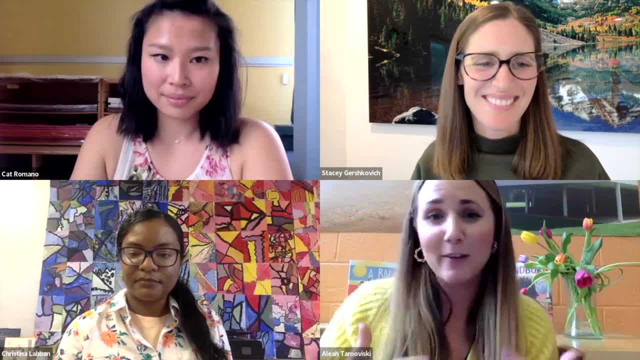 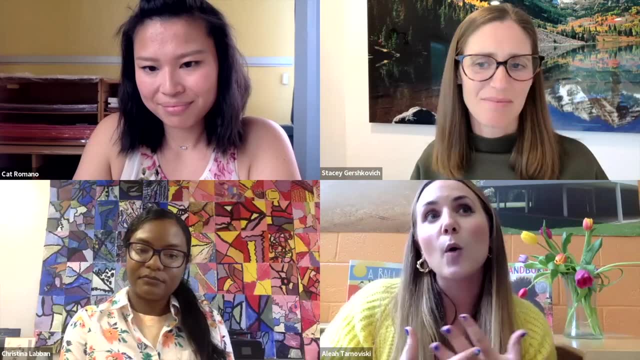 We want them to be 100%. they'll always ask a question when they're confused, they'll always ask for help. they might be at 25% on the first day of school they might be at 10%, but I think, just having some kind of preparation. 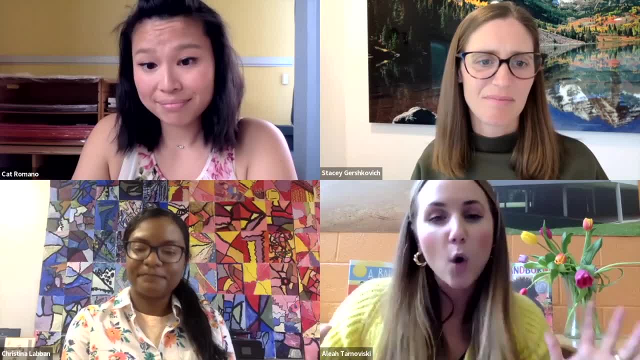 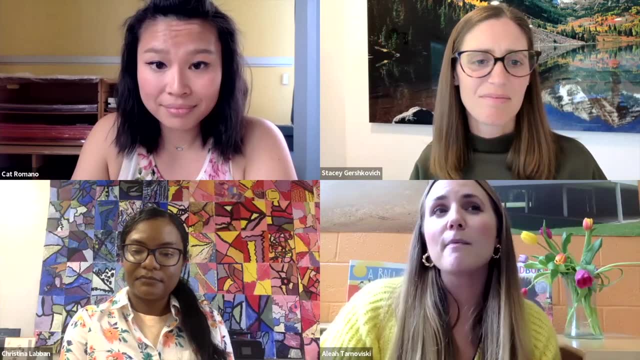 I think what's so amazing as a kindergarten teacher is you see kids come at so many different levels. some kids come in knowing the whole alphabet and all their sounds. some kids just know how to write their first name. some kids just know how to write the first letter in their name. 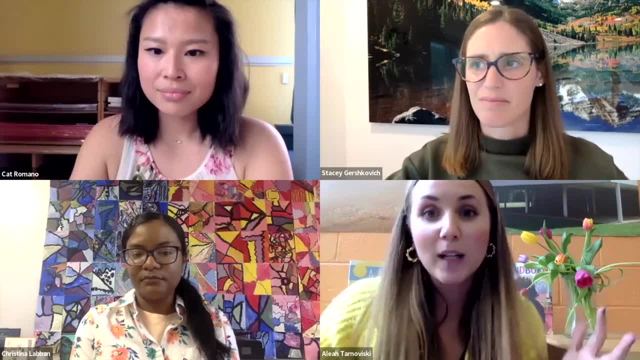 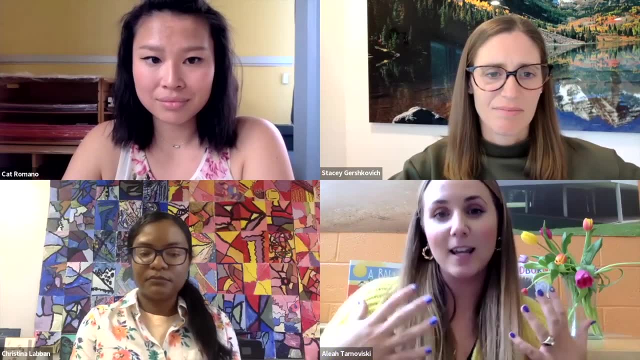 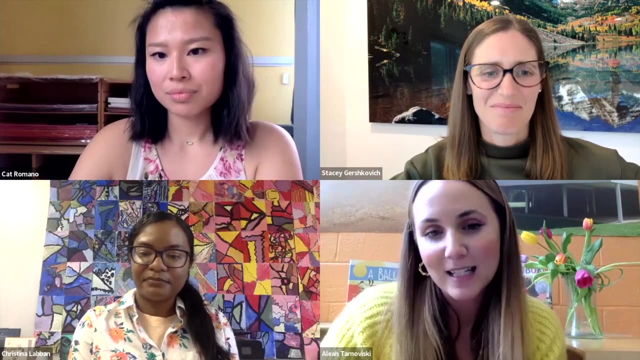 but with that sense of independence to what they're doing in kindergarten, they will grow and they will make the gains. and so I just think a readiness to dive in to learning and excitement, I think, is the number one thing I would say to get your child ready for in those beginning days. 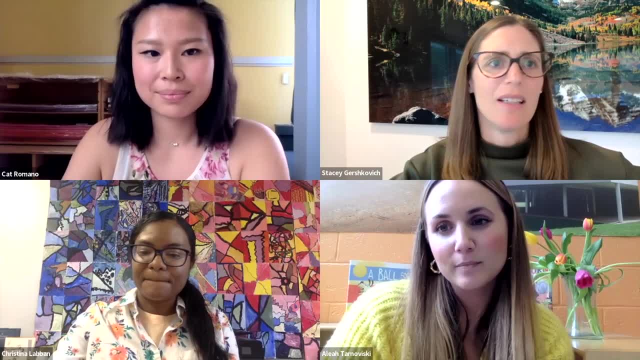 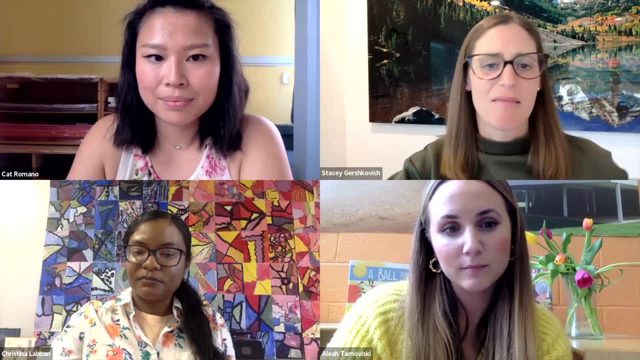 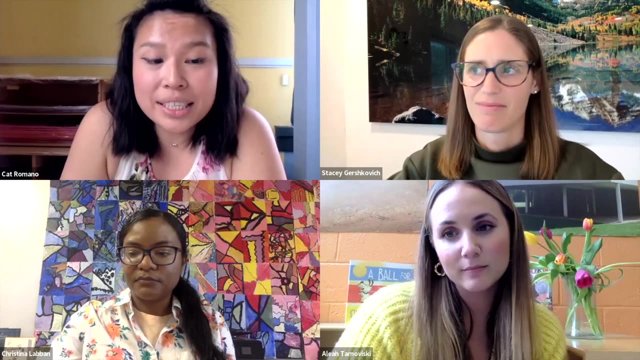 Anything to know, Kat, Christina, anything about maybe unpacking, about their social interactions, anything that maybe Aliyah hasn't touched on yet, I would say, when it comes to coming into the classroom, just knowing which way you're going, where you're going, because many times at the beginning of the school year, 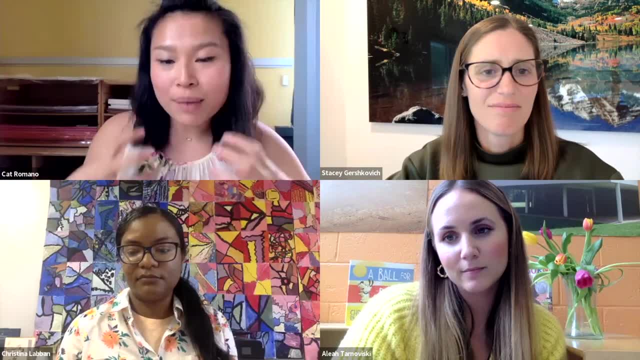 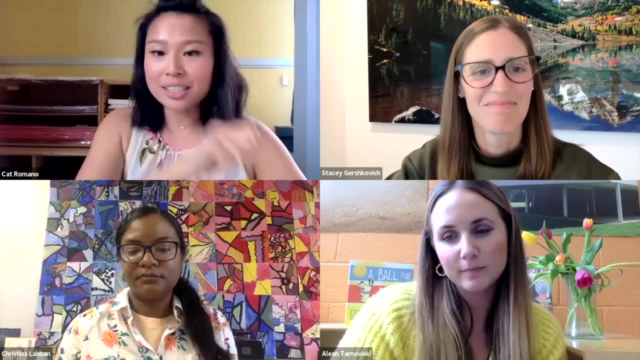 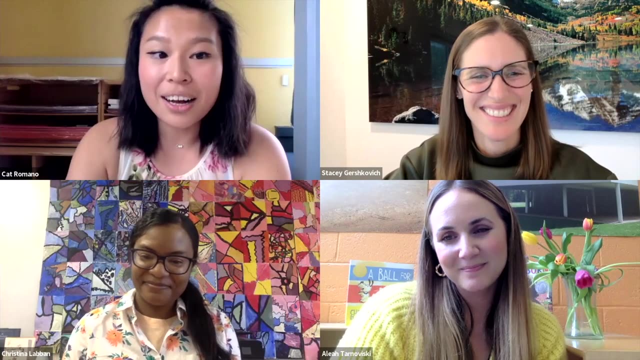 kids who are coming up the stairs will walk past their classroom just remembering who their homeroom teacher is. every day, just saying our names is very helpful: practicing unzipping that bag, because the little latch gets caught in the material and then they say it's stuck forever. 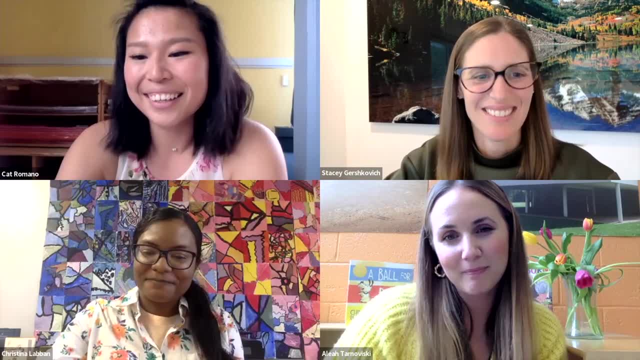 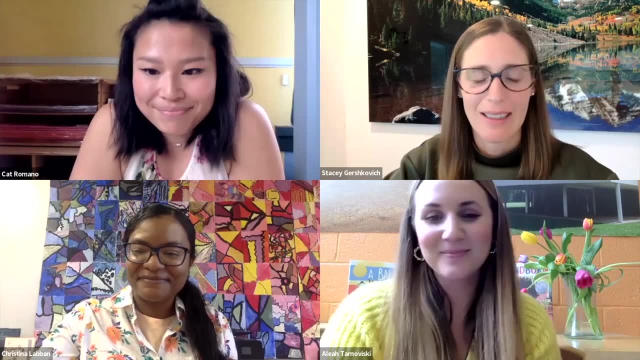 is definitely ways to get ready for kindergarten. Yeah, I guess we're all thrilled we start kindergarten, at least in the fall, so we don't have to deal with jackets and sweaters and scarves right away. but the zipping and unzipping is definitely something we can work on. 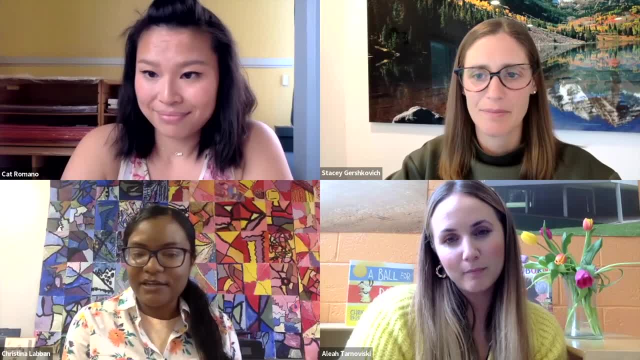 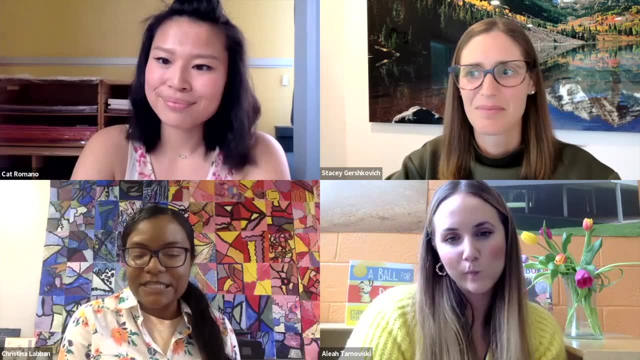 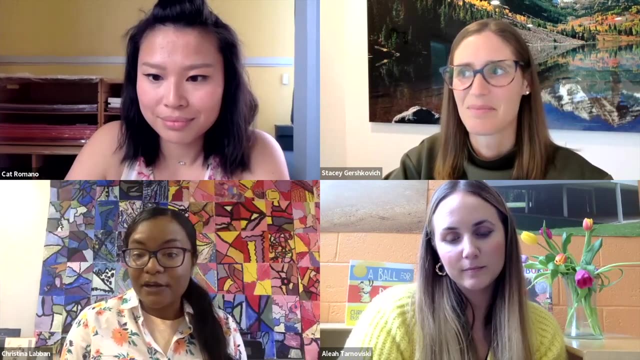 Go ahead, Christina. Yeah, I was just saying for them to just come in just excited and ready to learn, maybe doing a read aloud with them or reading to them a book about your first day of school and how exciting it could be just to prepare them better. 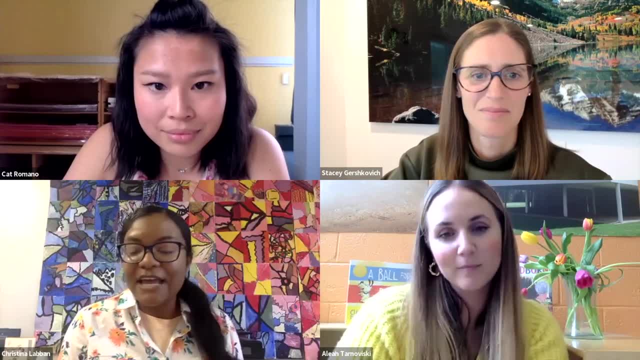 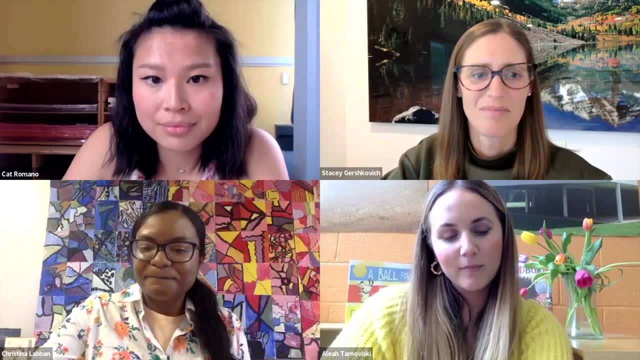 about what to expect, like meeting your new teachers, meeting new friends. there might be some things that you think are scary, but it's really not. I feel like that's really comforting. I also think to build up what they're saying, it's just an awareness of school. 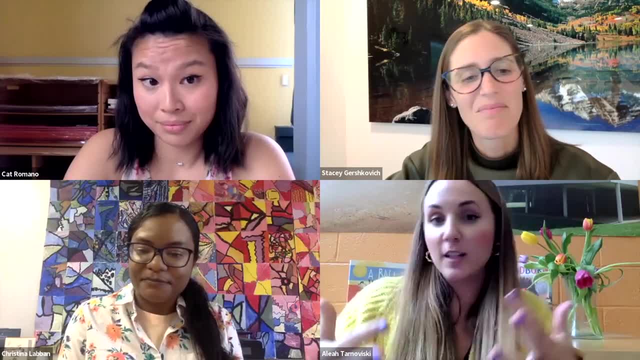 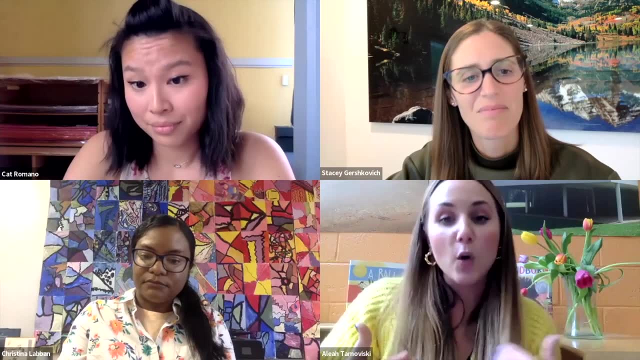 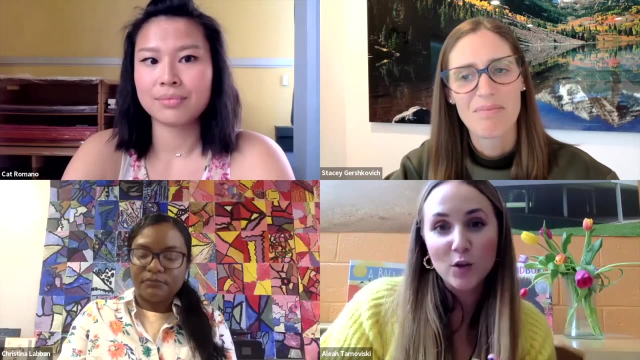 so you're preparing them. this is your teacher, this is your teacher's name. on the first day of school at your schools it might look different. you might meet your teachers outside, or you might meet your teachers before I know. at our schools we do a dress rehearsal. 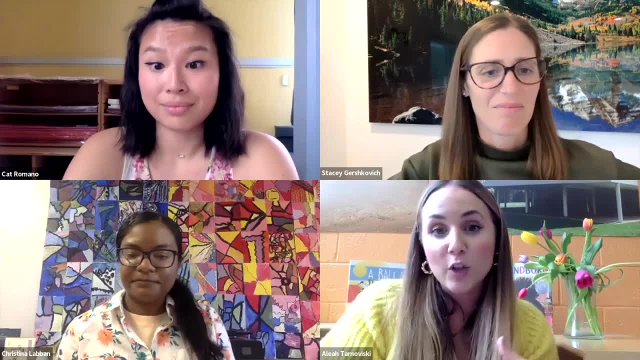 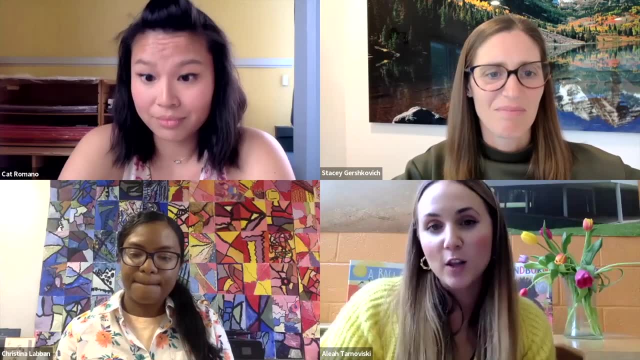 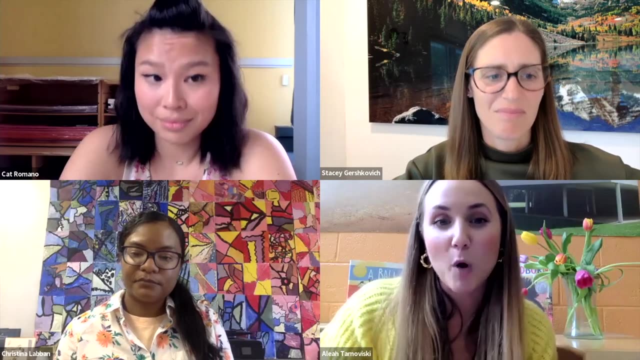 so they are familiar with us. so, preparing them, you're going to walk to that same teacher that you met last week. this is her name, this is the name of your class you're going to talk about. but I think for them to have some foundation, it helps them feel less nervous. 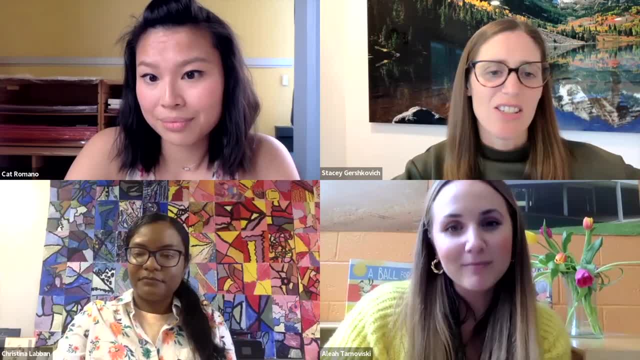 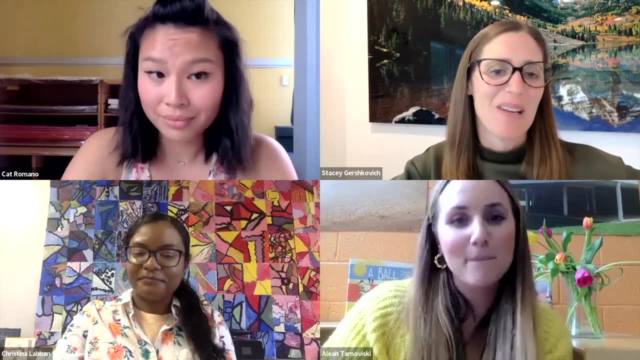 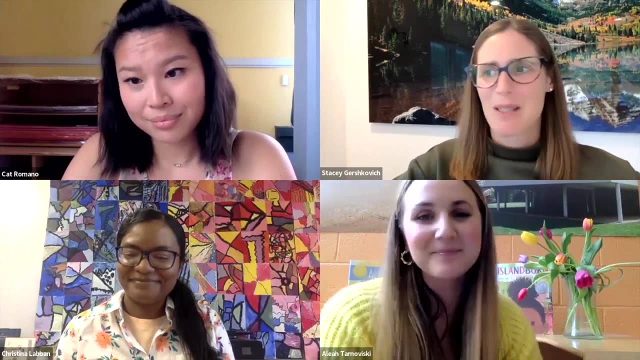 in those moments when it's brand new. I think that's really good advice: just talking to your kids about it: making that teacher's name a household name early on and using that name, the more often it feels really nice when you walk in and you say, oh, that's my teacher. 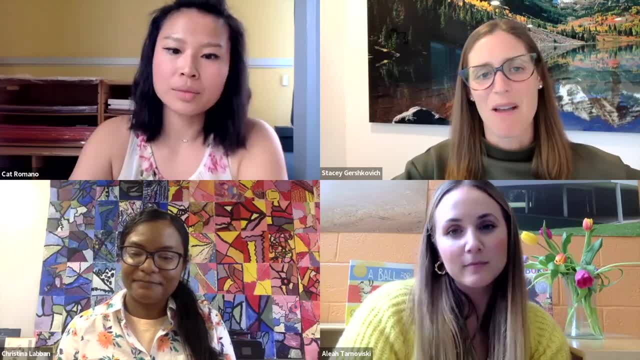 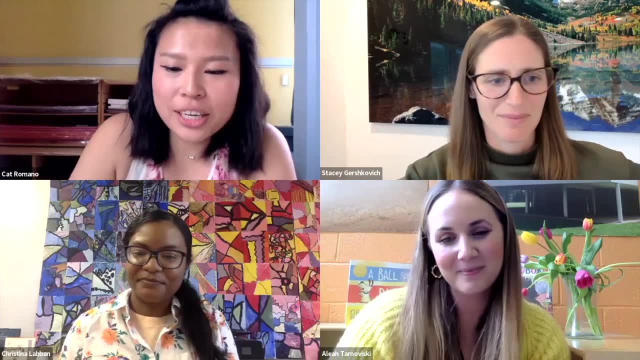 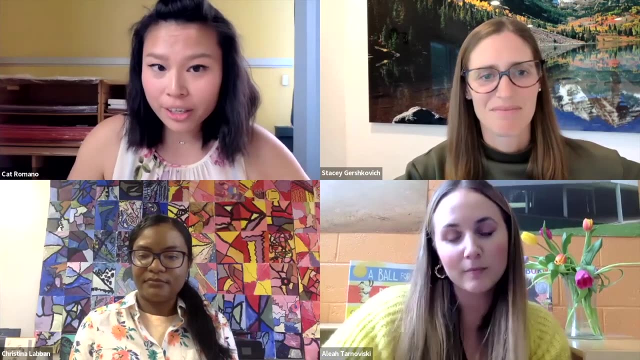 I want to hear from you any misconceptions that you've seen families have about what needs to happen before kids come to kindergarten. I think just looking over from the chat a lot of parents seem like: what do I need to do academically to get my kids ready for kindergarten? 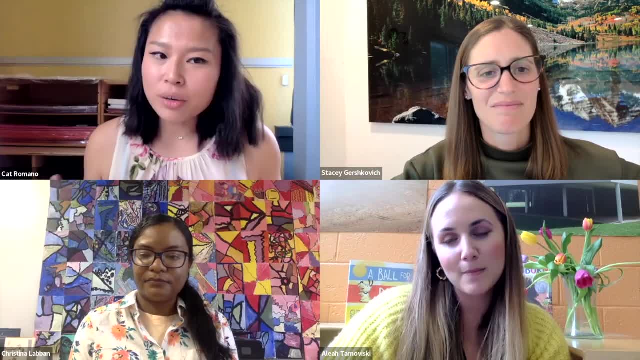 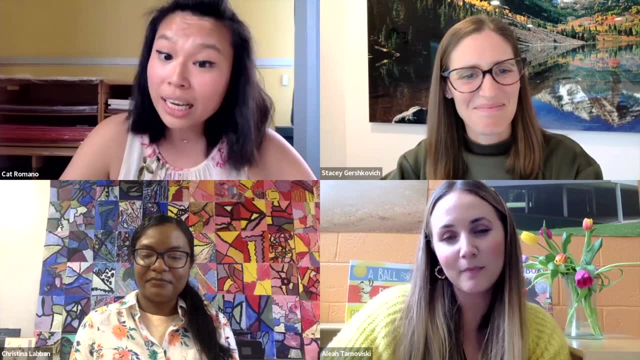 if they had some pre-k, if they didn't have some pre-k. just want to mention everyone is going to be okay on the first day of school. some kids know the alphabet when they come in. some kids can count and some kids cannot, and that's definitely okay. 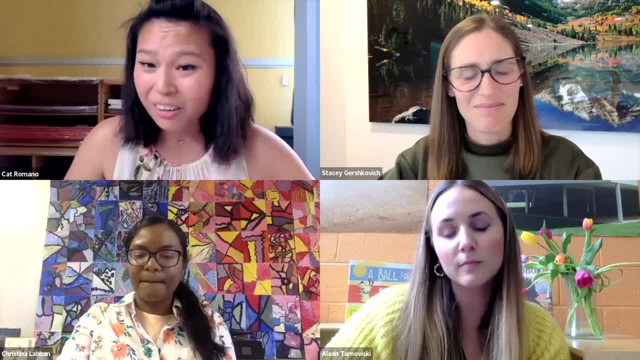 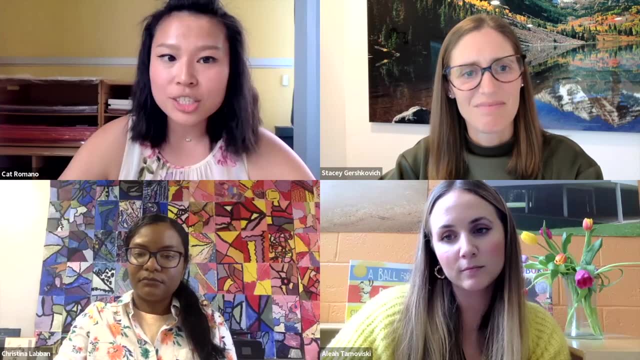 it is totally normal, it is fine. you don't need to feel like you are behind it all on the first day of school, because we are able to get everyone where they need to be by the end of the year, again just being super excited to be in a new space. 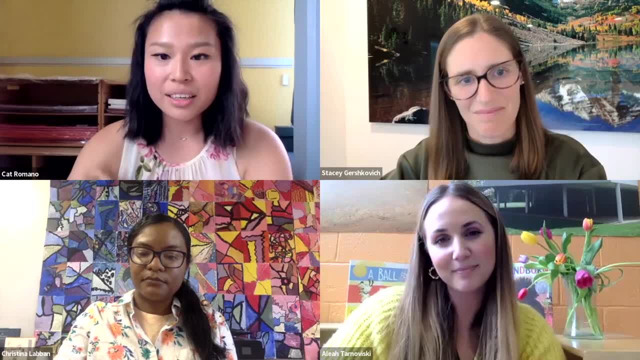 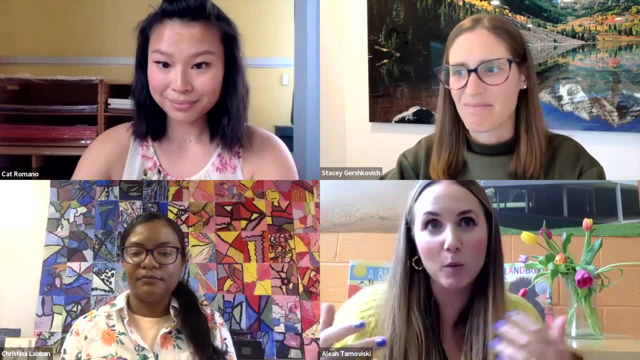 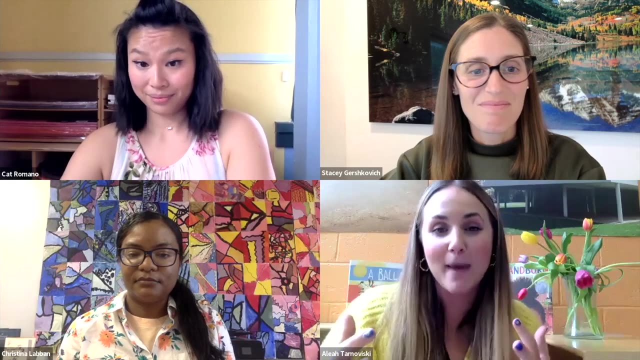 without mom and dad or aunt, uncle, grandpa, just being ready like they are not going to be there could be the best way to prepare your scholar. I also think you can feel confident that your child's needs are also going to be met, and I think that is the magic. 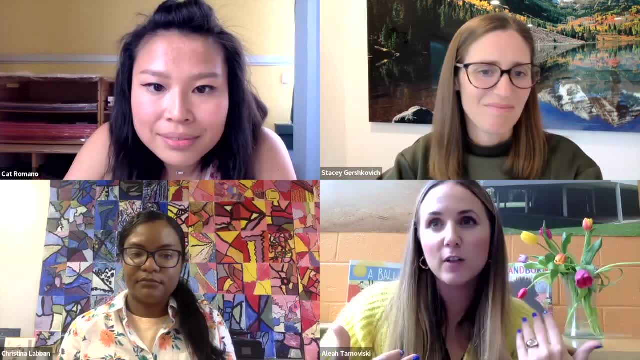 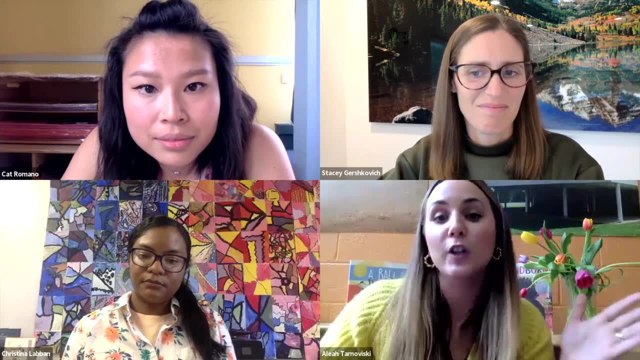 of kindergarten and being a kindergarten teacher, because you get kids at so many different levels and our job is to make sure that every kid feels challenged and everyone feels a part of that learning community. and so, wherever your kid falls on that spectrum, if you feel like they are not ready, 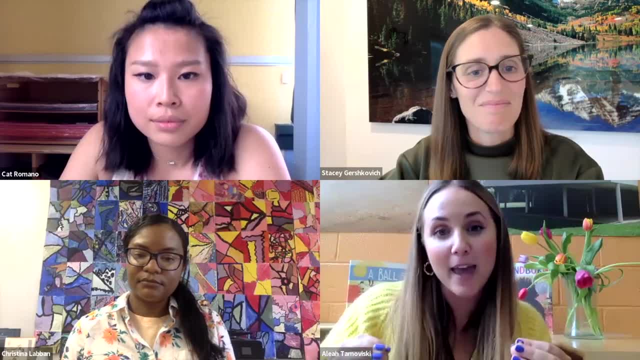 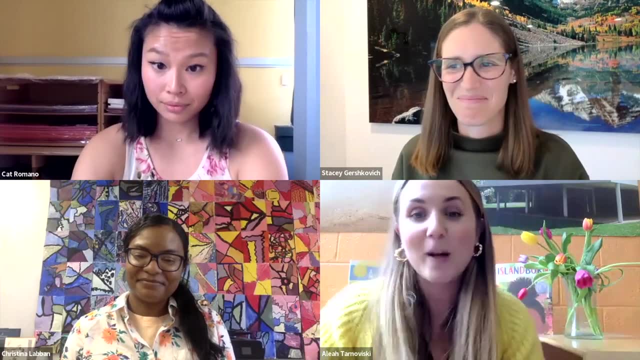 or you are worried or you feel like they are over prepared. they are going to be met where they are at as learners, and so I also want to say that you might be sitting there thinking they do know so much, and that is amazing, and I think what is so cool is in those beginning days. 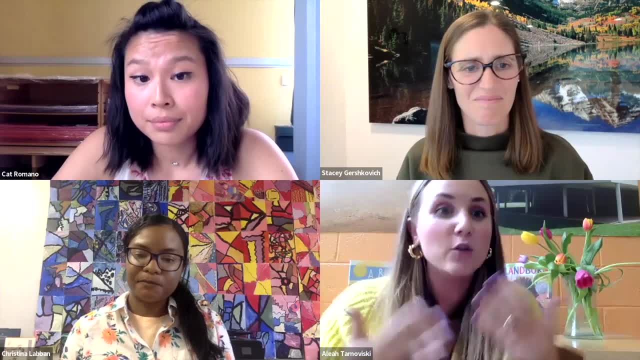 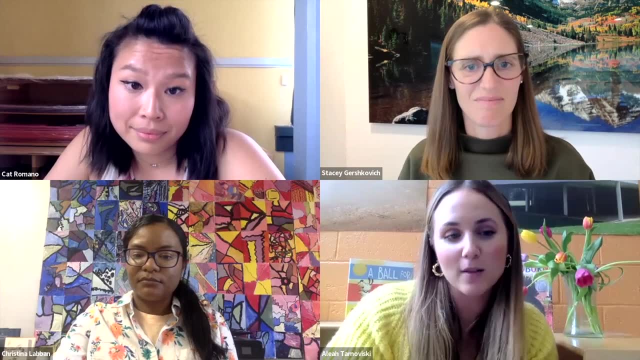 those kids get to be leaders in our classroom and kind of walk some of their friends who may need more support, and it just builds that classroom community and so there is a space for all learners in those first few months. yeah, I agree with Aliyah, and also just knowing that kids are like sponges. 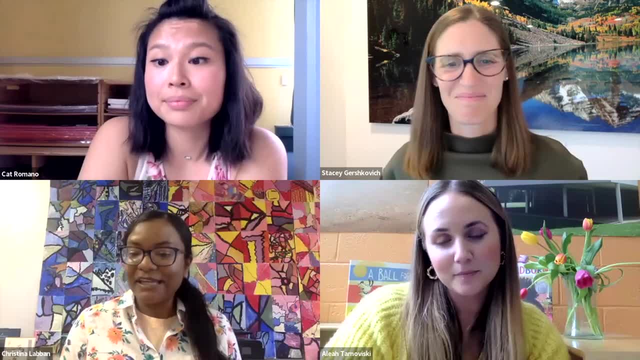 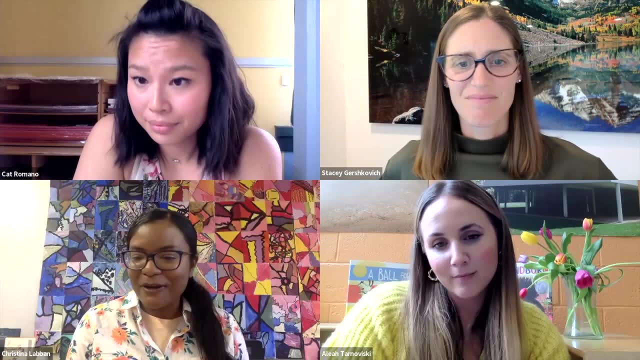 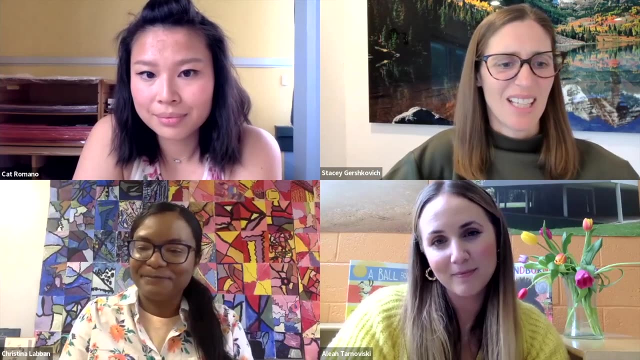 at this age, so they absorb so much so quickly and because we have routines set in place, they become familiar and comfortable right away. so you don't have to worry about your child knowing everything. they will learn as they go. yeah, I think all of that is great advice. 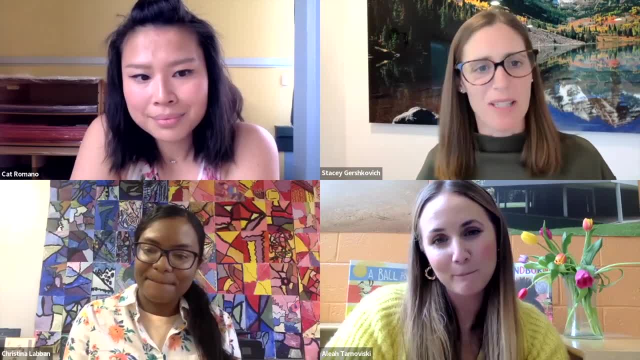 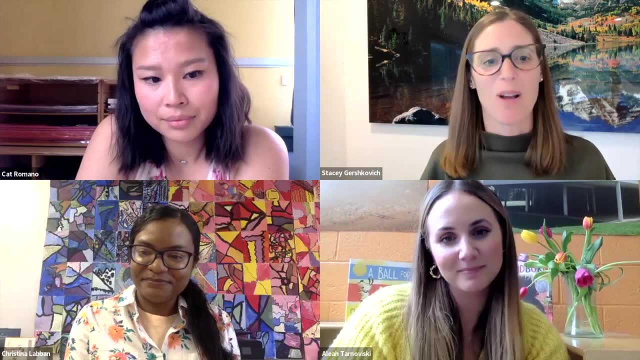 and I even think about my three kids, who, each of them, came to kindergarten with different strengths, and each of those strengths was really important. so we are going to talk in a moment. I would love to hear from you some concrete things that families can focus on, but I think my 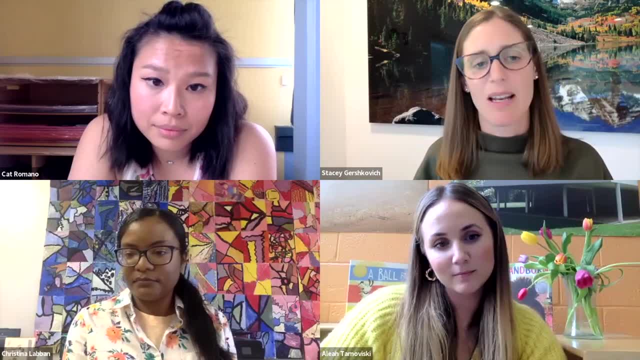 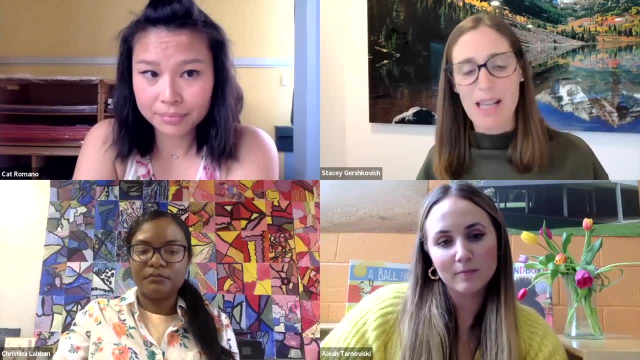 misconception that I come across most is that it is the academics that I should worry about the most. and I know in our conversations before- and I know you will talk about this in a moment- and I know from my experience as a principal, as a teacher of young kids- 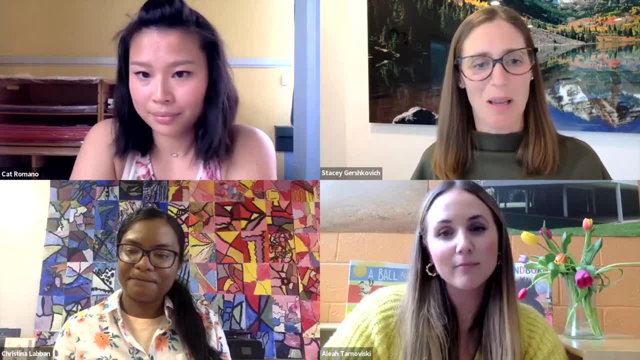 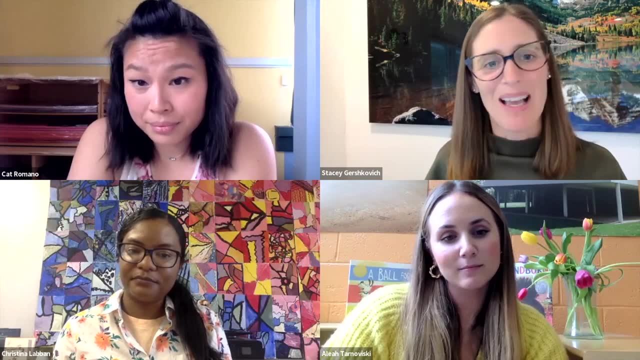 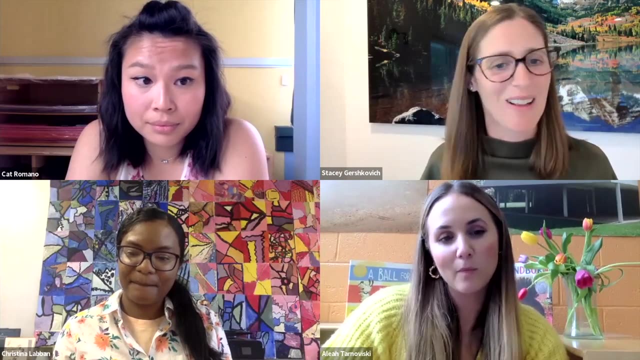 it wasn't the academics that usually was the the most important factor, as I remind my friends all the time that when they start kindergarten, guess what they are going to do on the first day of school: learn the alphabet right, learn other letters and if your kid knows other letters, 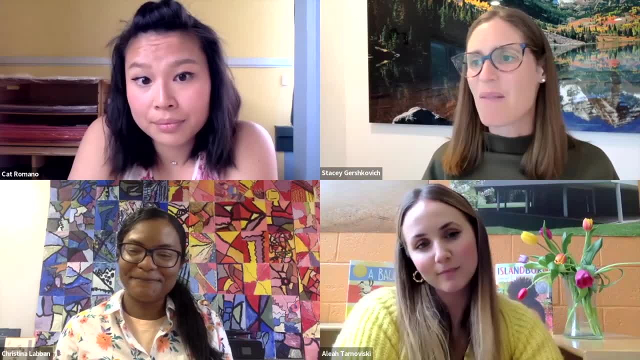 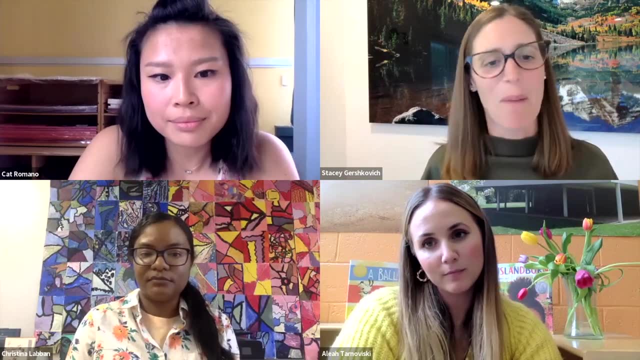 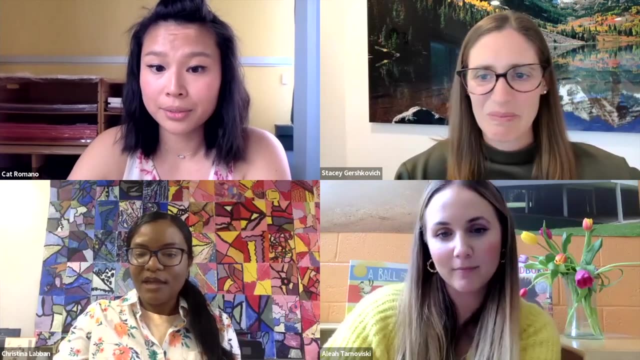 they will skip over that. but kindergarten is really about those foundational skills. so can you guys talk a little bit about some concrete ways families can right now start? we have a couple months to go before that first day of school, but what can we do now to help make sure? 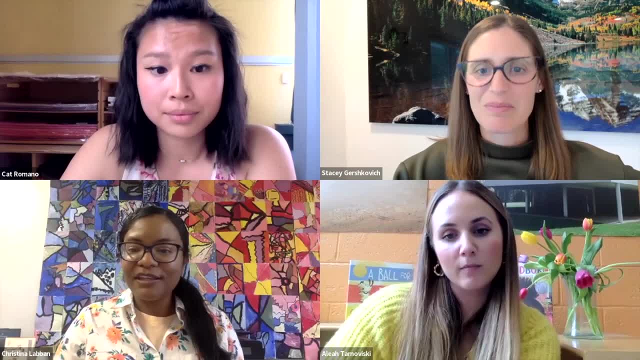 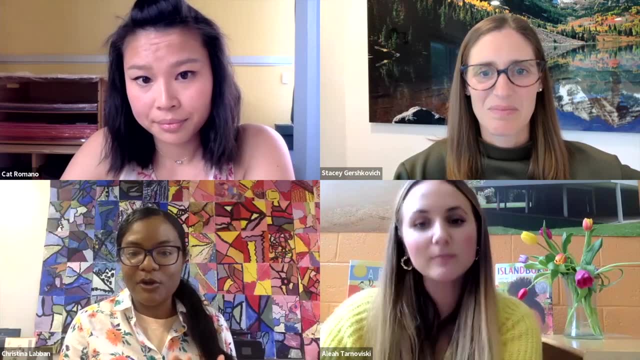 our kids are ready, I would say definitely going over how to use the bathroom independently, like knowing how to wash their hands and dry them, not being afraid to ask for one so they can blow their nose. practice handling their buttons on their jackets or zippers and sweaters. 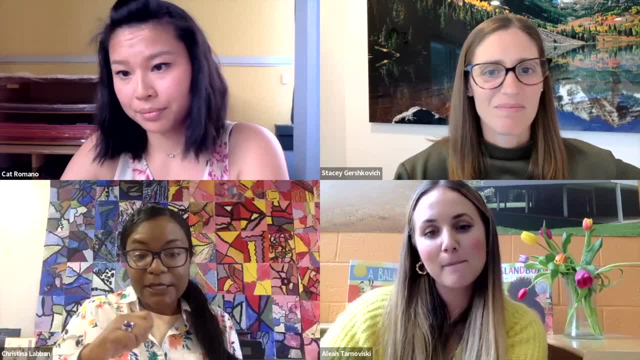 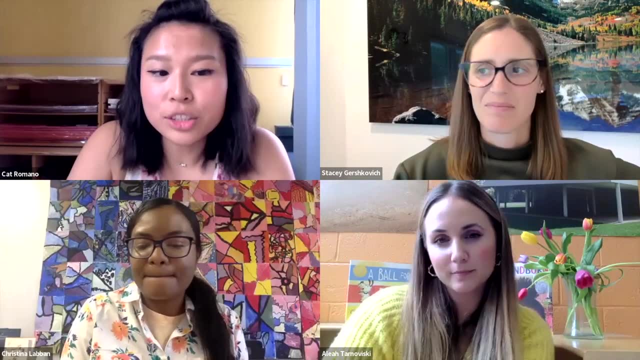 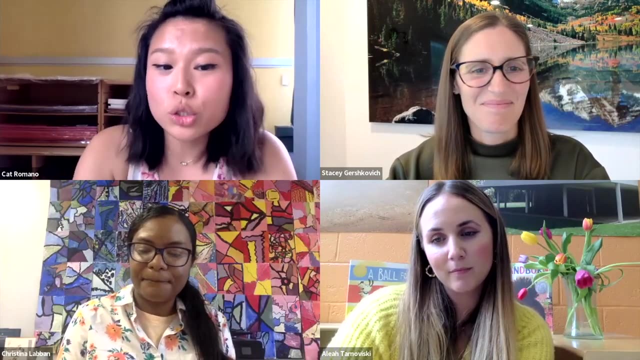 and working on fine motor skills like holding a pencil or crayons and coloring with a crayon and, I think, on the socio-emotional aspect of getting your 4 year old ready, or 5 year old ready, for kindergarten, helping them develop the language to express how they are feeling. 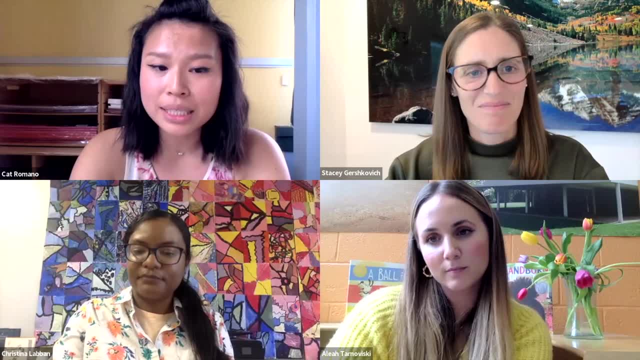 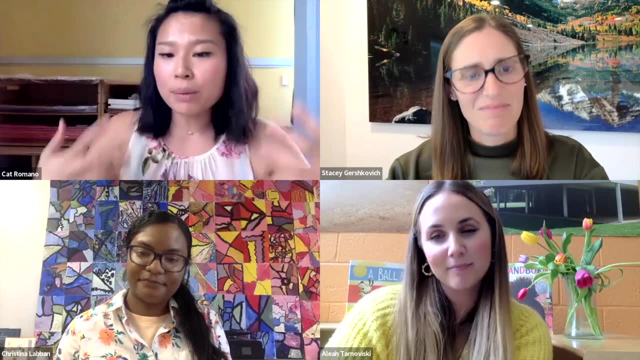 maybe going to the library and looking through books to name the feelings, because sometimes they might just be feeling something, but they have no word, they don't know what to call it, and so they'll say my tummy hurts, or they won't be able to tell me why. 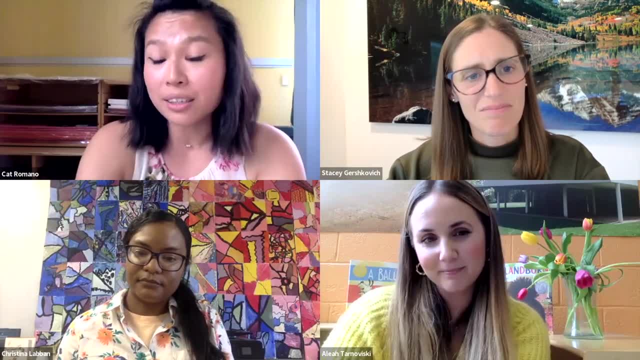 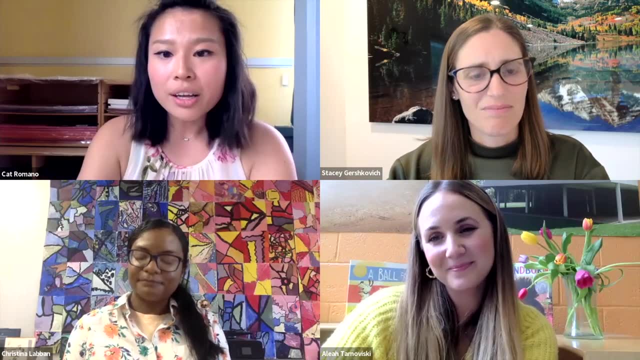 if they're upset they'll just say tummy hurts or I don't know. and so we have feeling books in school that we look through and we look at the appropriate faces and they're like it's that one and I'm like that's called feeling tired. 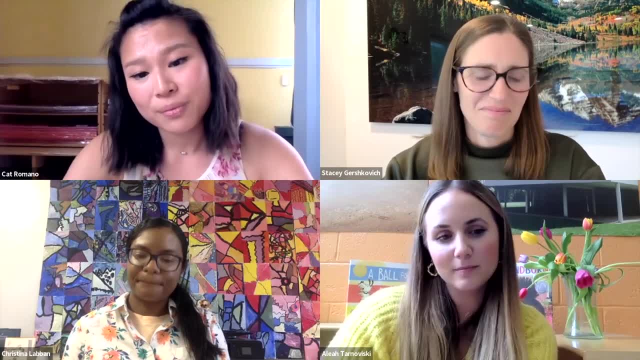 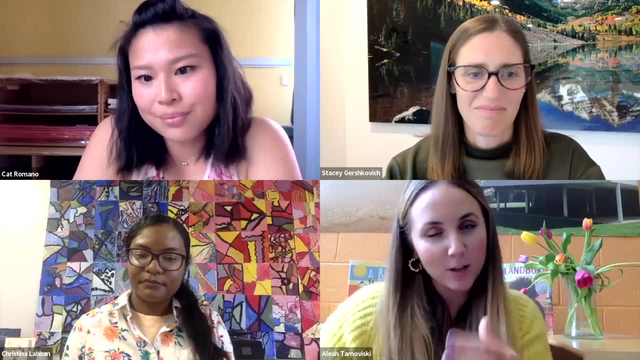 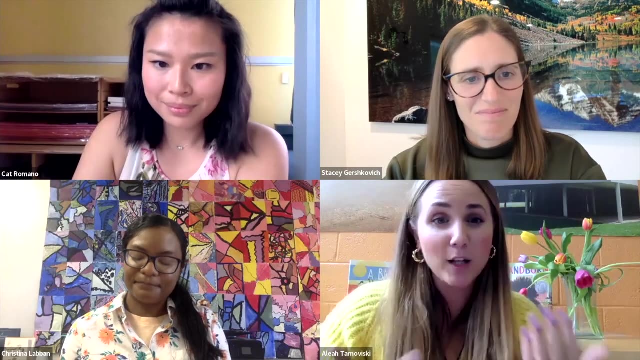 or feeling shy, and then I think, if you like that sense of readiness for a challenge, it looks different for a 4 year old, but knowing and preparing them and saying there's going to be hard things, there's going to be things that you know and you don't know. 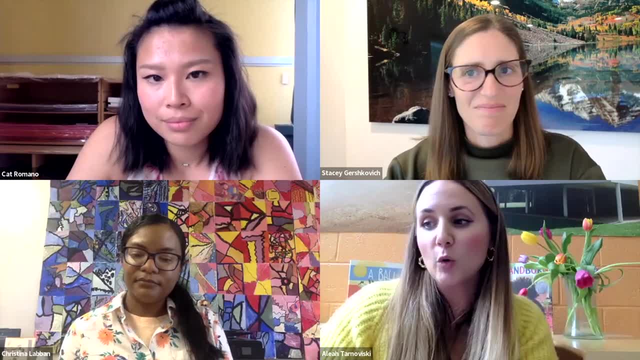 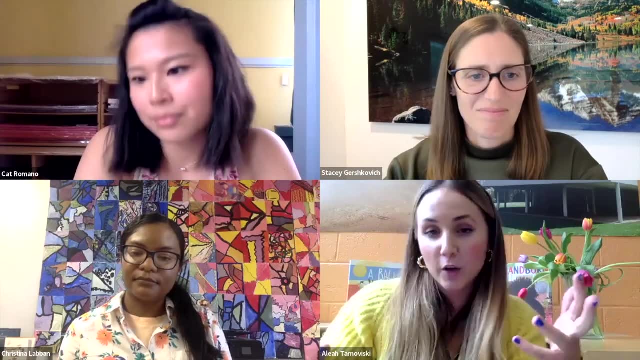 for the whole year of kindergarten, but particularly in that first week. and so not being afraid to speak up- and obviously that comes with the community being built, them feeling comfortable with me as their teacher or their classmates, if you want to start on the academic side of things. 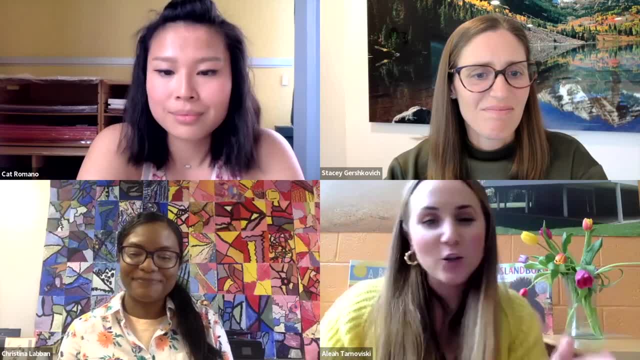 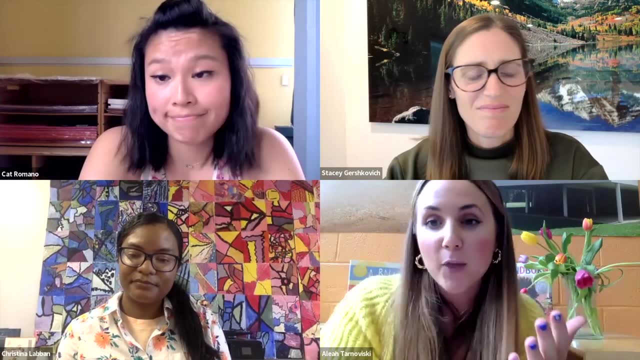 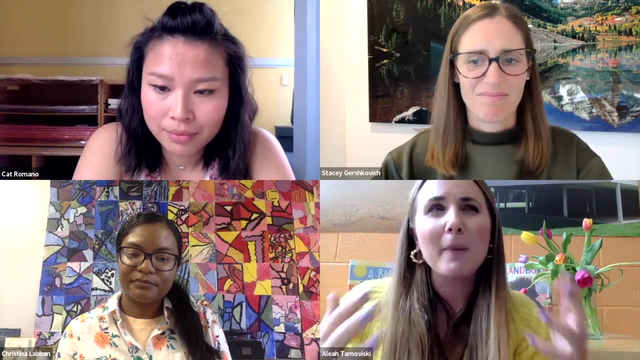 I'm not going to say go out and buy the workbooks or start having them read books. go to the library and get books that they love and maybe point out the letters that they see in their name. have them practice writing their first name or show them what their first name looks like. 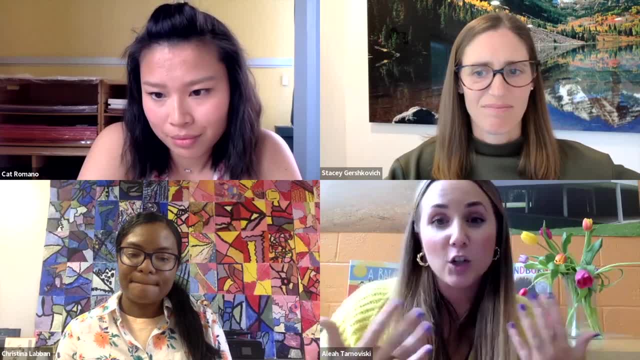 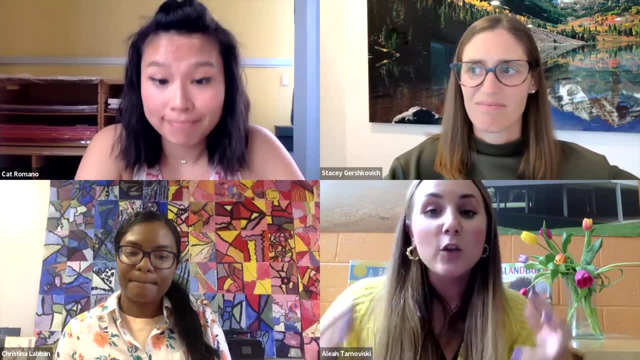 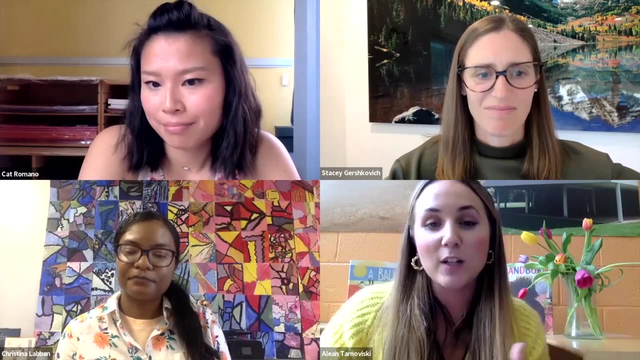 probably some obvious things that you're already doing are actually giving them the foundation that they need. so if you're bringing that excitement for seeing letters in the supermarket, those are the kinds of things that are setting that excitement for learning that is really going to blossom once they get to school. 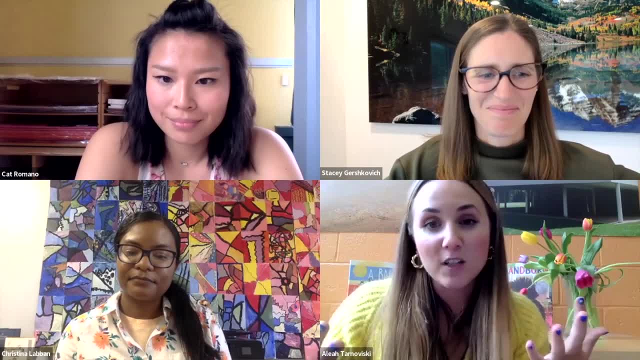 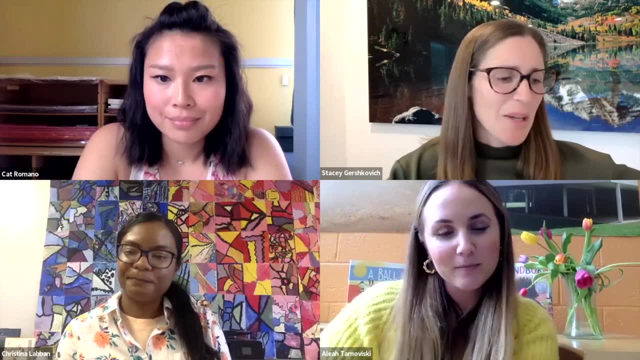 and so if you're doing those things, keep doing them, and if you're not, they're really easy ways to just start getting them thinking about what they're going to dive into when the school year begins. I think that's a good point: making sure our students realize. 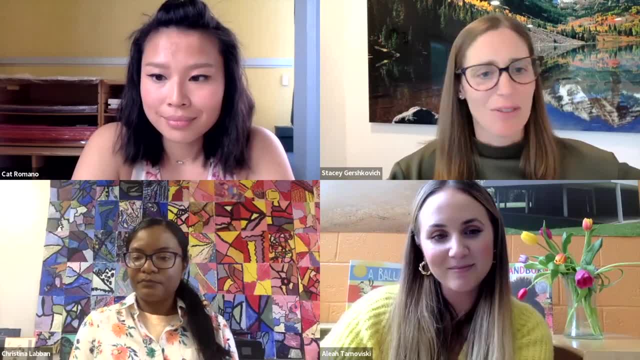 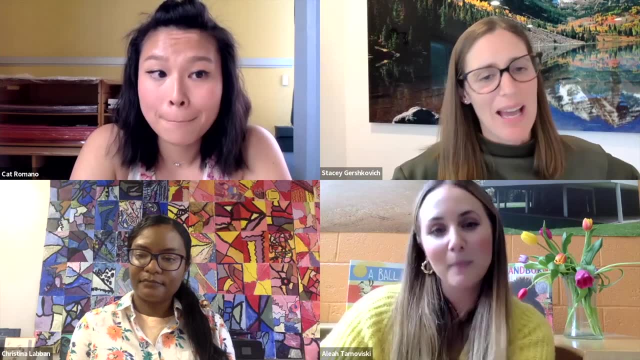 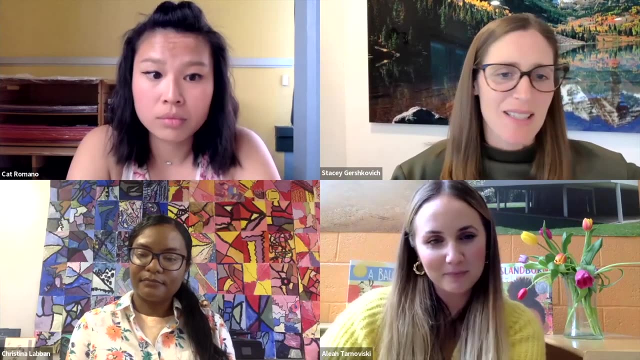 that the learning that they're already doing is the type of learning they're going to do in school. kindergarten is not that different in school, similar to the counting objects that they do at home: how many pieces of cookie do I have? how many steps does it take? 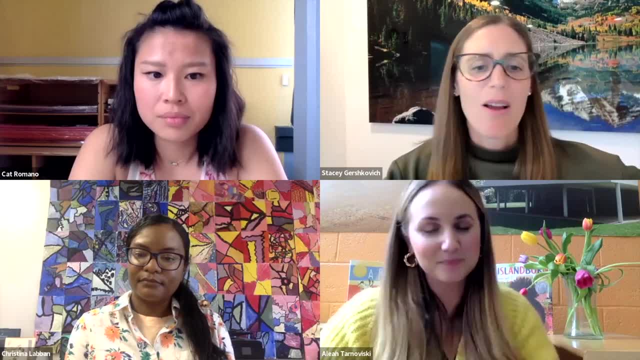 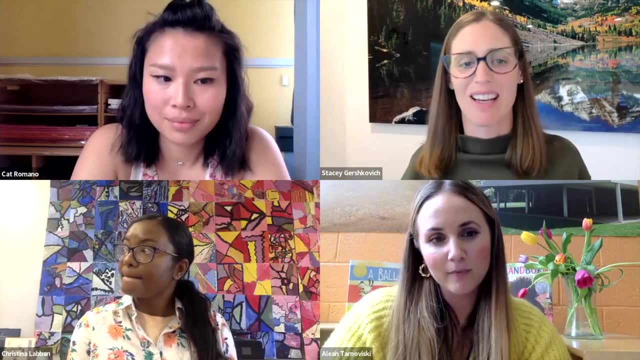 for me to get to my closet, whatever it is, the type of learning that they're doing at school- they're already doing it now- and giving them the confidence to recognize: oh, I'm doing this. that's kind of what you're going to do in kindergarten. 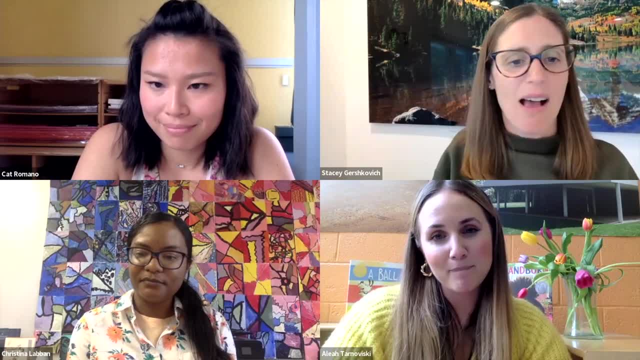 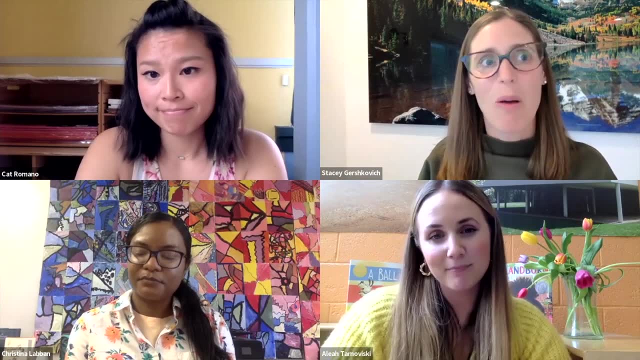 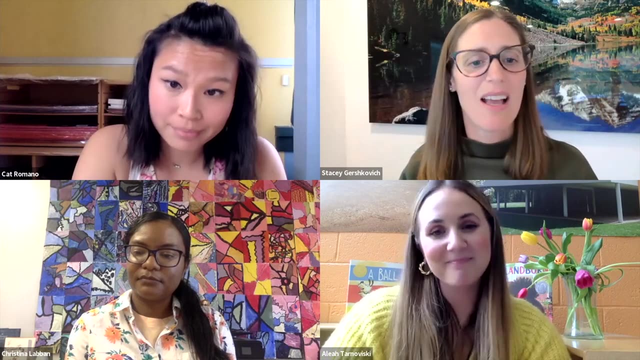 look at that. you're already doing it, and so the focus I think, Kat, you were speaking about is really naming those emotions that you're feeling is a really good one. you know us as parents, maybe know how our child's feeling, and so we don't necessarily need them to articulate. 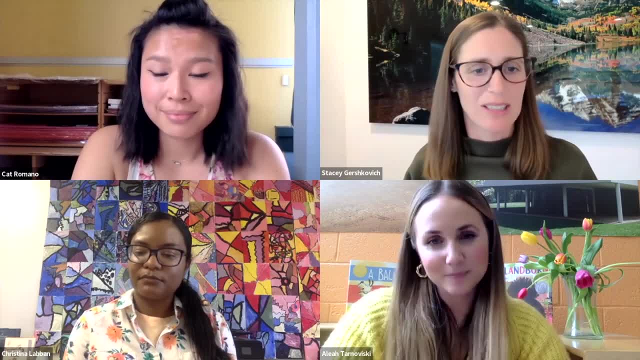 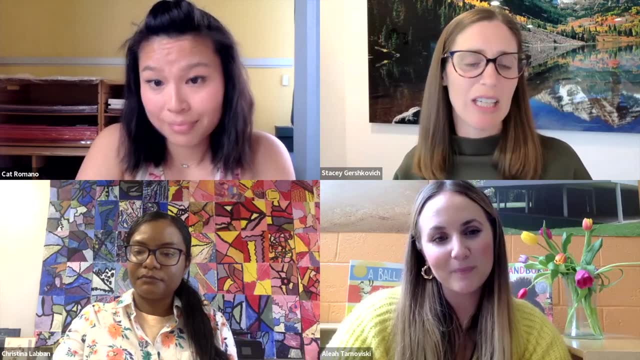 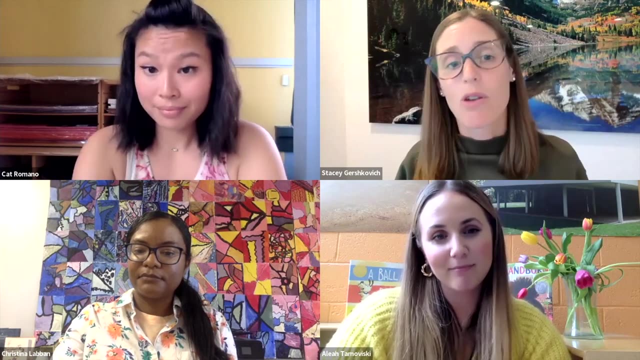 what it is, because we're much more aware of how they're expressing it and what their tendencies are. but I think that's a really great idea of using those books. you know, you seem to be feeling sad right now, or it sounds like you're feeling nervous right now. 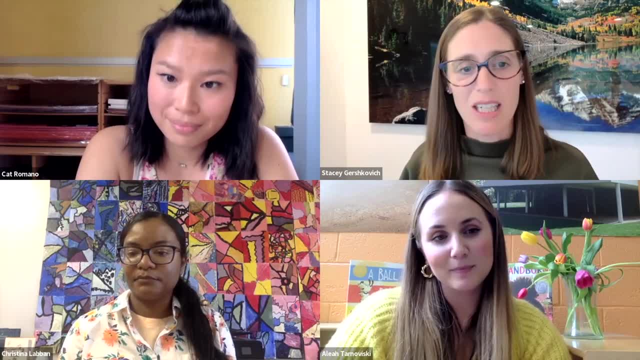 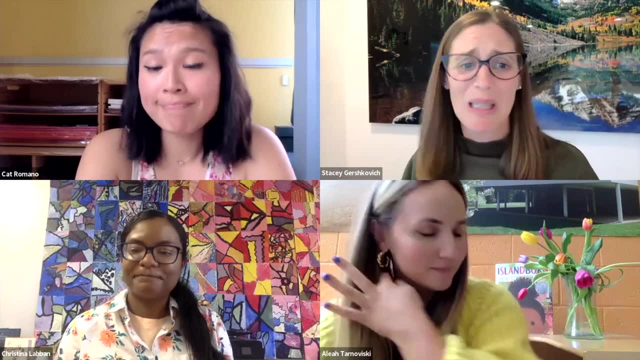 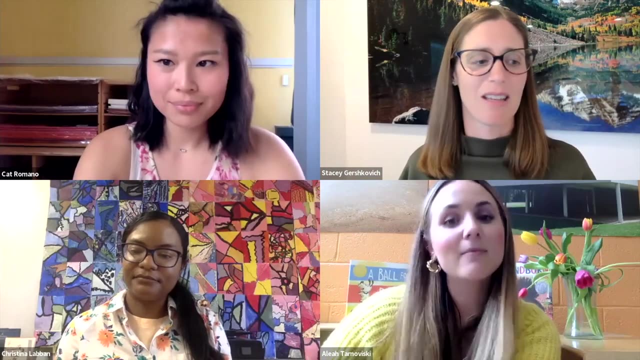 sometimes, when you feel nervous, your tummy starts to hurt- and getting kids to be able to articulate. you know, I think, Christina, you were talking about like raising your hand and saying: I need something, I need to go to the bathroom, I need a tissue. I'm thirsty. 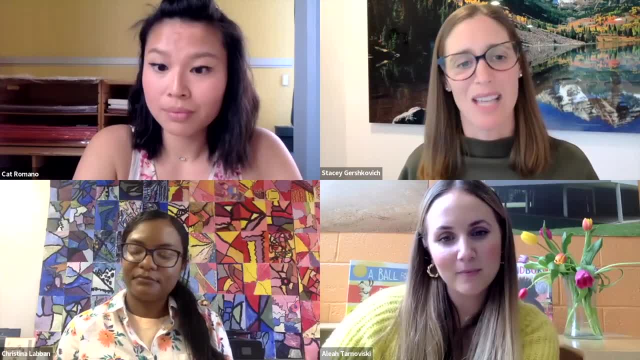 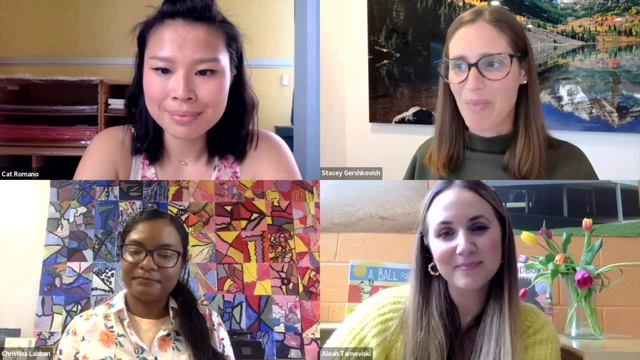 being able to raise your hand and say what you need again. as parents, I think often we know what our kids need, and so now is the time to kind of say: I need something so that when they're in school they feel much more confident doing that. okay. 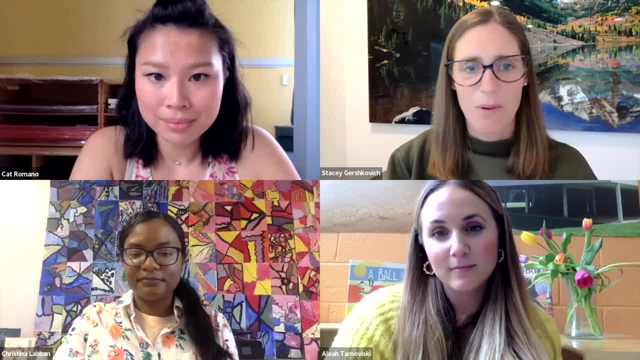 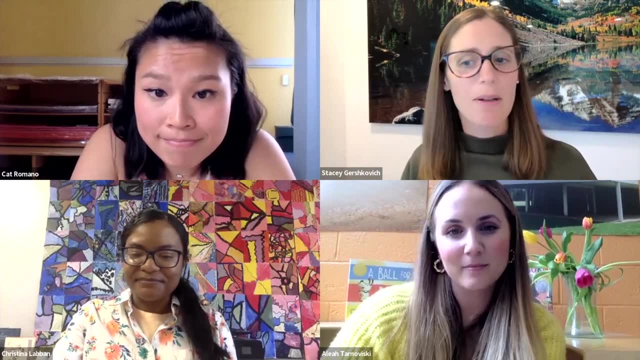 well, we're going to go to that question and answer, unless there's anything else that you guys want to talk about before we do that. we've got a lot of questions to get to, okay, so there's a couple questions coming in about homework. can you first speak to? 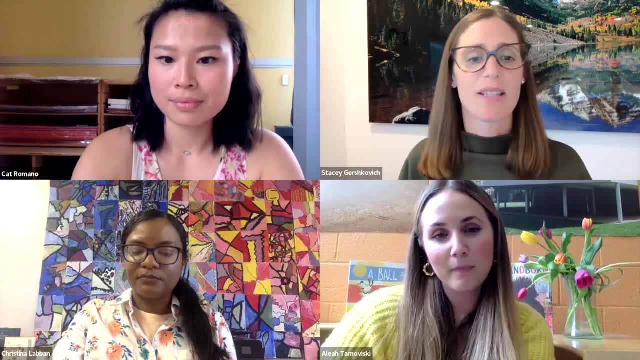 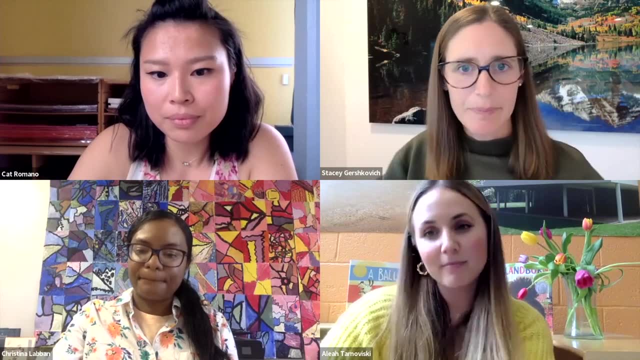 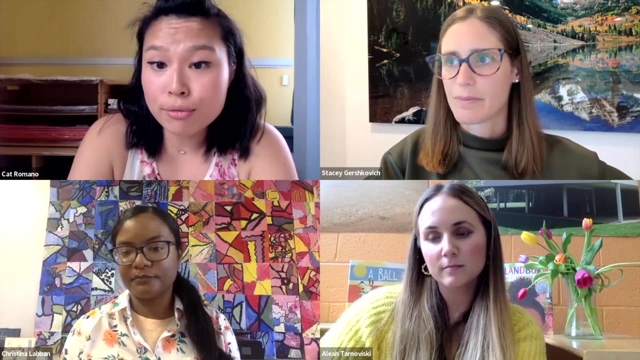 the purpose of homework from your perspective and then give a sense of what homework looks like in your classroom, knowing that obviously homework looks a little bit different in different schools. I think for me for homework it's about three pages a night for kids and I think it's purposeful for two ways. 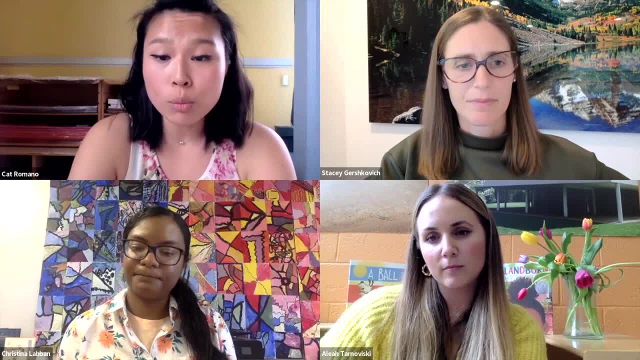 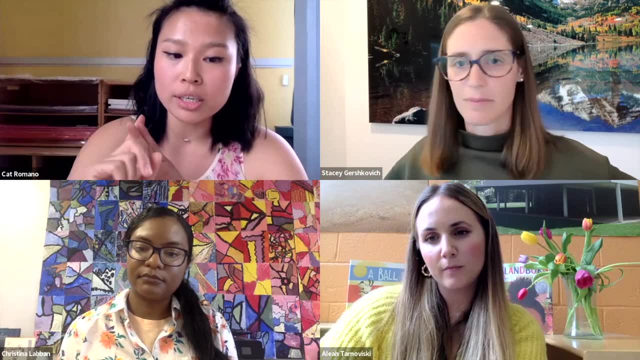 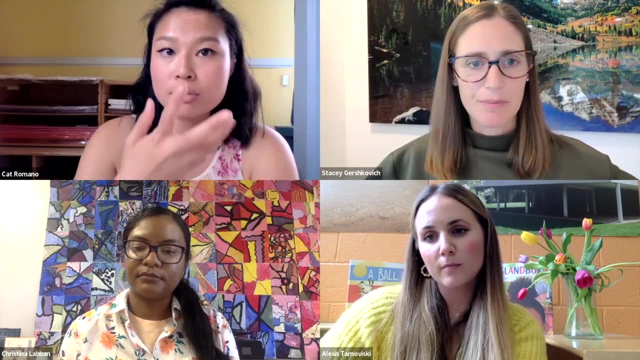 in one. it's showing parents what kids are learning in school, because often homework is a reflection of the type of classwork we do in school and it helps children with their motor skills of practicing writing with a pencil, and it also just helps for kids to review what we've done. 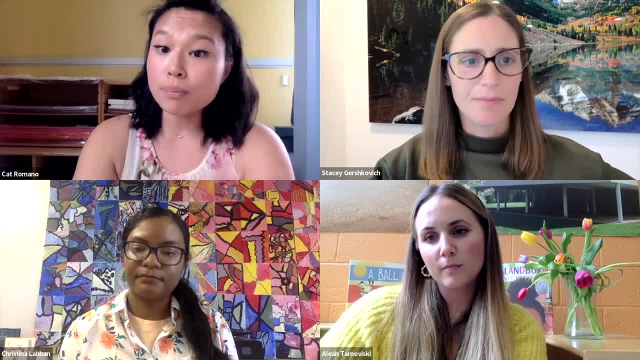 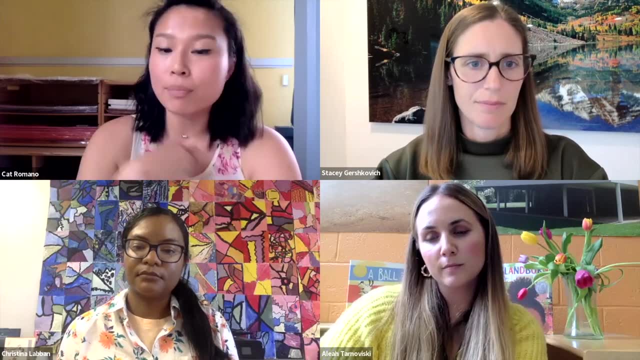 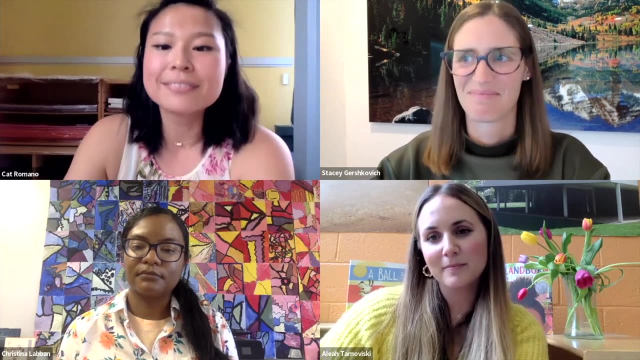 in school and get extra support from parents as well, and then come back the next day to try again in either small group or just like show off in morning meeting. being like I practice my homework, I am able to write my name. I can trace the letter N. 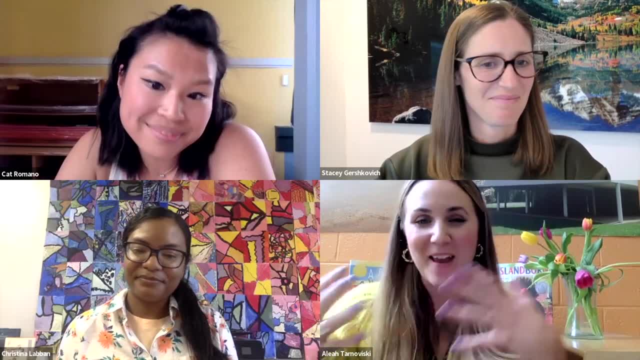 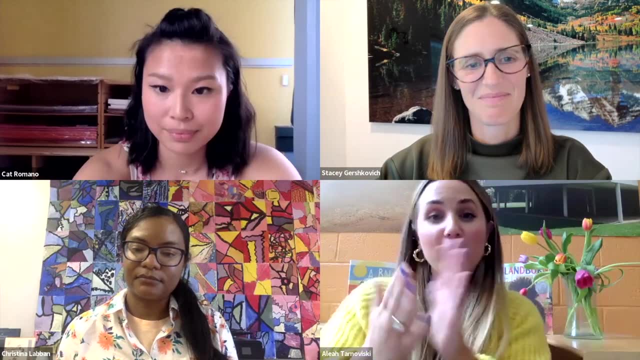 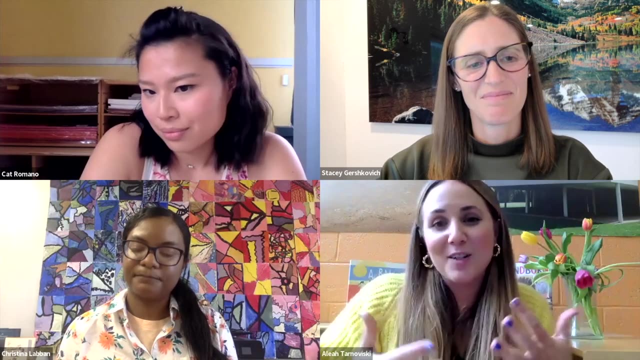 yeah, and I think hearing like three pages it might feel like a lot but say multiple pages. like I know in my school in kindergarten it's usually around like a front and a back, like the morning work that that scholar held up, but it's definitely scaffolded as we go. 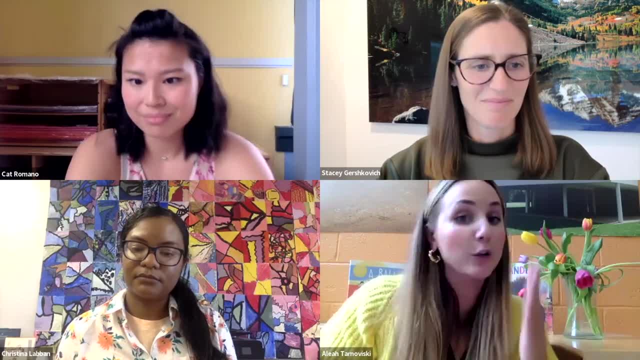 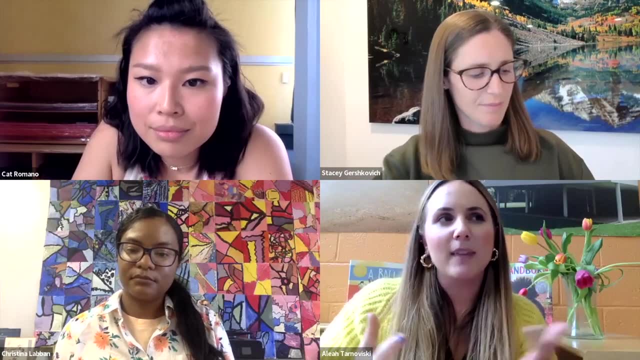 so at the beginning it's going to be a page of writing your first name and then maybe by the third week of school it's writing your first and your last name on a tracing sheet and then some counting on the back. so what I tell parents is: 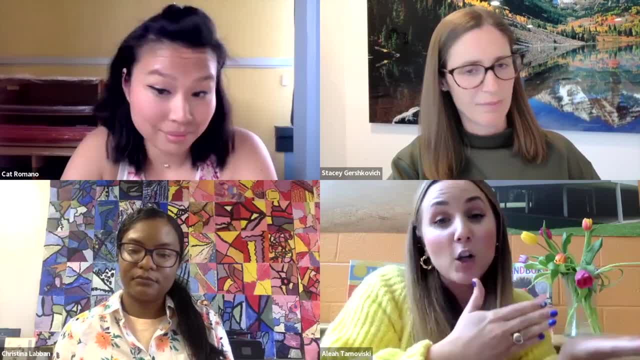 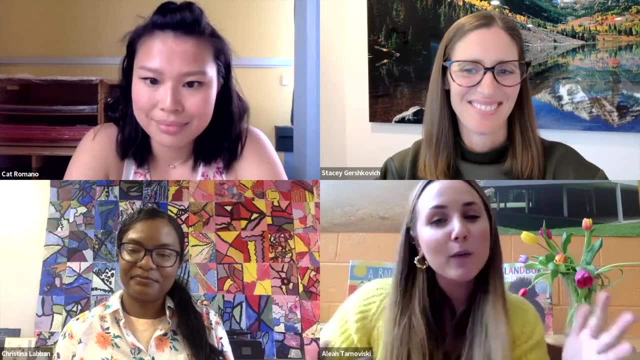 it's going to be about. it should be like 15 minutes of independent work, maybe closer to 10 at the very beginning. I want them to go outside and play. I want them to have dinner with their families. we want them to be doing all those things. 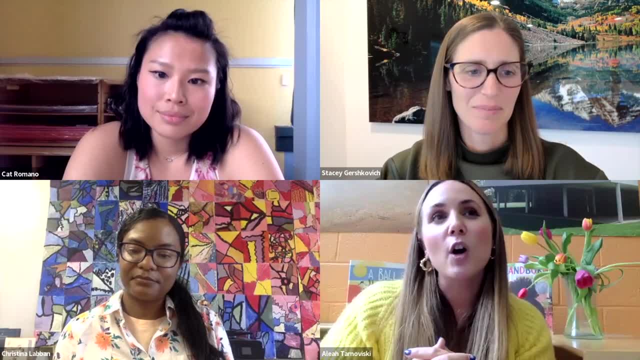 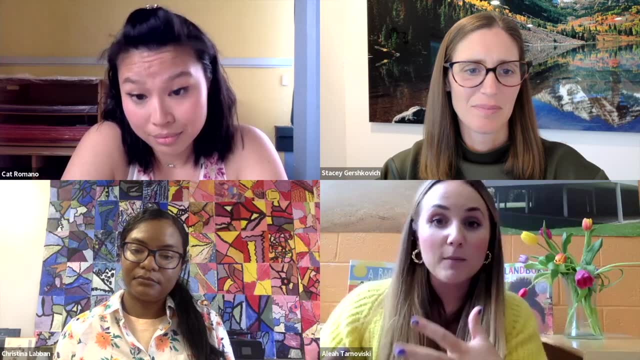 that are so important for them to become little people, and so, like Kat was saying, it's just to reinforce, particularly at the beginning of the year. it's like writing your name, maybe doing some number tracing, just some things that we know they may need some extra practice in. 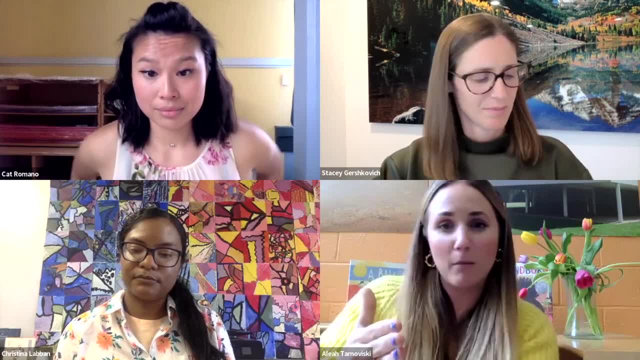 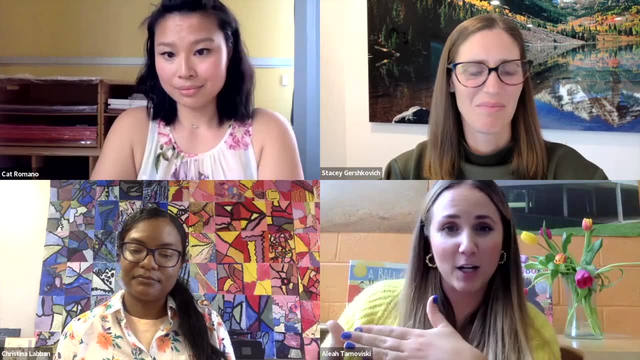 and what I always tell families is, if it's taking them, like when you reach the 20 minute mark, like they're gone, give them a break and at the end of the day, if it's not done at dinner you say: Miss T, this is how far we got. 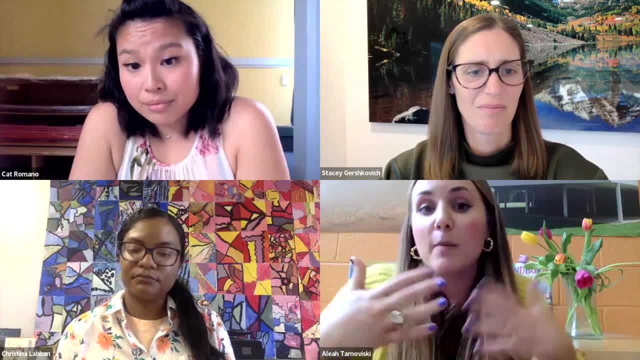 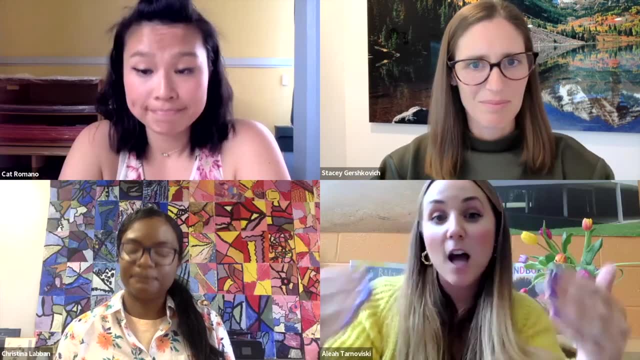 like that's a sign to me: okay, you've got to put some supports in for them at school and at home and I can give them different work. so I think all teachers are not sending work home and saying: just get it done. that's not like we're a team. 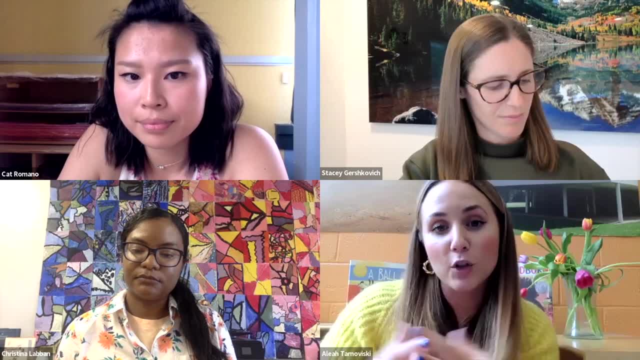 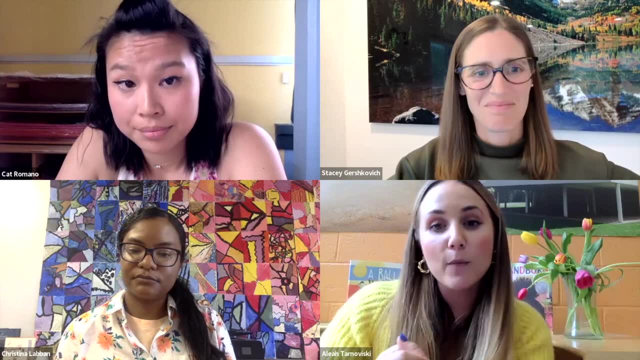 we're a partnership and so it can be an opportunity for you to kind of get a picture of where they're at with things, and then for me as well. I think it's really important to be able to do that independently and Stacy. I see a question about tablets. 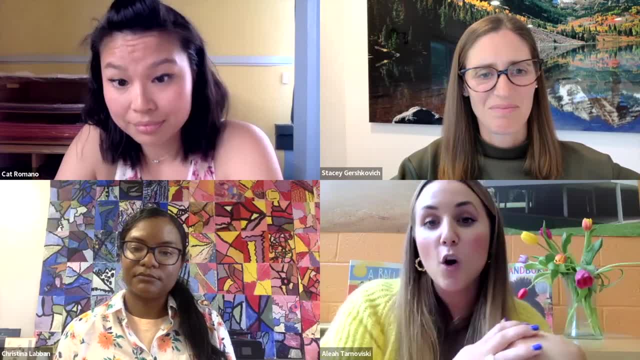 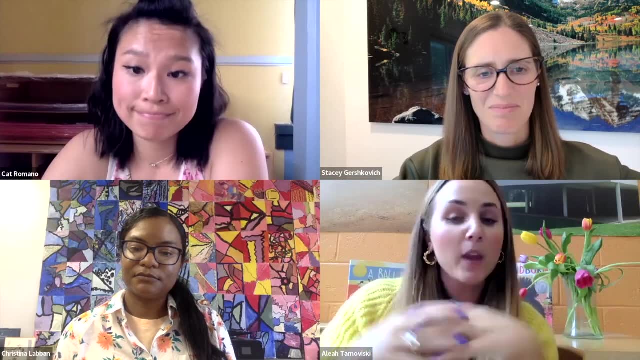 I know at Success our scholars use tablets. I know that in my room we're still giving paper homework. we're still doing paper morning work. I know for a lot of our kindergarten teachers we're still making sure like they're getting those motor skills with a pencil. 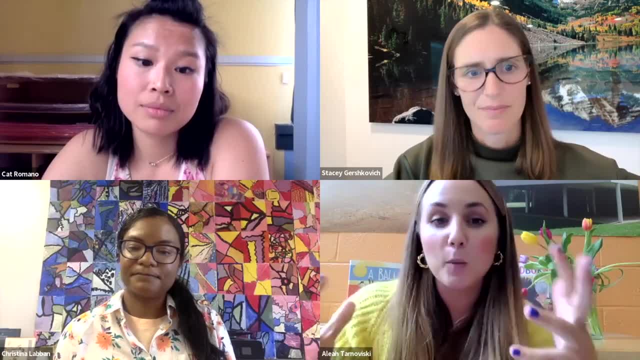 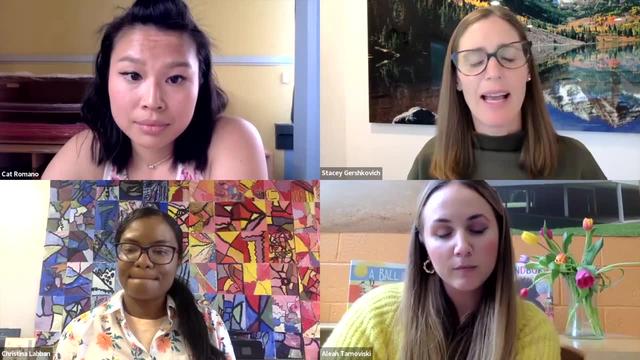 and so wherever you're going to school, it's most likely going to be paper homework- that they're able to practice holding a pencil and things like that, for I think that's a good point. that homework really is about A the parent seeing what the child is doing in school. 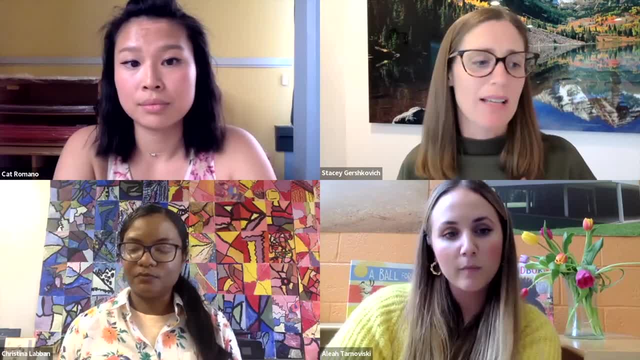 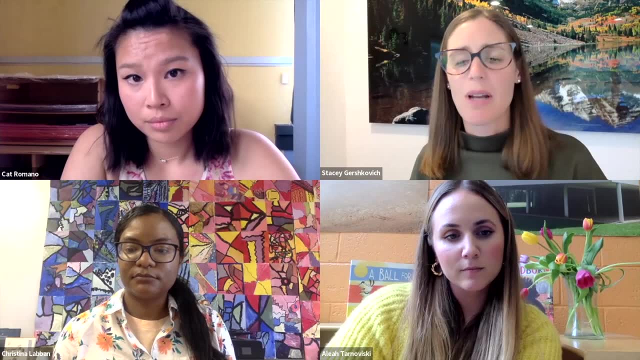 and seeing how they're doing with it. so you should see homework as a little bit of a glimpse into the classroom for you. and then again, as Aliyah pointed out, it is also an opportunity for you to communicate to the teacher how your child is doing when they're not in the school. 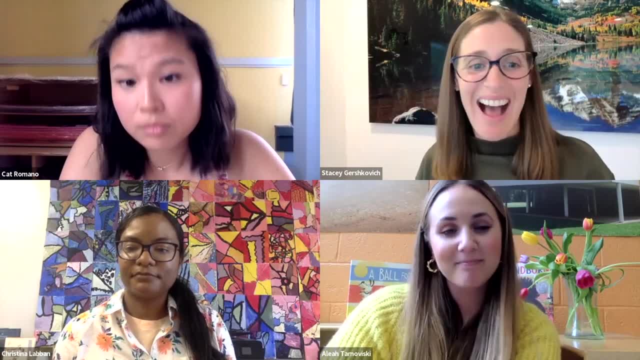 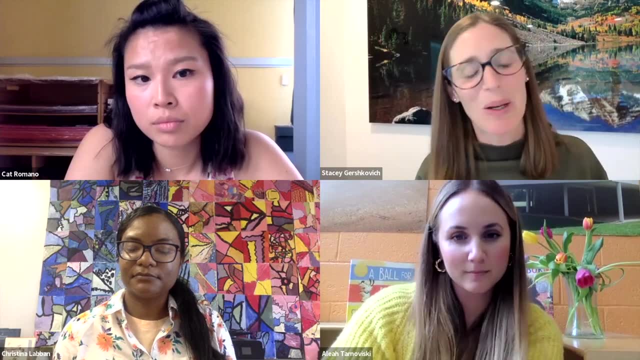 sometimes we have kids who do better at home. sometimes we have students who maybe at home give their parents a difficult time and they can do things at school, but they won't do them at home. all of this is information for the teacher and for you, and so 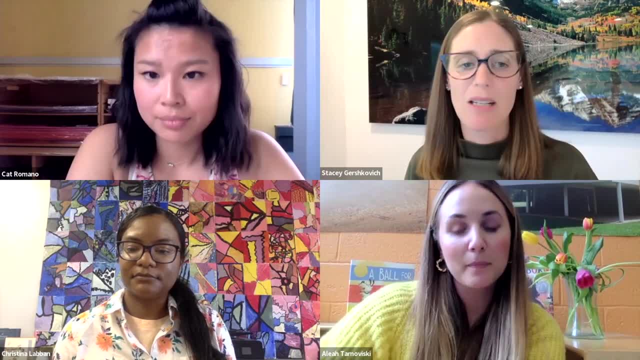 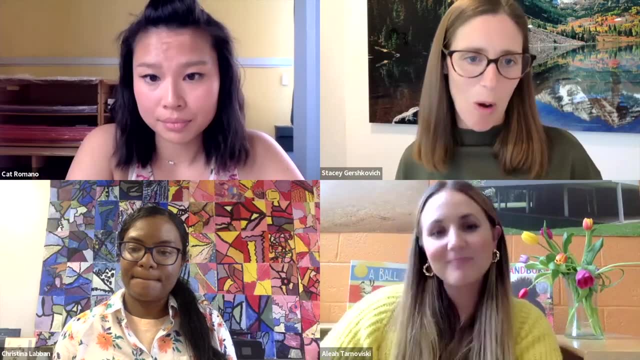 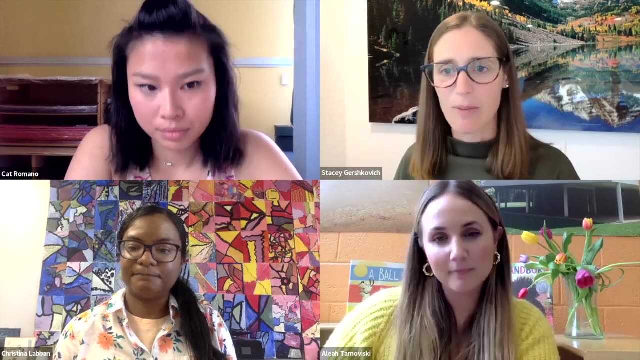 if homework is taking an inordinate amount of time, that's a time to speak to the teacher and certainly not the expectation that it is becoming a tearful fighting moment. that is a time where you stop and you say: this is how far we got. can we talk about what we could do? 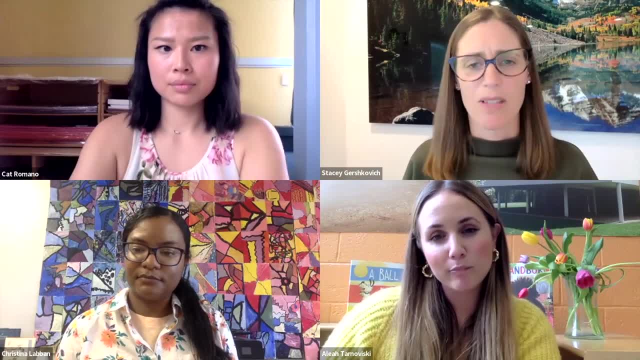 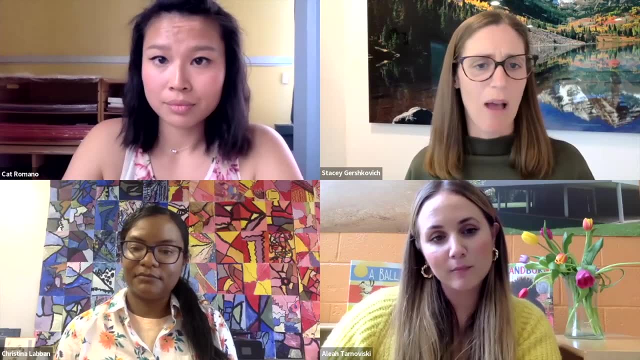 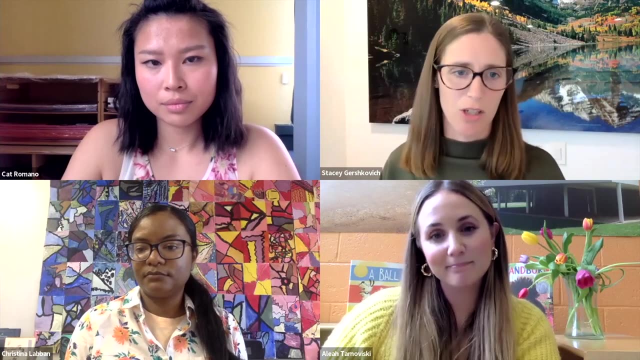 so that leads into another question that has come up a couple of times. obviously, as you mentioned many times, kids come in at all different places. so what are some structures you have in your classroom so that students at different levels are getting support, so that they are not bored? 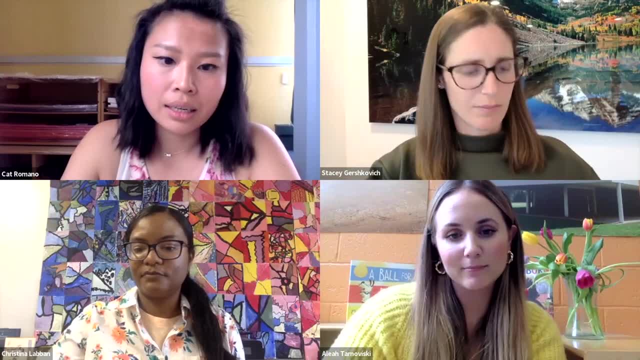 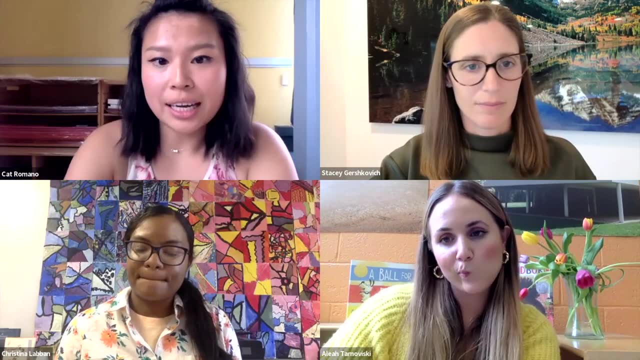 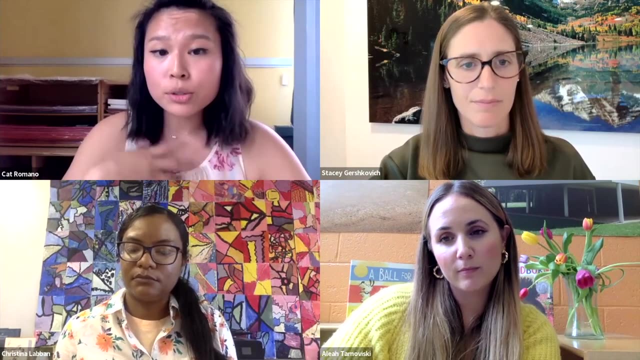 but they're also not frustrated. in our room at Success Academy we do have two teachers, and so at the beginning of the year it's kind of like a little bit of a. we have to put the students together because we just need to have everyone feel comfortable. 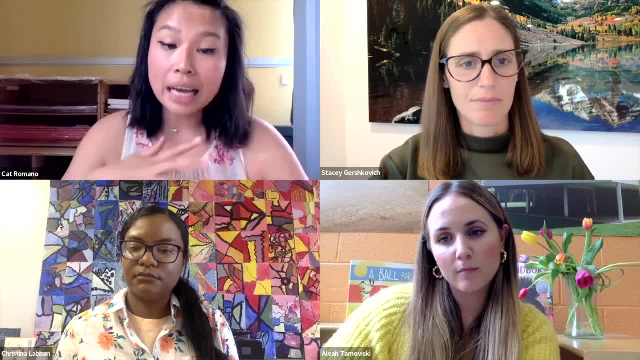 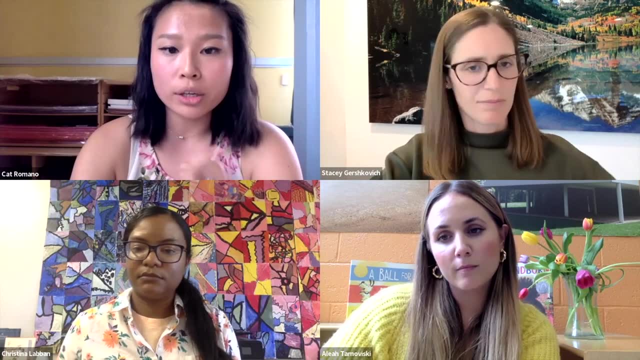 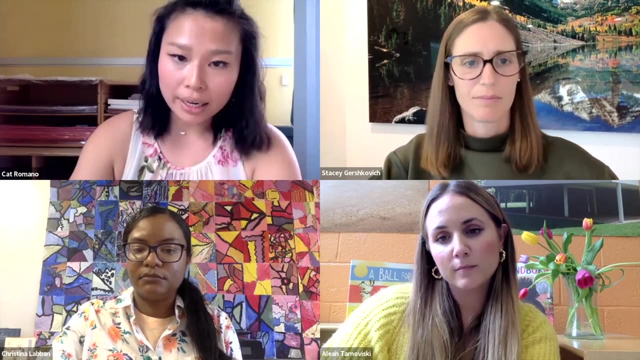 learn the routines and then towards September, October, then we can sort of split up the groups and create scaffolded work based on their needs and their learning at the level, and then we split up with our two teachers, or sometimes across the grade, depending on where kids are falling. 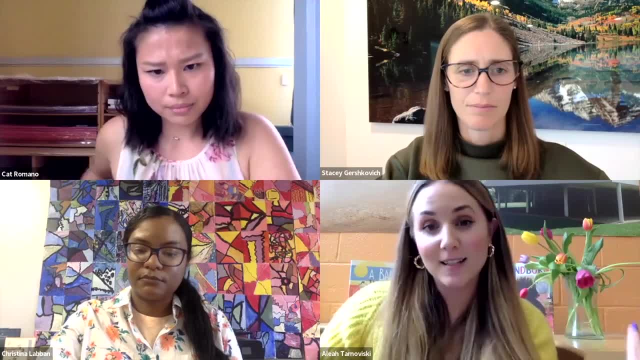 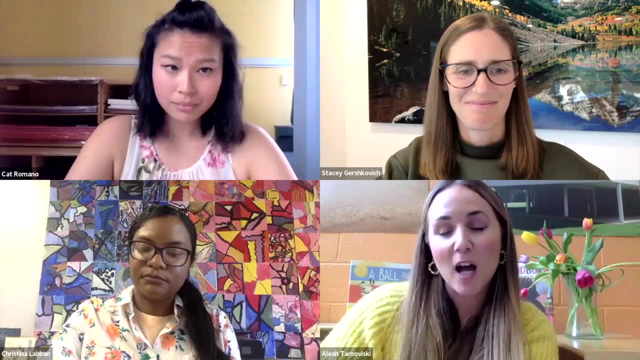 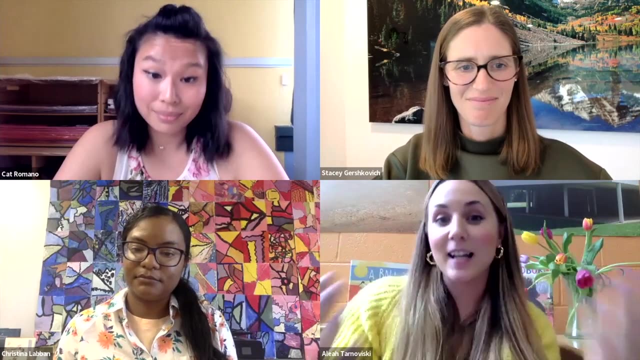 in math, reading, phonics levels if you're not coming to Success. and you know, like I went to kindergarten, there was only one kindergarten teacher and there was 20 something kids on her rug. I think feel at ease that kindergarten teachers are ready for this. 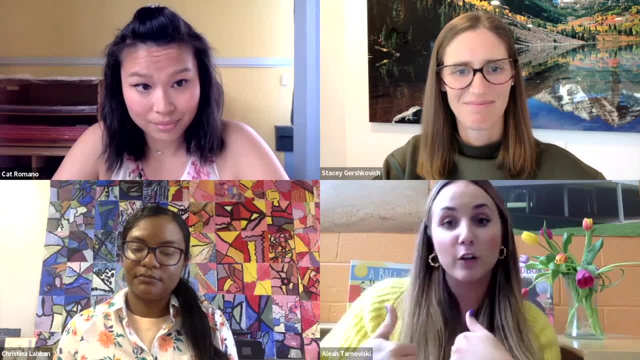 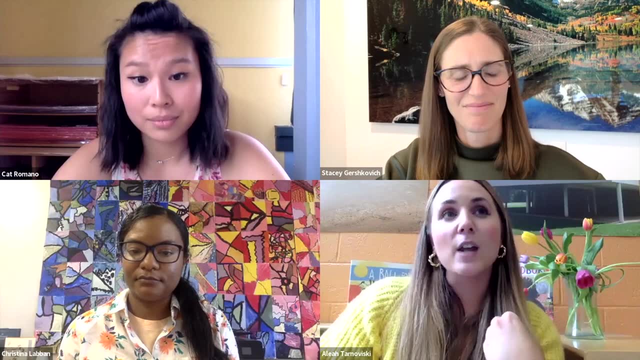 like I said before, we know we're going to get kids coming in that can write their first and last name and can count to 50. I know that I'm going to get scholars that are just learning how to write their first letter, and what I think is cool about kindergarten is 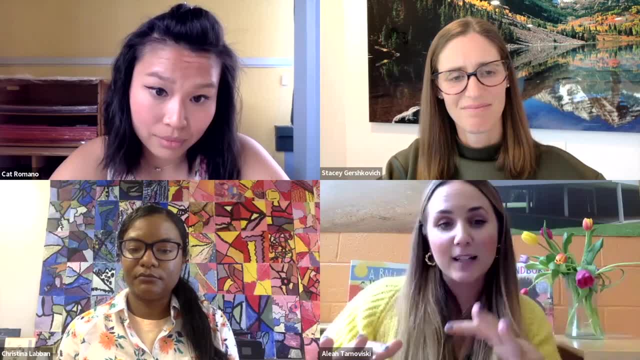 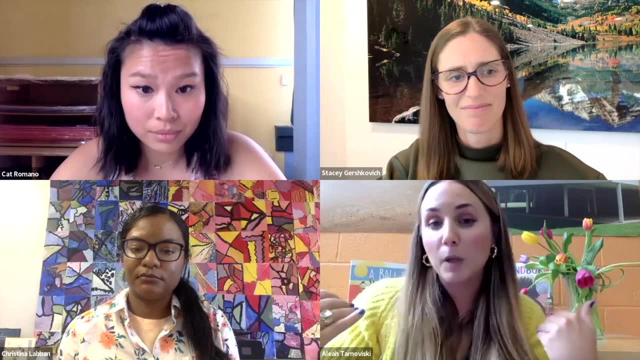 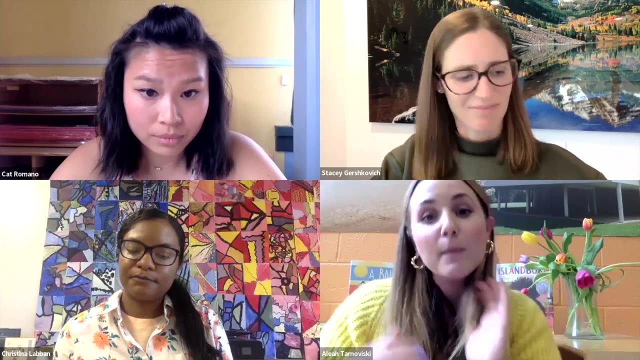 that it's not just about the number of students and the number of students that you're going to go to. it might be center time, so kids are working on different level activities and then they're coming and meeting with their teacher in a small group. that often happens in math. 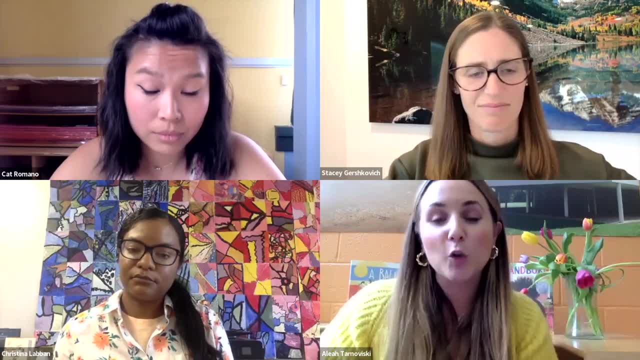 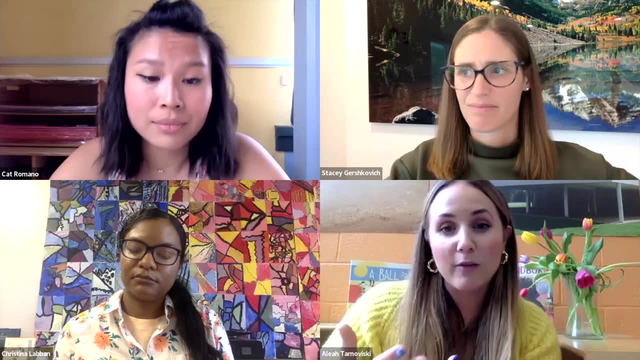 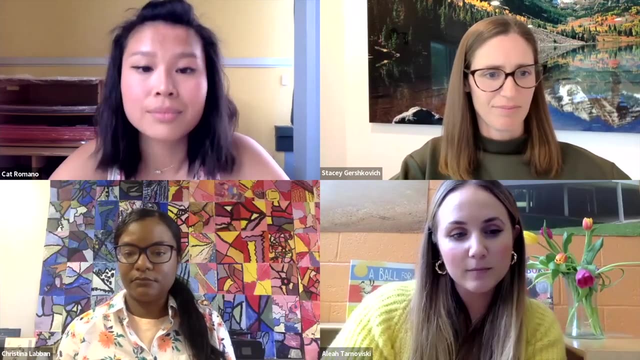 and also happens in reading and that's mirrored in what we do at Success. but most early childhood rooms will have some kind of center time for reading and math and that's something that we do on a similar level that are able to challenge them, to make sure that every kid is challenged. 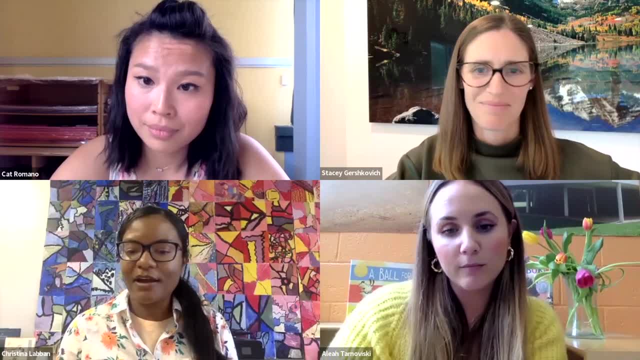 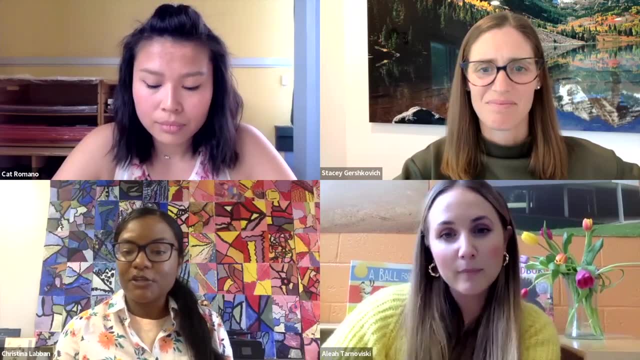 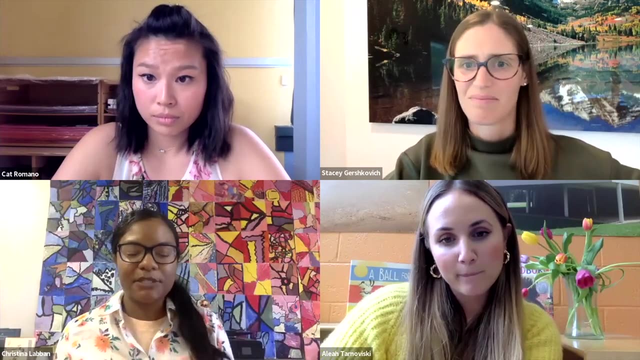 and met with what they need. yeah, I agree we have a larger classroom setting, but then we also do break off a lot of times into small groups so that the small groups are catered to a smaller group of students and it's working on its particular skill. 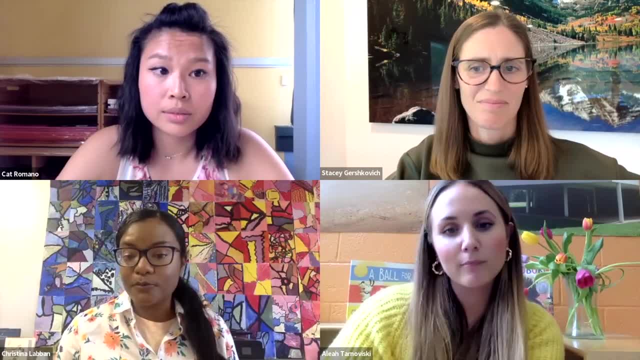 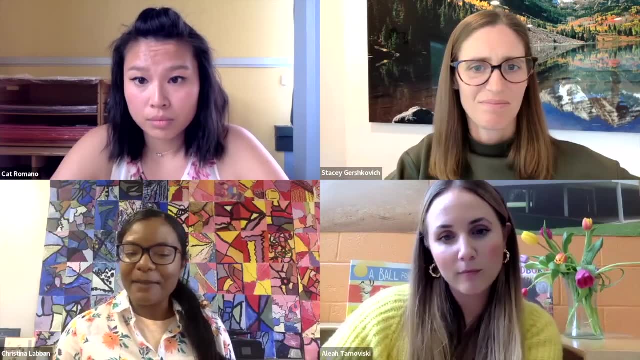 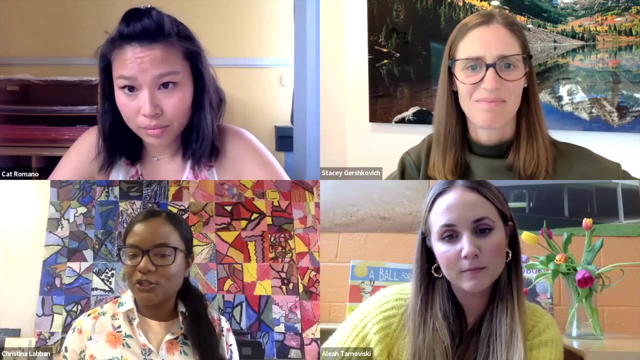 or sometimes parents will access for extra supports at home, extra packets, extra work that they might want, and then for scholars who might be able to be challenged a little bit more, I'll send them home extra things to work on at home with their parents, like extra challenge tickets. 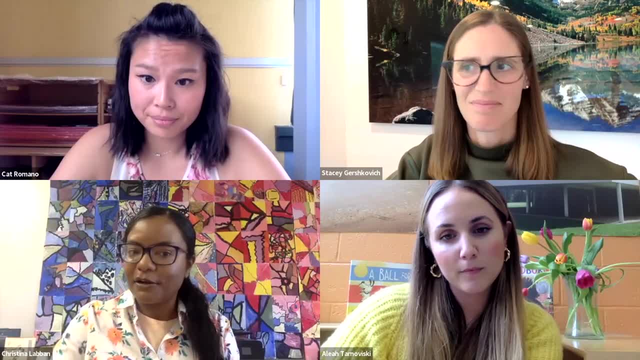 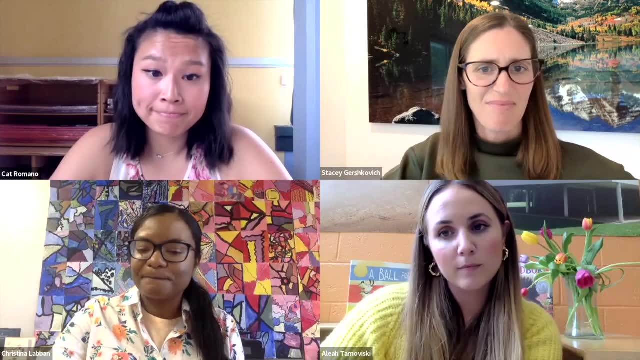 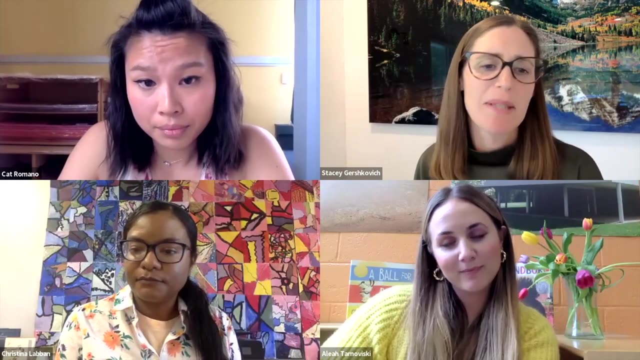 the same concepts, maybe different numbers, things like that. so we definitely are prepared to handle the students coming in at whatever level they're at. what about if there's a parent who kid comes home and is feeling upset? maybe there was a child who was mean to them? 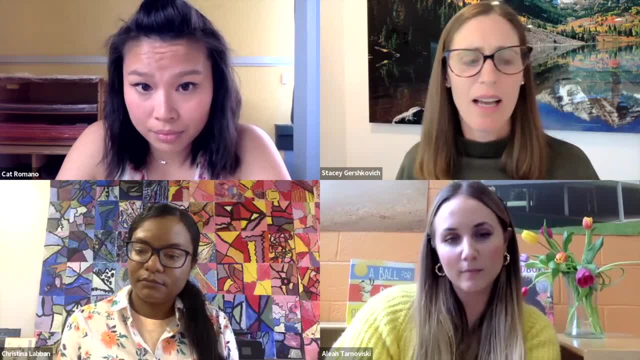 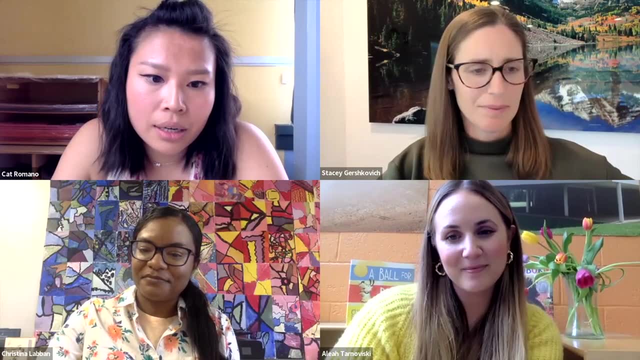 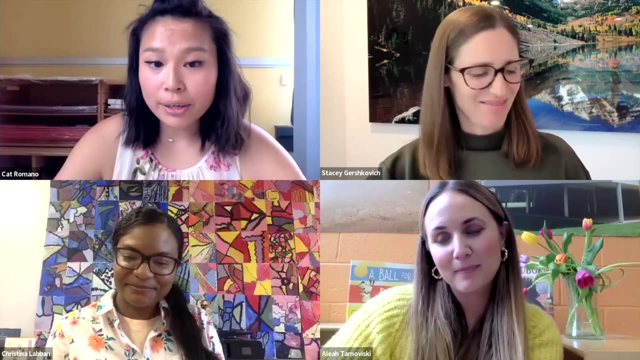 or there was some situation that made that child come home feeling maybe sad or upset or angry. how should a parent handle those situations? what do we do? go ahead okay. I mean in our classroom space. we really try to have our kids feel safe. we try to make sure. 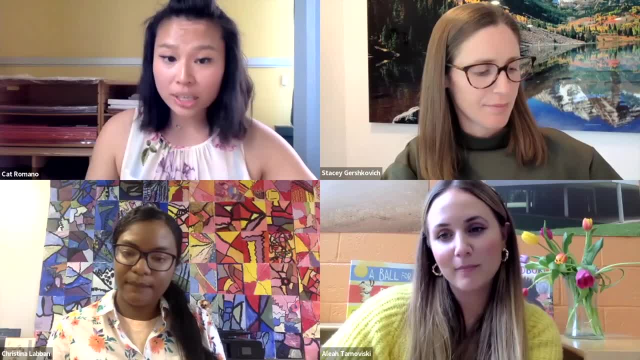 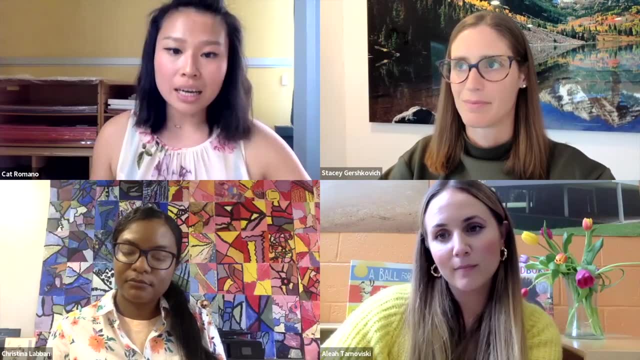 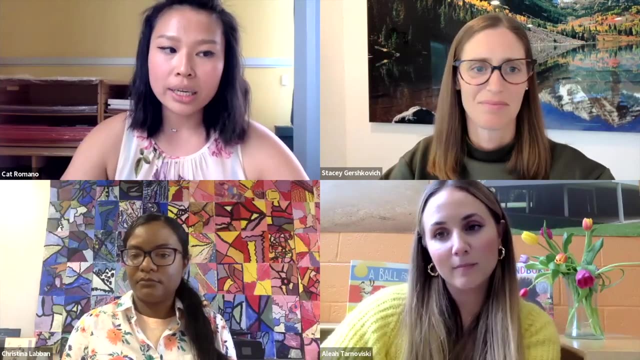 that when something happens, we always have eyes on the kids so we are watching. there's never a time when they're not being watched by an adult, so we always try to catch it. but there are times when maybe we did miss something, like in the line. there was like just a little. 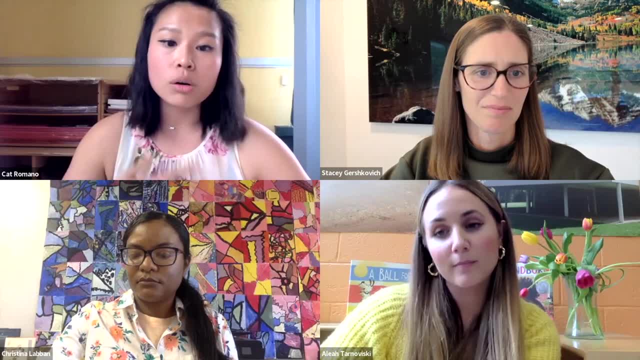 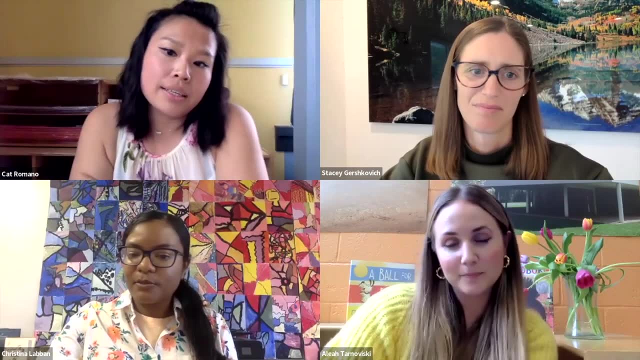 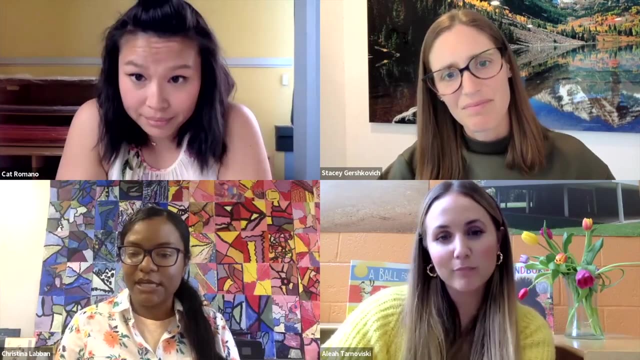 hand, touch somebody else and we encourage parents to just reach out to us first and we try to make sure that the child is feeling as needed. I think it's also important just to validate your scholars feelings. so whatever they're saying, they're feeling that you agree with them. 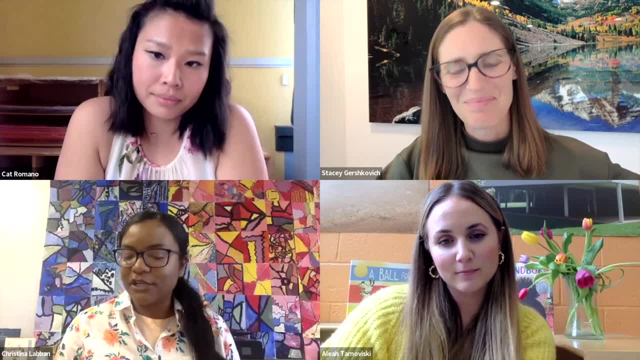 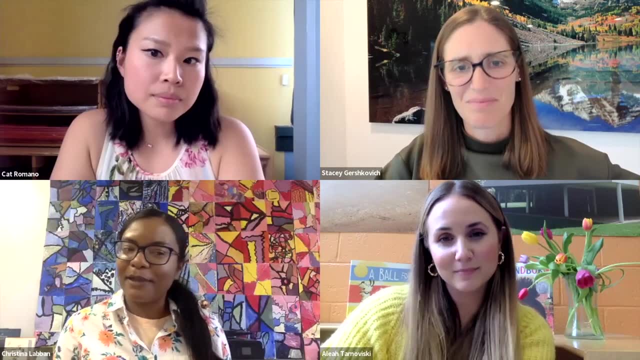 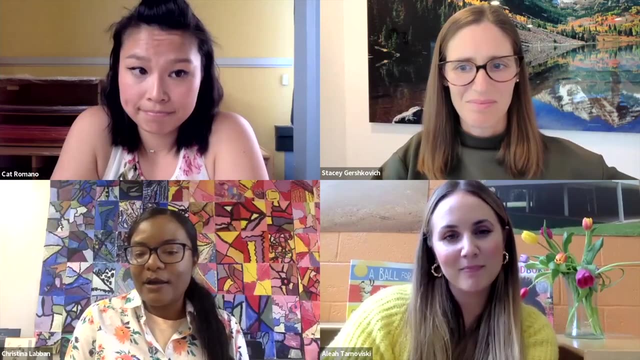 that you understand, but then also just try to get details about what happened and not try to interject what you think happened, but what actually happened. so letting them talk first so that they can tap you to get your attention. so it's good to just listen to them. 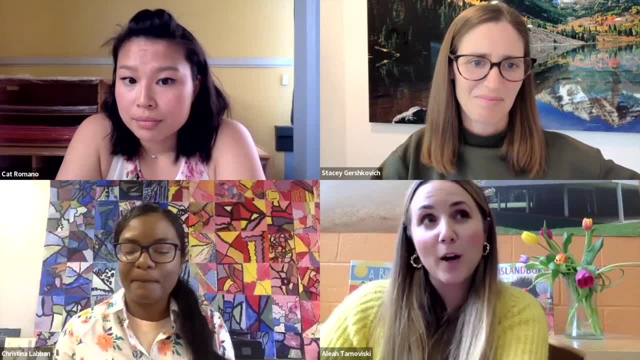 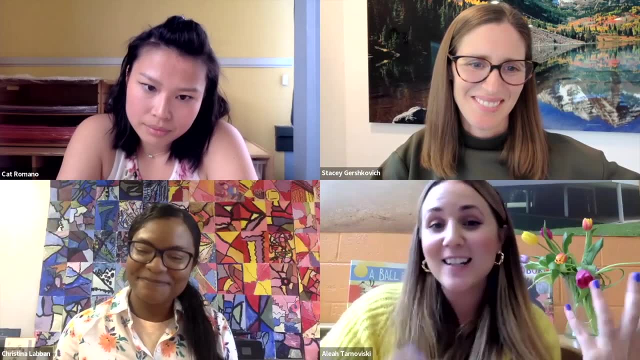 but also just to validate their feelings. yeah, I know we talk about a lot like we're in New York City and so a lot of kindergarten at the beginning is like oh my goodness, they bumped when they were walking to the closet and I'm like there's 25 of you. 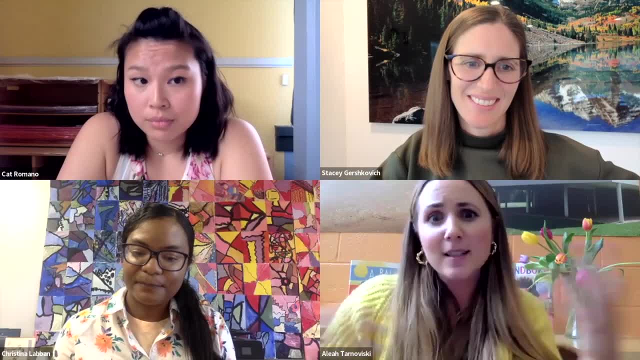 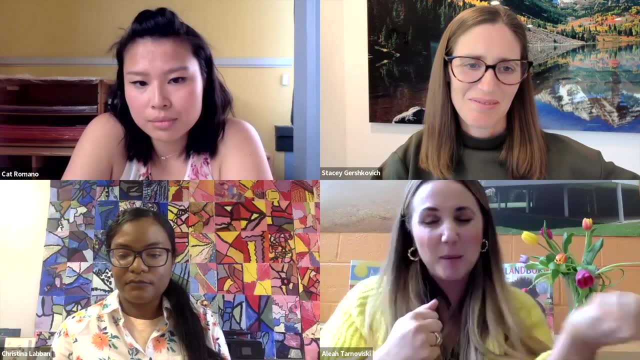 and we're in a small room and so we talk about- like you can talk about it if you're in New York and it's so packed and we might feel other people touching us as they're getting on, but they're not doing it in a mean way. 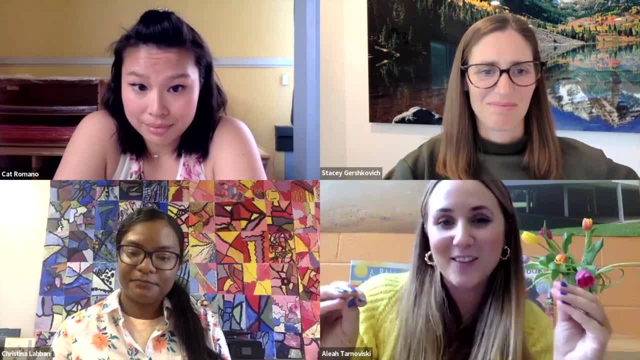 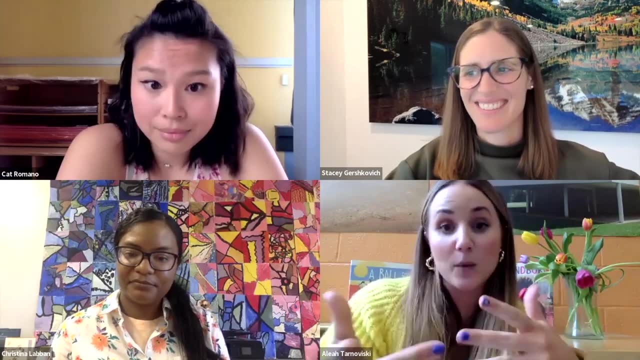 sometimes it's just the way that life is going at that moment. obviously, I don't want your child to feel like they're on a crowded subway when they're in our room, but I think a lot of those times- like Christina was saying earlier, about speaking up when you need something- 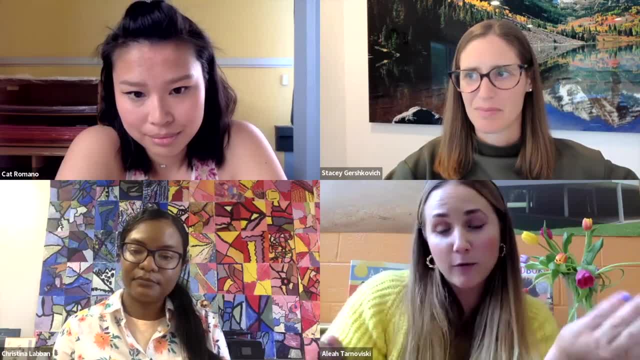 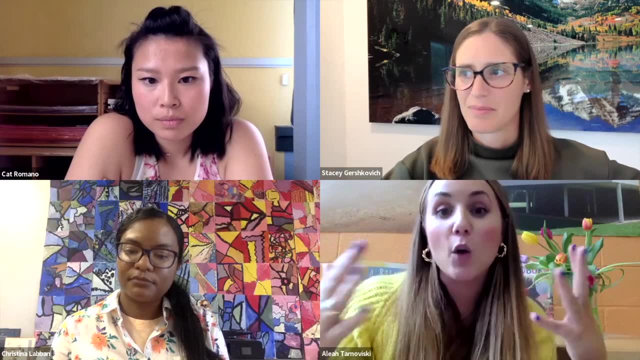 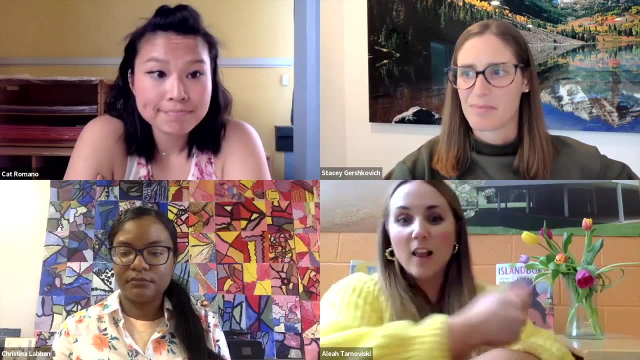 and preparing them like you might have interactions with other kids, that you're meeting in a space with other kids like that and just encouraging them to speak up. because I think those teachable moments of how do we walk safely to the closet to make sure, how do I carry my backpack back to my seat- 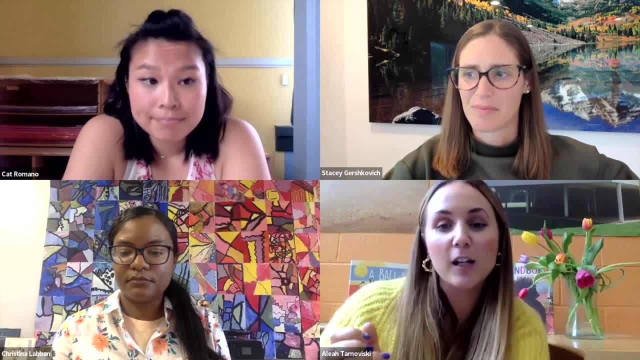 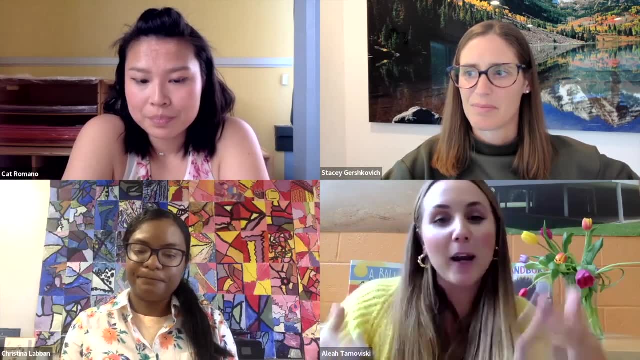 so that it's not like swinging and maybe accidentally hitting my friend as they're walking to their chair. a child speaking up in that moment is a really awesome teachable moment and, as a parent, you obviously can always reach out to us- phone, email, whatever your school. 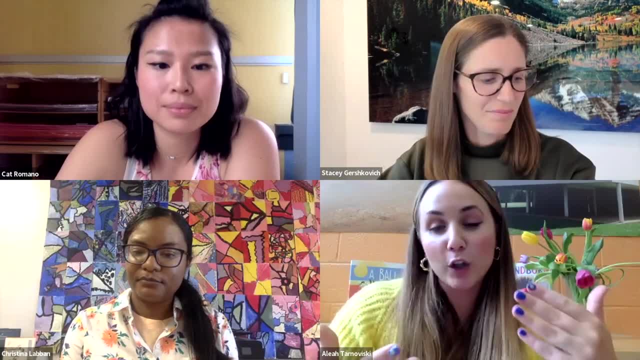 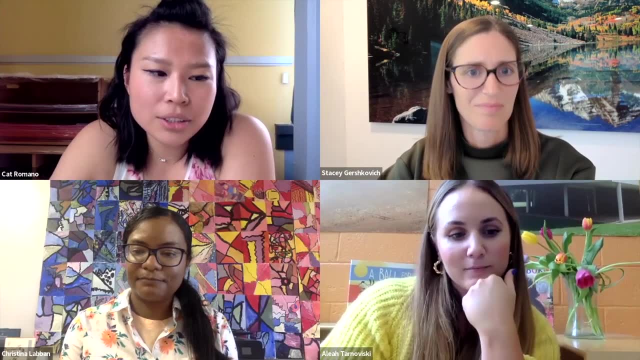 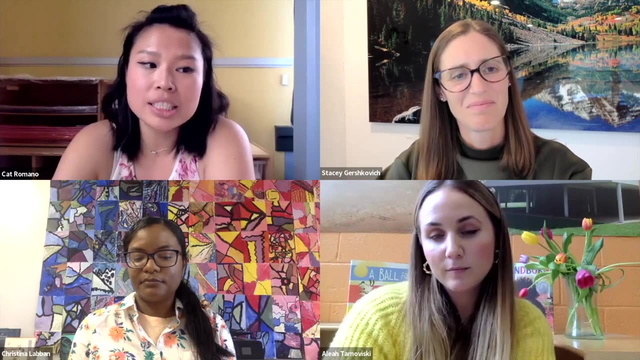 goes by. but I think also encouraging kids to speak up in the moment creates that opportunity for the community to grow in that moment. and then also what we have is a small socio-emotional curriculum which does give us different types of scenarios, because I think often when kids especially 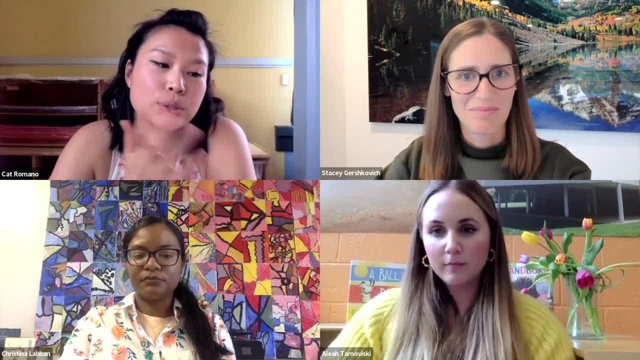 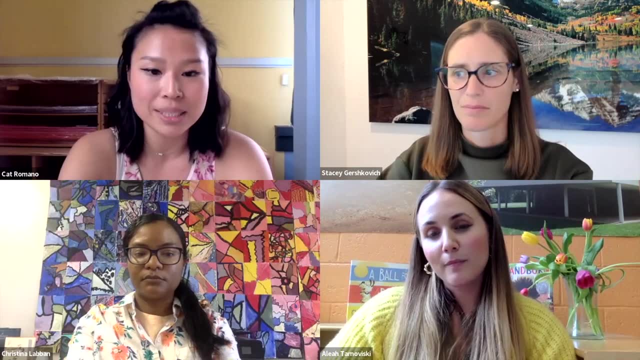 come in the beginning of the year, they're not really sure between the difference of an accident and someone purposely trying to be mean in a way that makes you upset, and so often times when I've talked to kids in the beginning of the year, one scholar is saying: 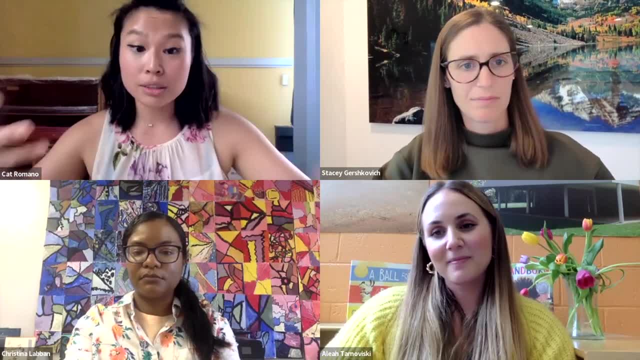 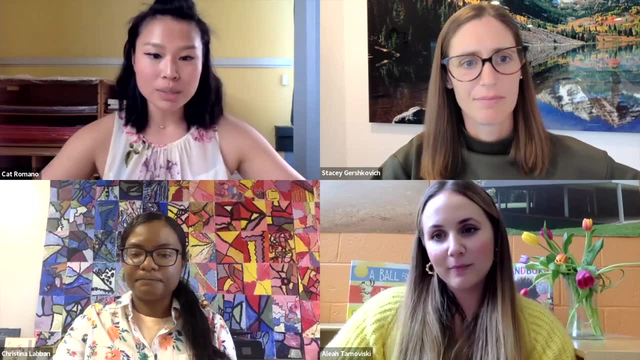 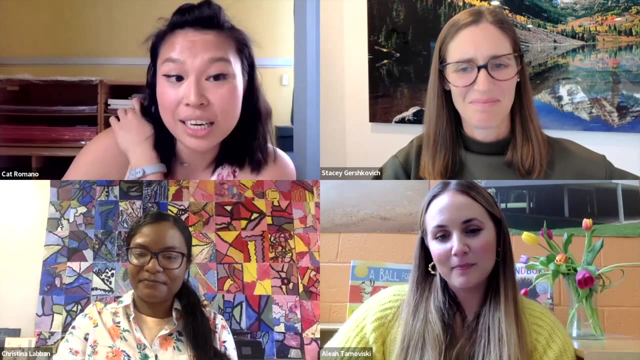 she bumped me like this and then it turns out she was just walking to her backpack and they were both walking and they just shoulder bumped and didn't know how to react in that way of humans bumping into humans, little humans. so we do go over a lot of different. 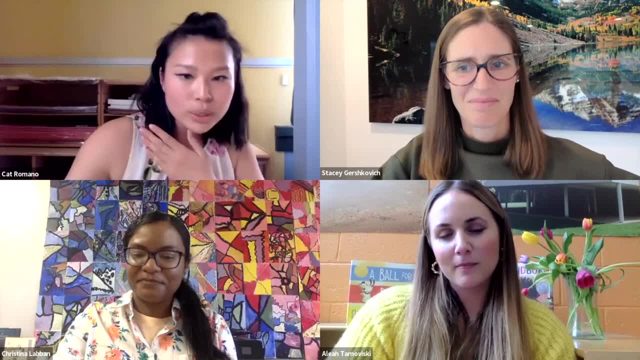 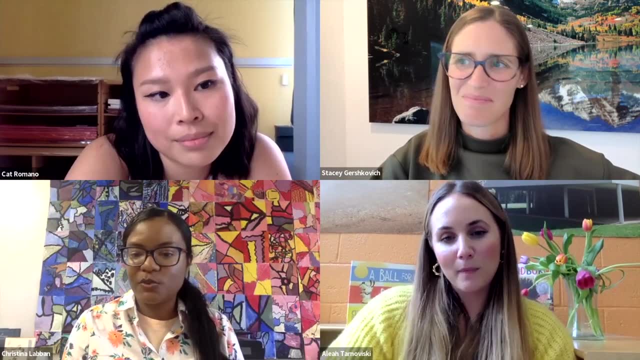 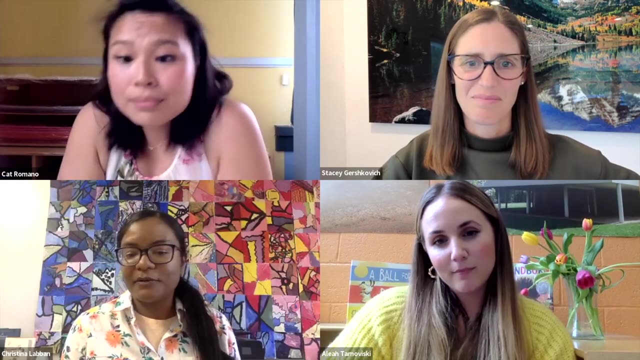 role play scenarios and talk about what can we do. do we get upset? how do we react? yes, we also do that in my classroom as well, where we're catered towards talking about our feelings or talking about how we deal with friends when maybe they've bumped into us. 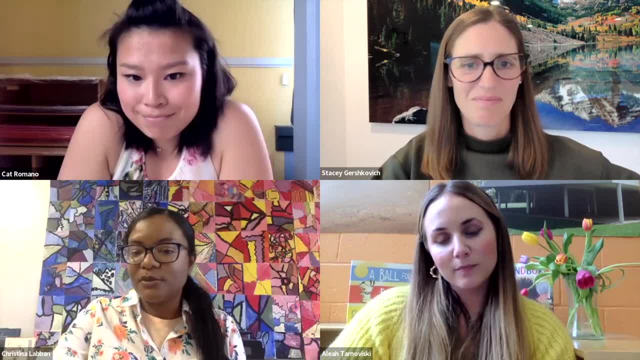 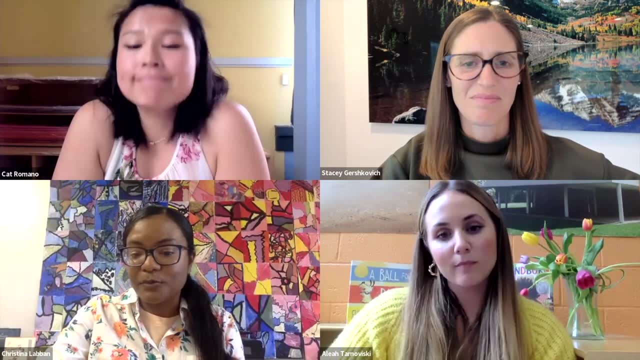 or when should we say sorry, things like that, so they do get the chance to role play, as Kat was saying, and also just hear about read alouds. that will help them learn more about those social skills. yeah, I think those are good points. the more we can talk to our student. 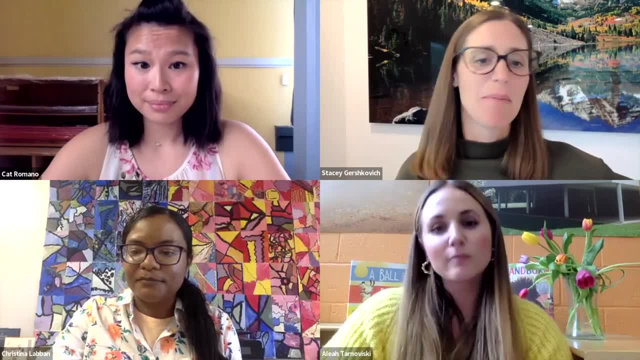 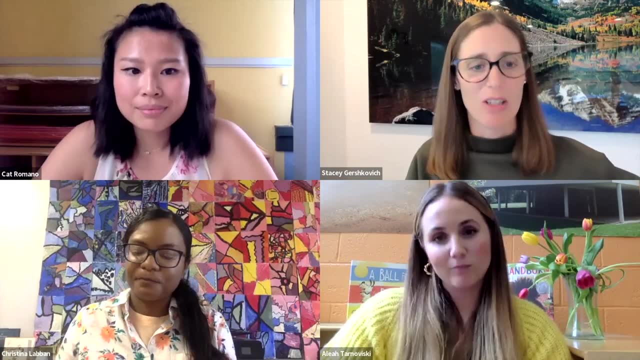 about what happened and talk about how they handled it- maybe how they would handle it differently- and then that communication with the teacher is key, right? teachers only know what the child told them. it's possible that the teacher is completely unaware because the child hadn't mentioned it. 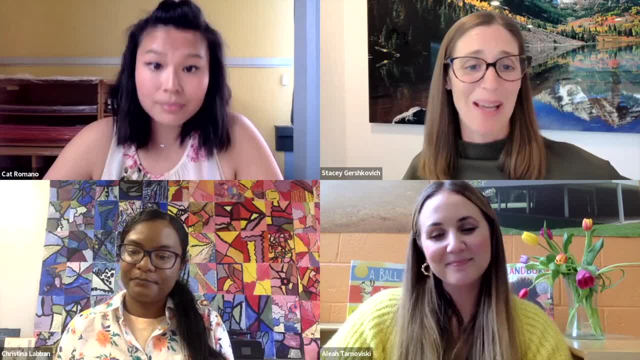 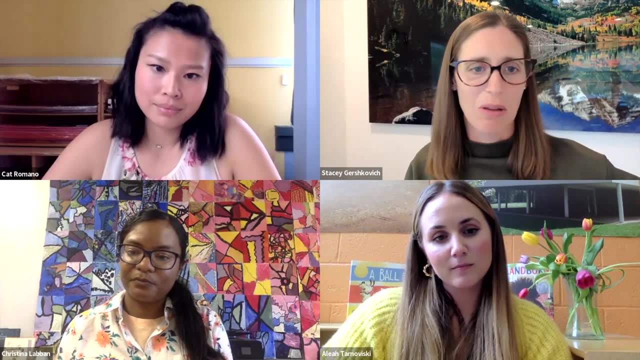 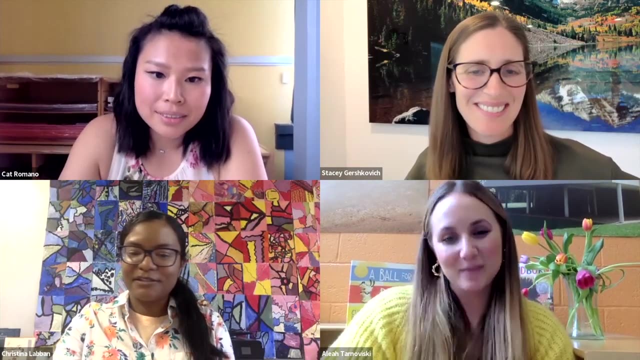 or it's possible that the teacher absolutely knows exactly what happened, because the teacher was there and spoke to the child. but the more you communicate, and what is the best way to communicate with you guys? I assume parents can call you, they can email you. yes, parents call. they leave voicemails. 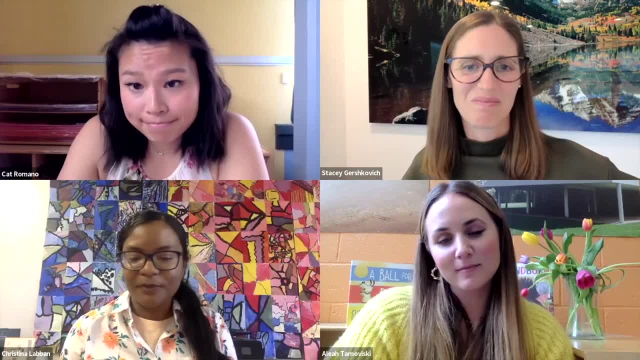 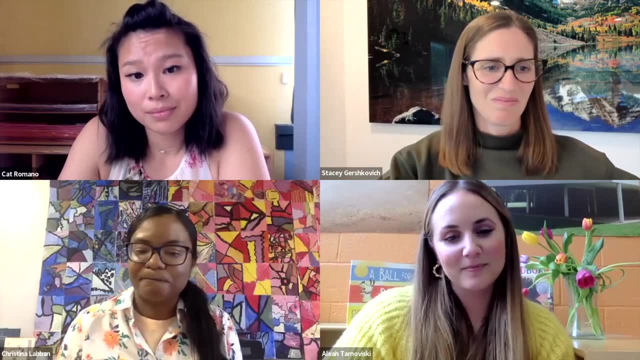 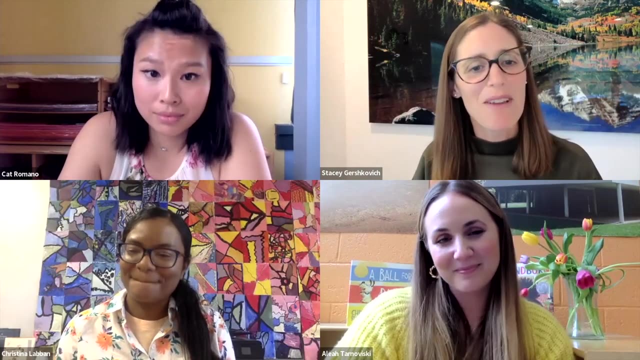 they text, sometimes email. we're available through various methods or just even at dismissal. they'll talk to us too. and then we have the very often question lunch and recess. as we saw from the video, it is our student's favorite part of the day. do they have enough time? 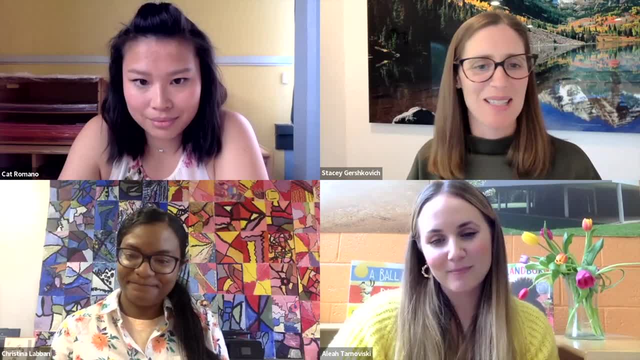 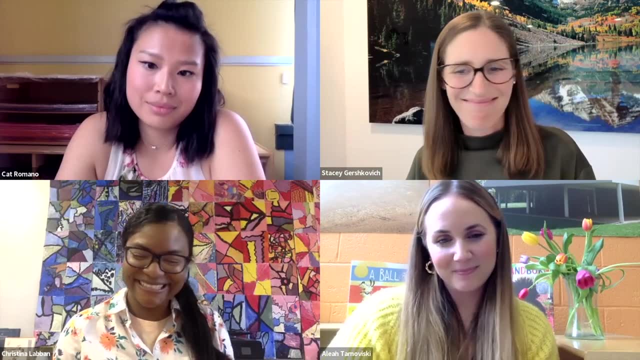 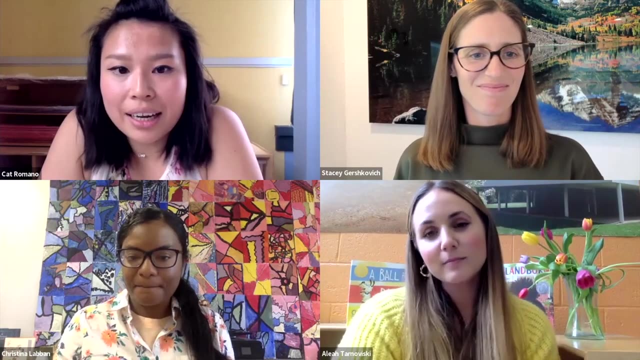 for lunch and recess. what happens at lunch and recess? talk to us a little bit about that part of the day because I know- at least my kids- their favorite part of the day. at our school we have a cafeteria. lunch is about 30 minutes and scholars sometimes bring their lunches. 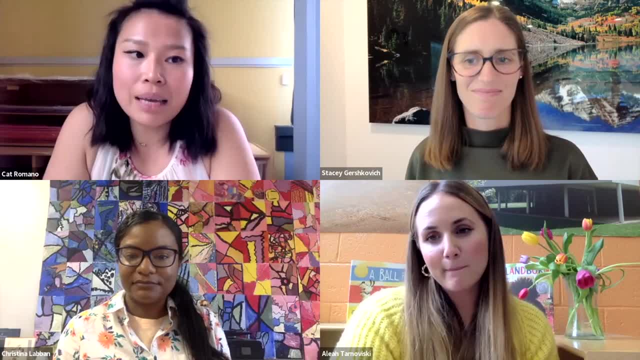 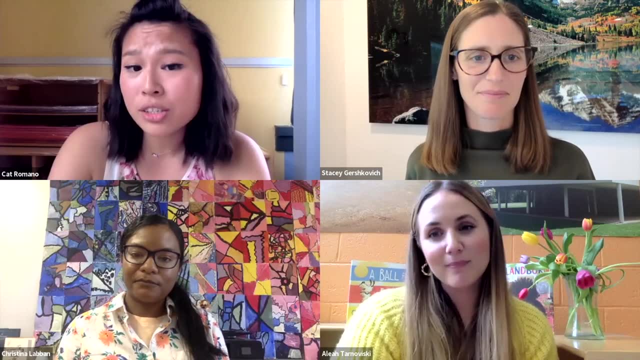 from home with their lunch box or they come get a school lunch. everyone gets to pick where they sit at our assigned table. they eat, they talk. they talk about their favorite TV shows, they share about their snacks. sometimes they get really excited because they have the same lunch. 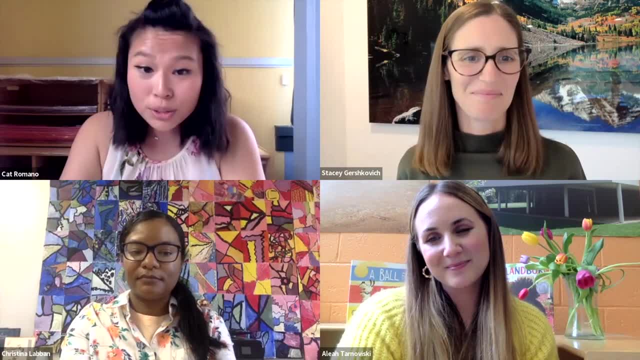 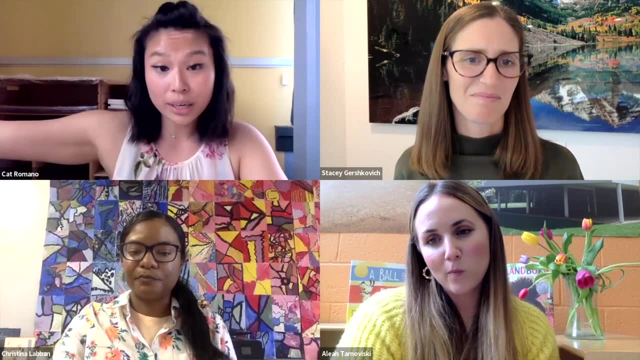 they both have lunchables. they're like: whoa, you have lunchables, me too. after lunch we'll clean up, and then at least in our school our recess yard is right outside, so we just exit the cafeteria, we go outside to the recess yard. 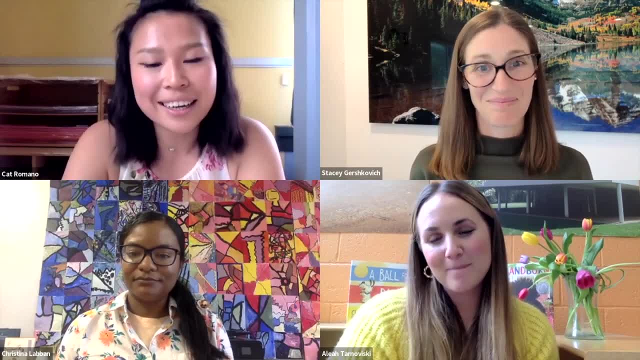 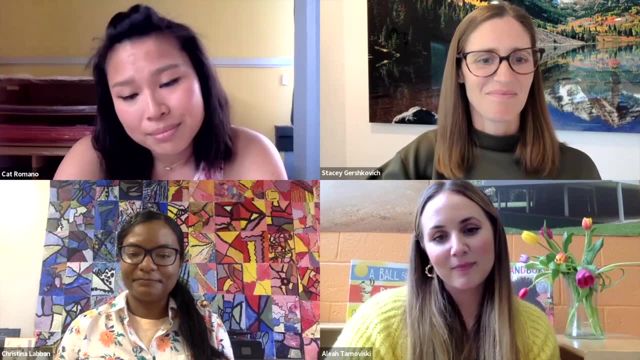 it's currently under construction here, because they're building a playground, which is very exciting, and they get to play for about 25 minutes and then we line up and we go back upstairs. I also will say I know at our school we do play throughout the day. 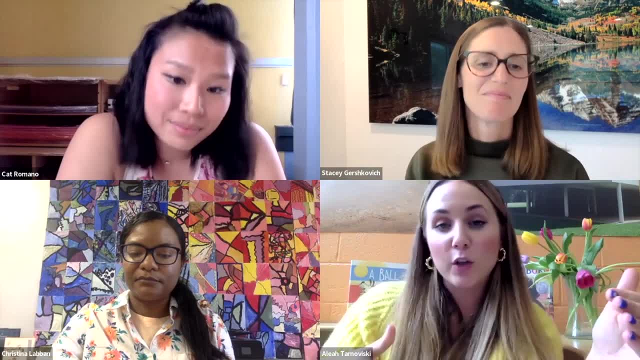 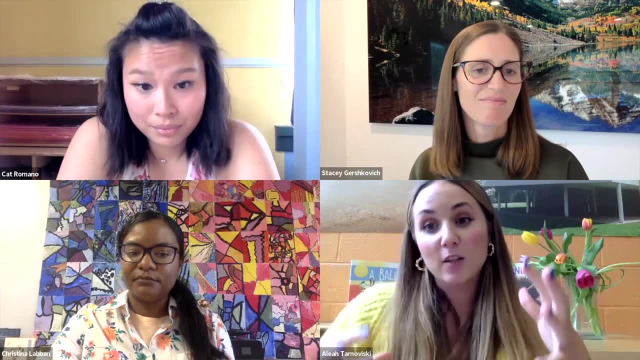 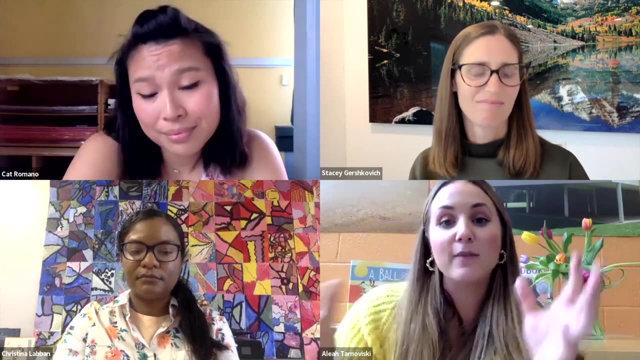 so their moment to play is not just at recess, there's also. we have blocks, we have different center games like dramatic play, so there is almost an hour block in our time at success where they get to play, and I know that's similar across many kindergartens. 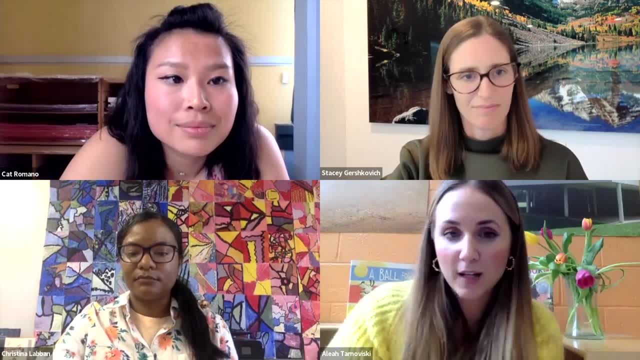 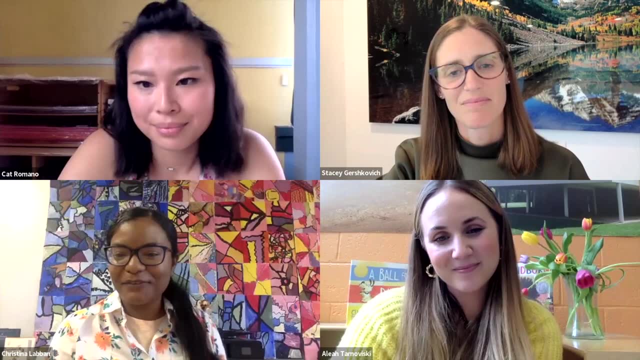 where they're going to have time to play within their classroom or a playroom, and then they'll also have recess, and then, additionally to that, they also have snack time, which is an opportunity for them to just relax, to chat with their peers, and they enjoy that time as well. 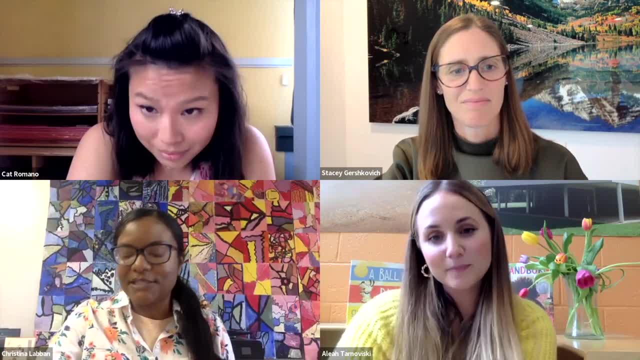 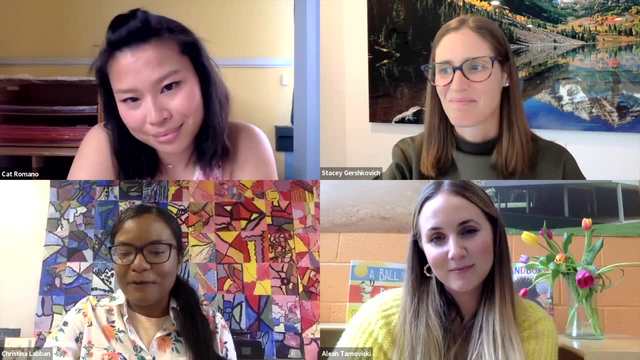 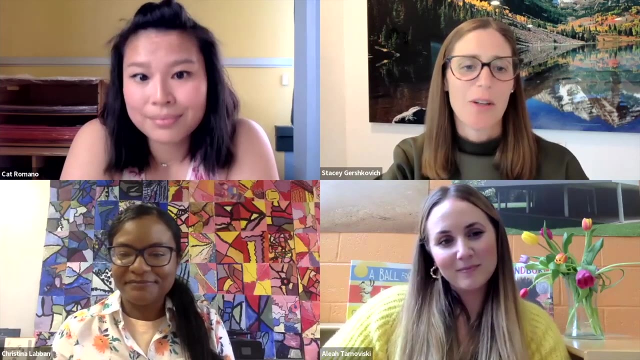 and then in my school we also have specials, so they get to go to dance, they have sports. they love those teachers too. they get to have science, so they really love going to those specials as well. Yes, and I can speak as a former teacher principal: 30 minutes, 25 minutes is more than enough. 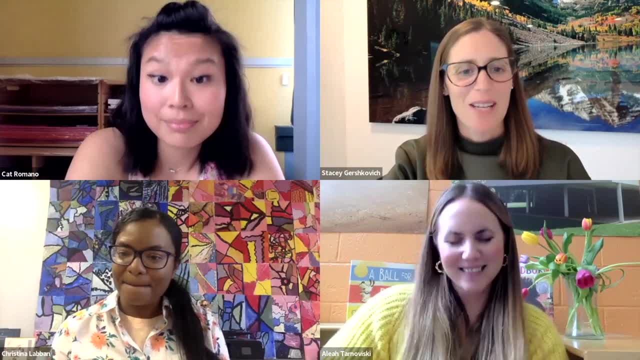 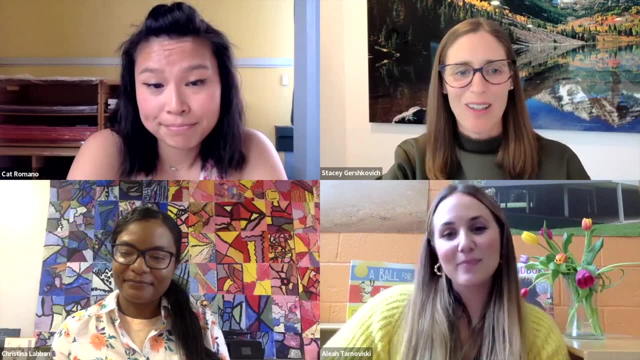 for children to eat lunch. they usually eat their lunch in about 5 or 10 minutes and then spend most of the time talking, but the staff that are in the cafeteria will make sure that kids are eating and tell them you have a couple minutes left. now is the time to stop talking and start eating. 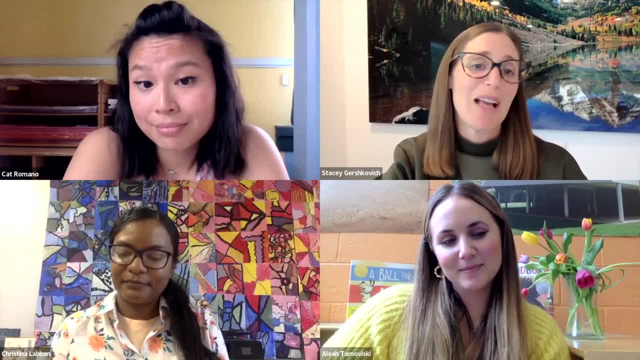 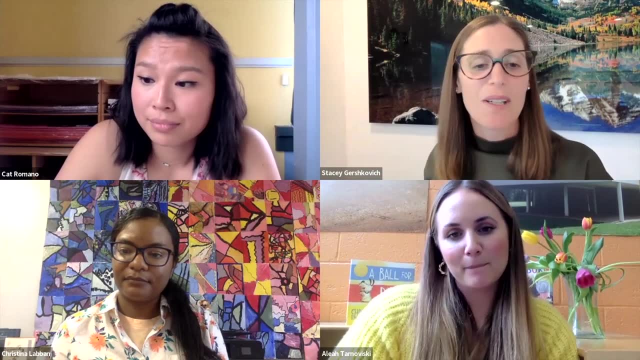 because I want you to make sure you finish your lunch. but if you come home and you find out that your child isn't eating lunch, or they say they're not eating lunch, or your lunch box that you send is coming home full, that is absolutely an important thing to tell the teacher. 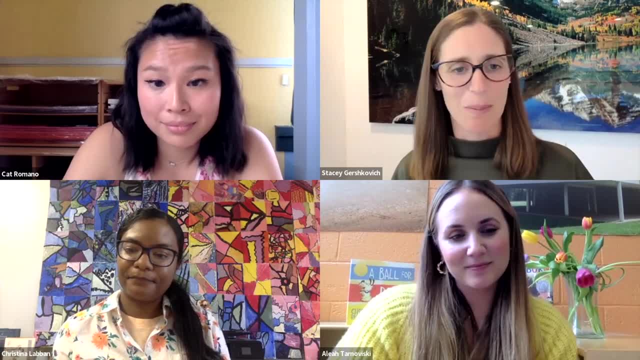 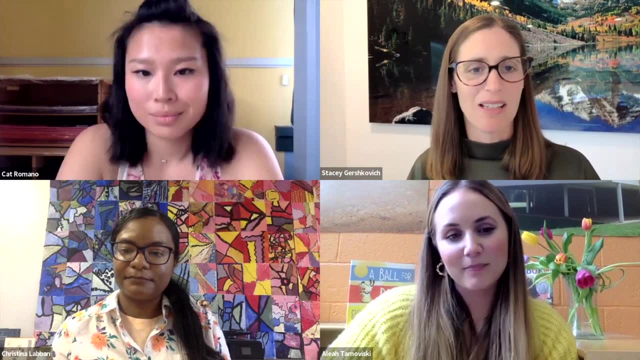 and we will be aware of that. but that is not my experience. my experience is that kids do have plenty of time to eat and then they do have obviously plenty of time to play, both at recess but also in the other parts of the day. and Stacy, I'll say 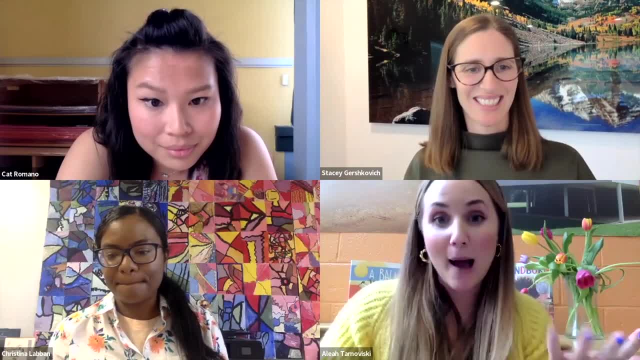 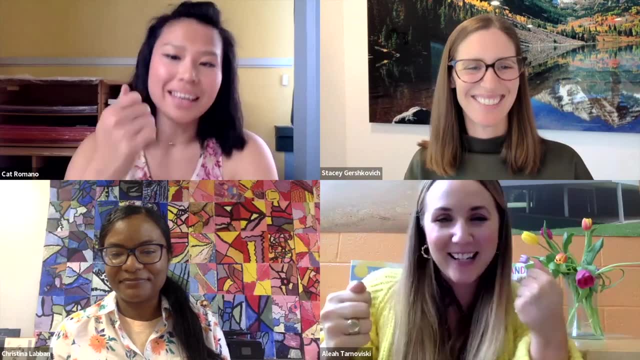 another thing that you can kind of like rehearse and practice at home is like if you are packing a lunch, talking about like showing them what's in the lunch and talking to them about the order, you want them to eat their things because you know if there's Oreos in there. 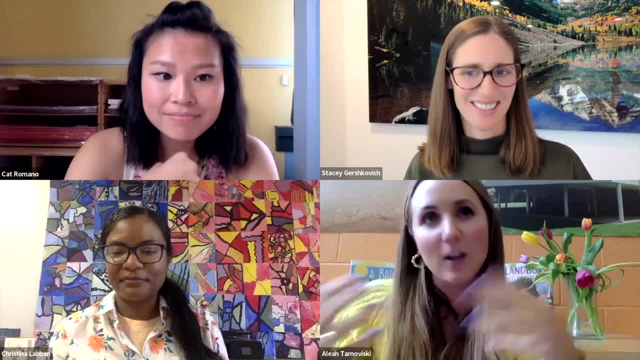 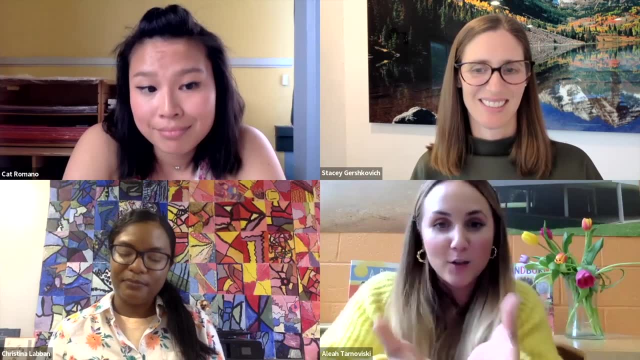 that is the first thing I'm seeing being broken open as soon as lunch begins. of course, if I see it, I'm like: okay, let's eat our sandwich first, let's eat our carrots, right. so talking to them even just about like: okay, these are all the things that are in your lunch. 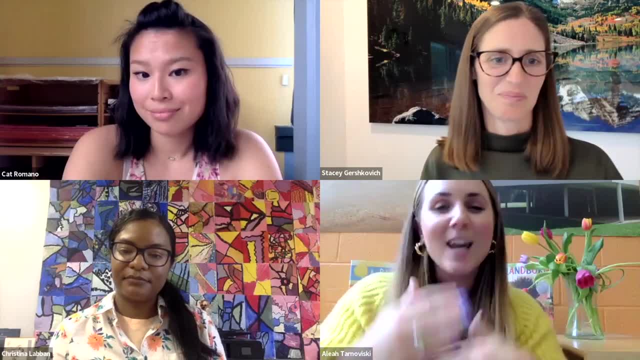 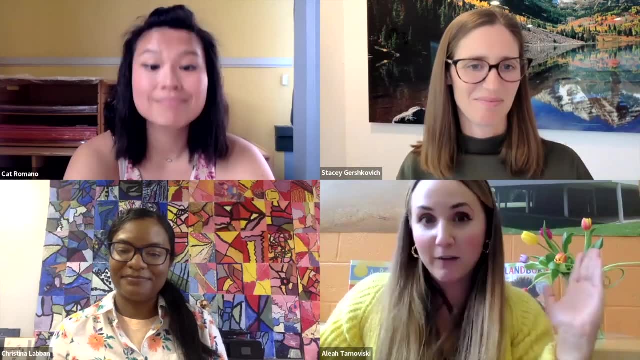 like: let's eat your carrots for snack today and let's eat. make sure you eat half of your sandwich before you open your cookies, just talking them through, like that's the first time they're really just like on their own to eat and kids will just feast on whatever. 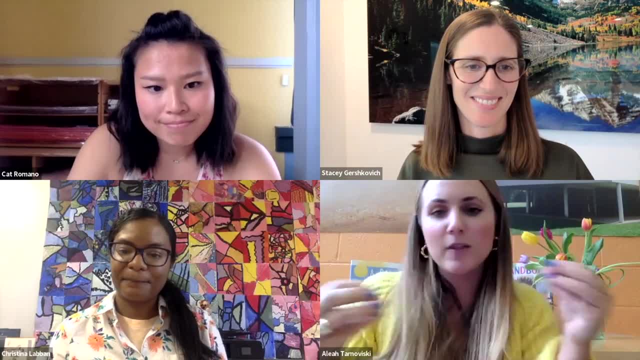 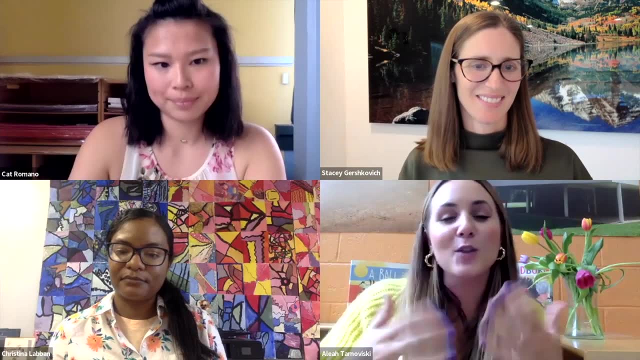 like fun things are there and so we talk a lot about like we want to make sure we're eating our like sandwich or rice and beans, whatever they have packed for the day. we can enjoy our treat after that's done. so, yeah, talking them through that, I think. 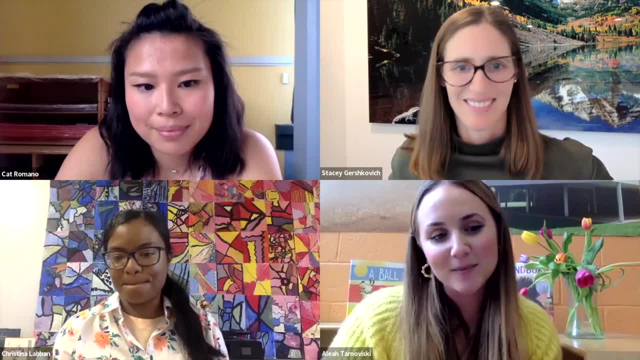 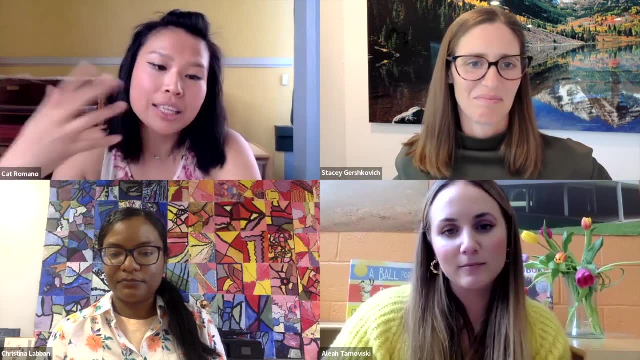 is another good thing to practice before school begins and then to answer some questions in the chat. yes, we are always there with them at lunch time. the only time we're not is when they go to their specials teachers, but every part of the day at least one, if not two. 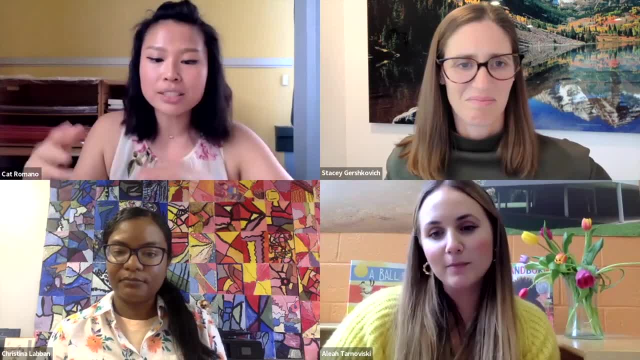 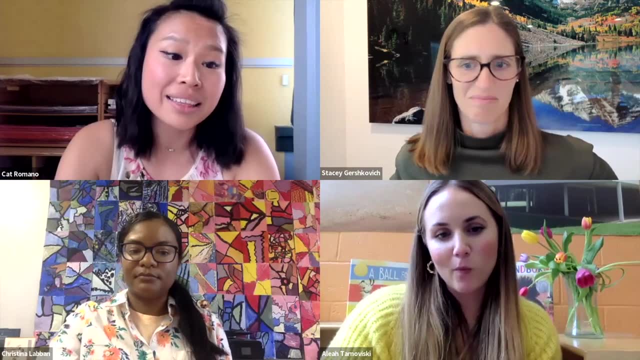 teachers are there at lunch and we are just kind of like moving around to make sure that whatever's in the lunch box or whatever's on the school tray has at least three big bites before we put things away and then in my classroom, if someone tells me. 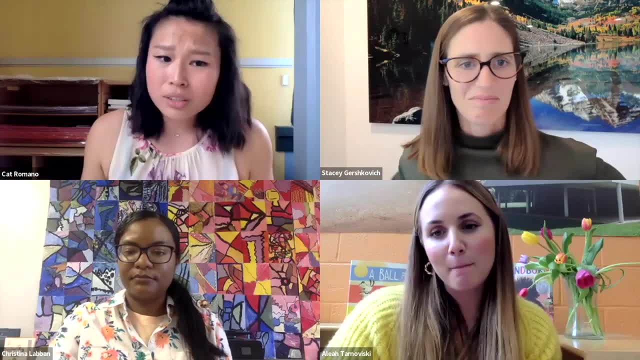 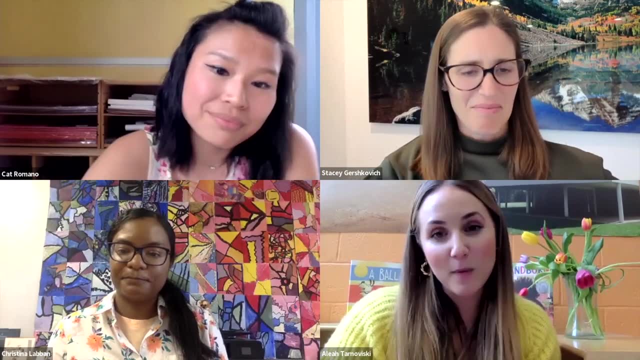 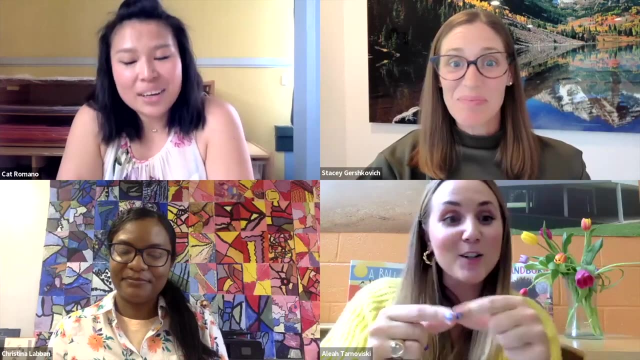 they're hungry. later on during play times, I tell them: go get your lunch box. you can sit at your seat and finish your sandwich if you're still hungry. I'm still thinking about things that are popping up because Kat just reminded me, like practice opening snacks at your house. pinch and pull. 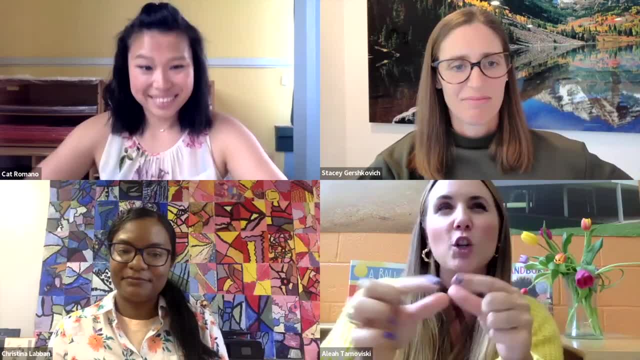 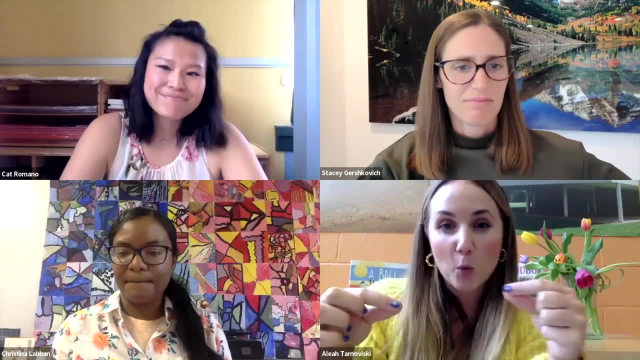 like a little bag of Cheez-Its or a little bag of fruit snacks. like you can practice that. I know we give snacks that are like pre-portioned, like that, so they're getting Cheez-Its or Goldfish. like practicing opening bags if you're sending. 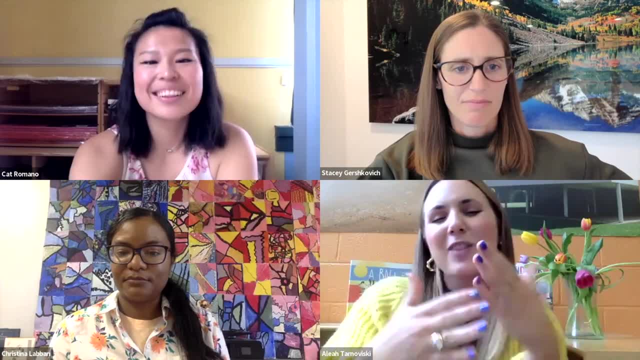 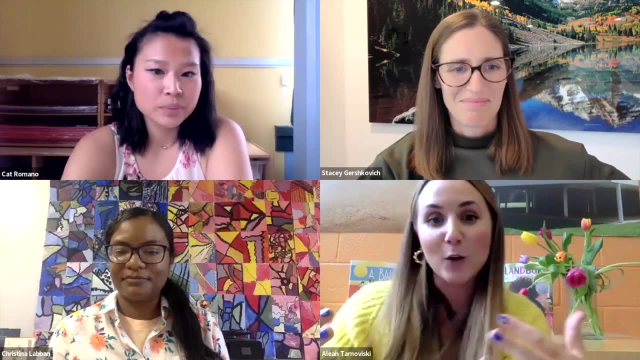 them to school with lunch, like practicing opening a Ziploc, like they don't need to be experts at it. but I think on those first days of kindergarten where it's like 25 kids all have their hand raised because they can't open their Goldfish, like we do a lot of. 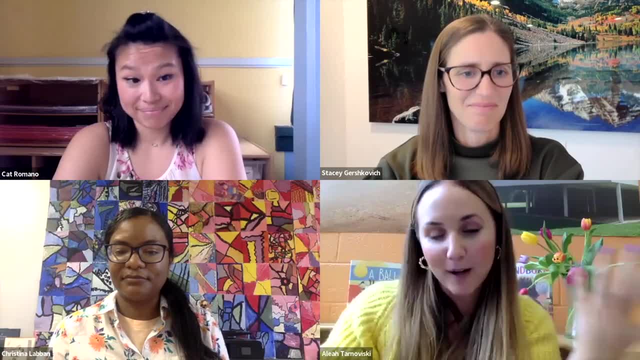 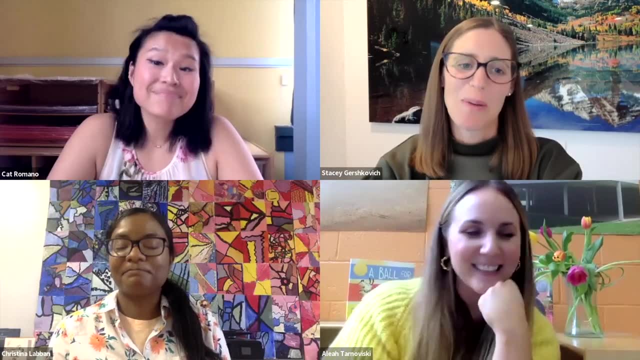 practicing. but practicing that at home is really going to prepare them for those moments as well and make them more independent so they can enjoy their food. and then they can help a friend, and that is always feels really good when I can help my friend open their Goldfish. 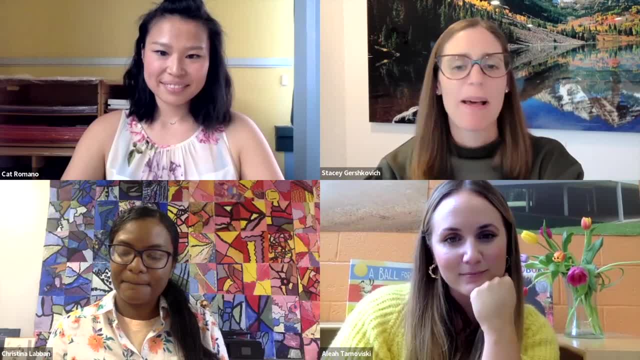 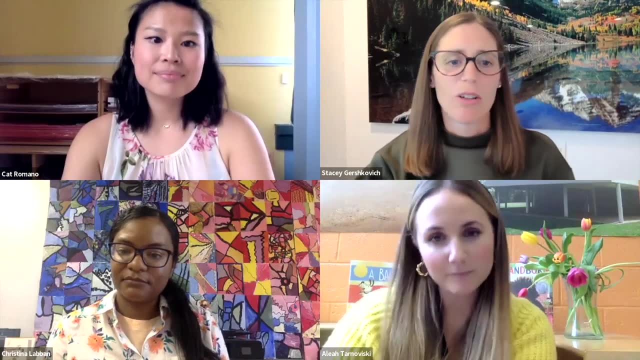 so there's a lot of questions coming in. we spoke about it a little bit, but I want to go back to this topic. some of our students are coming in and English is not their first language. they're learning English for the first time. some of our students maybe have 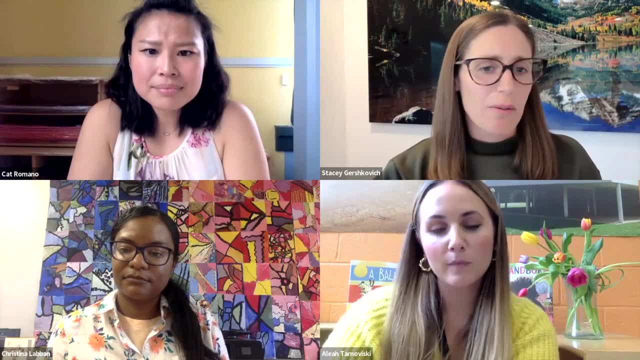 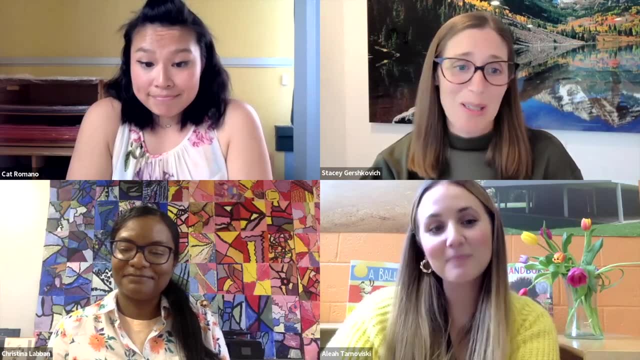 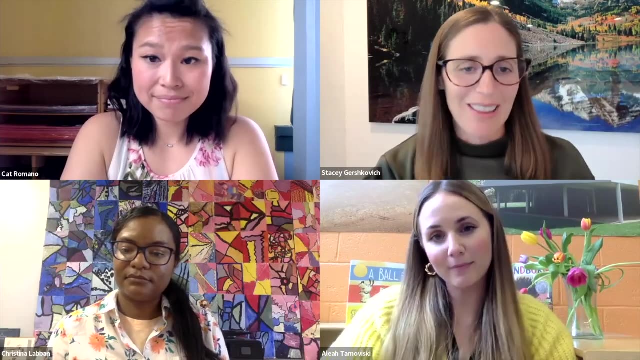 speech delays. some of our students are behind for other reasons. some of our students maybe are those December birthdays right and they're still four years old for quite a long time when they're starting kindergarten. all of these you know, and more right because they're not all of the things that maybe parents 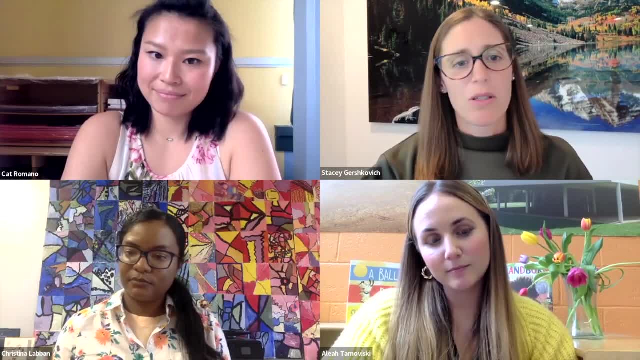 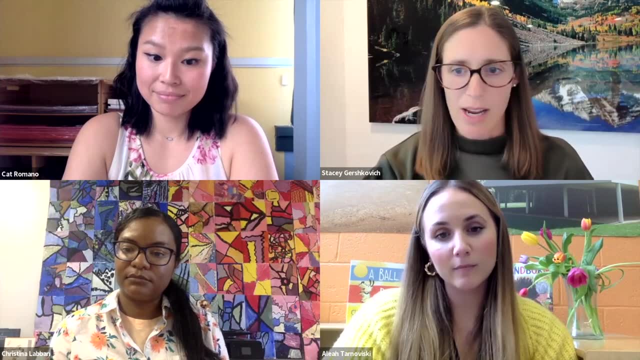 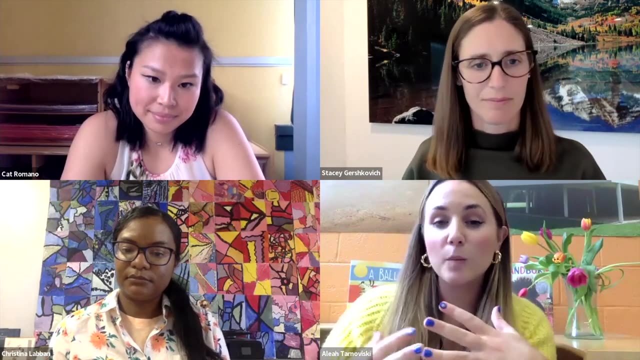 are worried about. what are we doing for those students? what is your experience and what should parents be thinking about or doing to help support their child? I will speak a bit. I teach. I'm a special education teacher, so my kindergarten classroom in New York we call it an ICT classroom. 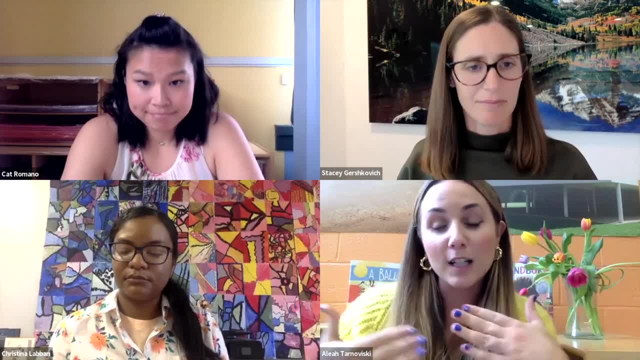 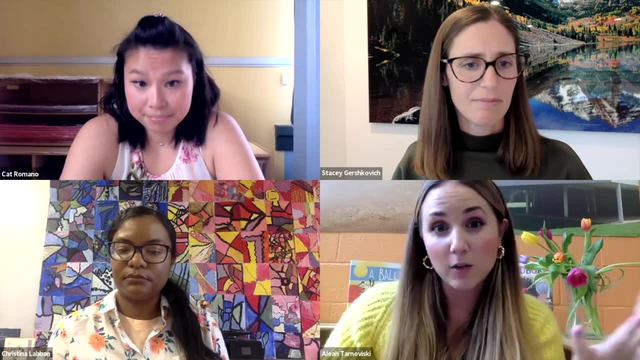 so it's myself and a general education teacher and we co-teach in a classroom, so I have some scholars who have come in with IEPs, and some of those IEPs are about speech. most of my scholars are working through speech delays and so, again, 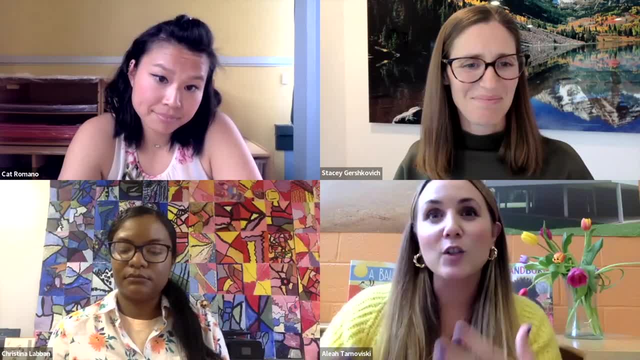 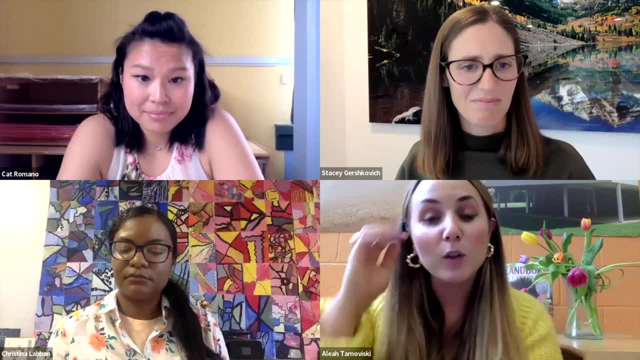 I think feel confident and at peace and at ease that your scholar is being placed in the right setting, with teachers that are knowledgeable about the things that they're going to be working on, and what's awesome is their speech provider. I'll just use speech as my. 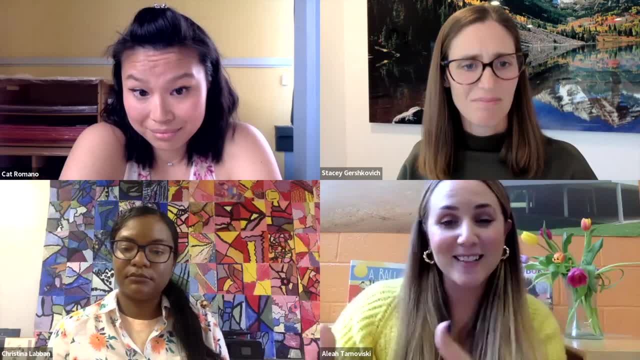 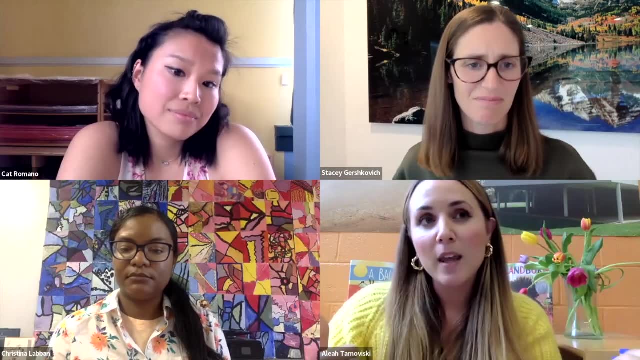 example. I talk to her almost every day, so our speech provider, her name, is Miss Amanda, and so I'm meeting with Miss Amanda, and Miss Amanda is working on things that we're doing in the classroom, and we're a team in the same way that your family. 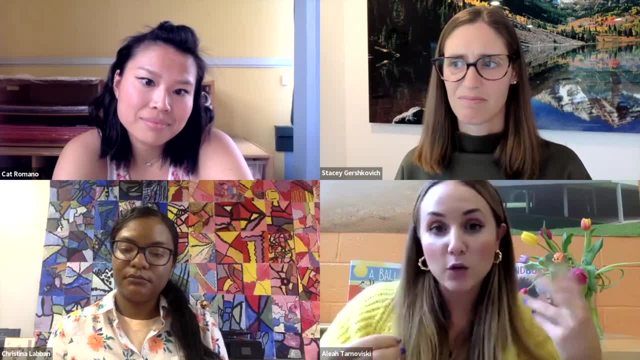 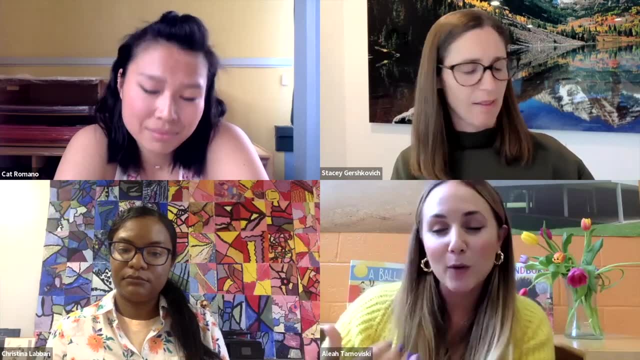 and myself. we're a team as well, and so I think that dialogue is really important, and your child's teacher will be familiar with what they're working on, will have read through their IEP before they come into the room. but be at ease that we know. 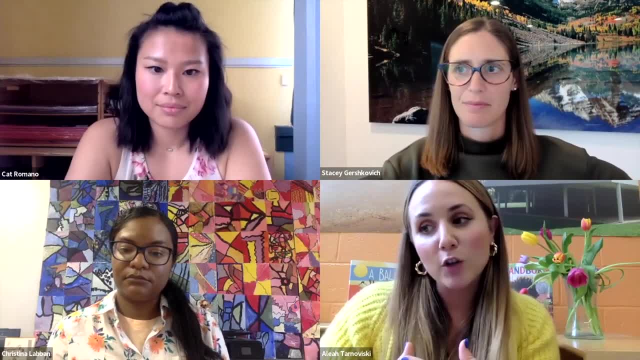 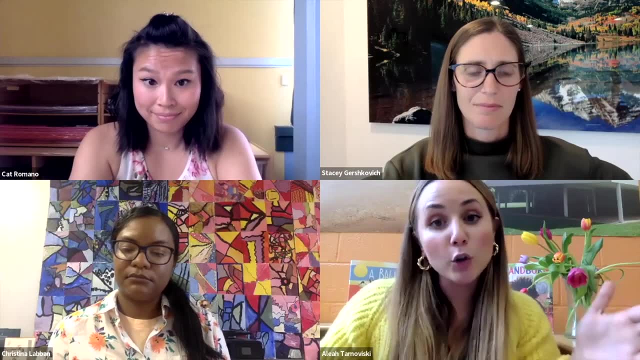 like kind of what to do, and we also are planning. every time I plan a lesson, I'm thinking about your child. I'm thinking about how to support them when I'm teaching whole group, but also when I might be working one-on-one with them or in a small group. so it's a part. 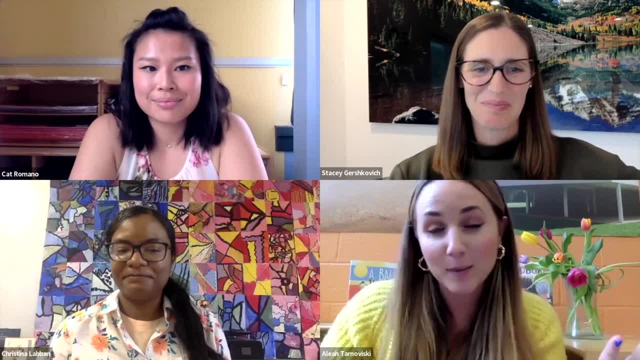 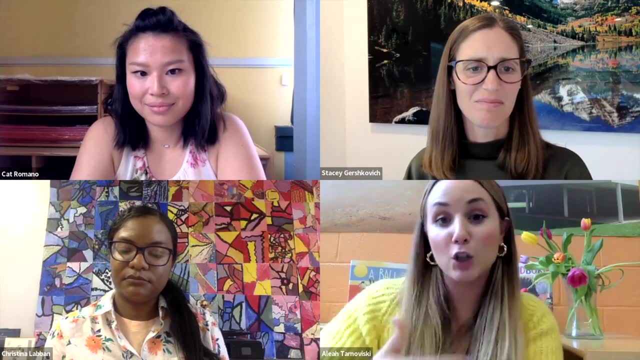 of my planning and I know I see everyone nodding. I know that's a part of all of our planning. it's very similar to kids who we know are coming in learning English. we're thinking about them as we're planning and we're making it a. 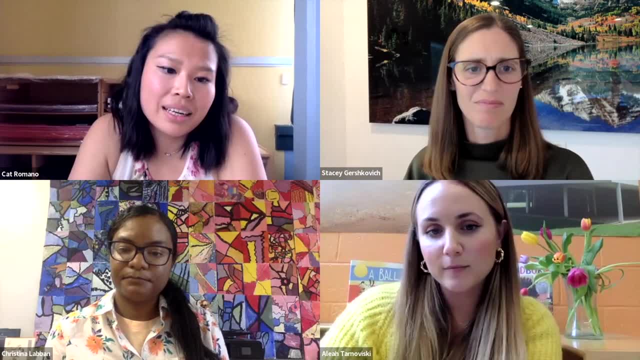 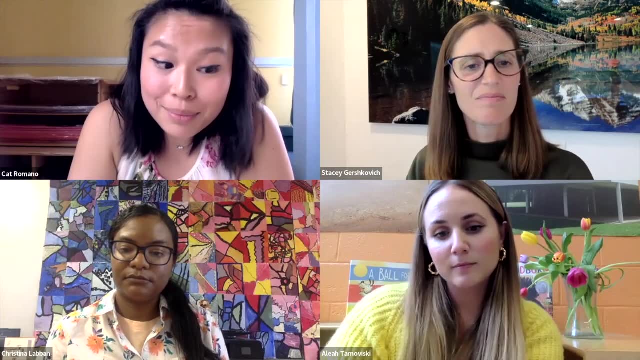 part of how we're changing instruction day to day. for scholars who are younger, coming in turning five in December, and my experience of working with four-year-olds I have. every four-year-old I've met has been the most excited about learning every single thing in the 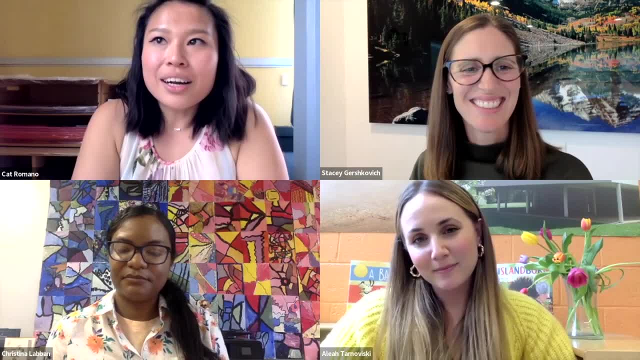 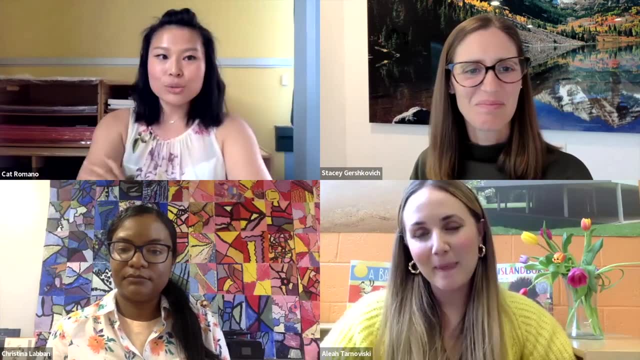 classroom is magical and they are just in such a world of like, of utter disbelief, of like they are really in school doing and doing big kid things and they're there to learn and they are, like, probably the most competitive and they just love to be involved with 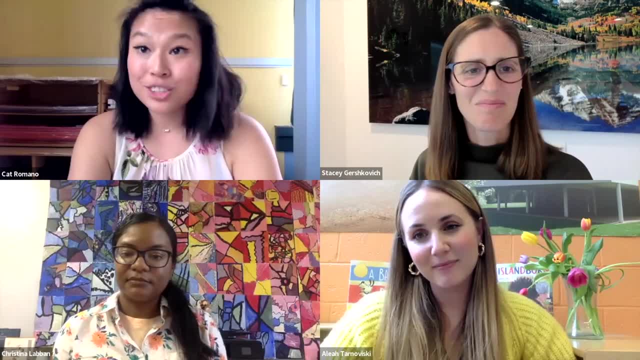 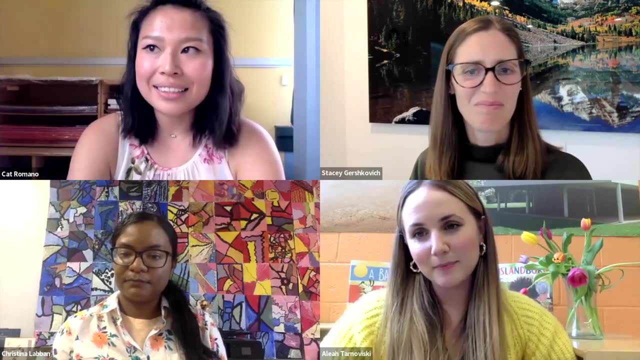 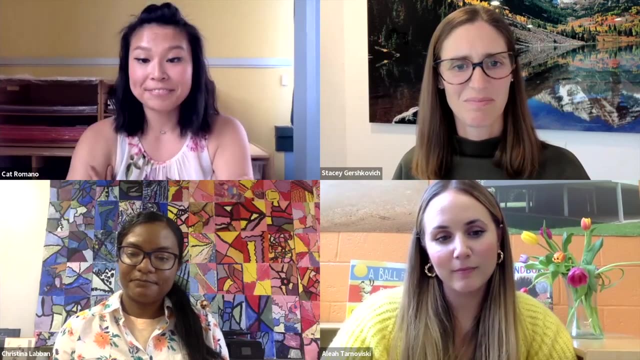 every conversation. so the best way to help your four-year-old is just get them ready there. get them so sure they're already excited, they're ready to just go off on their own and, you know, just be part of a new community. I'll also add for: 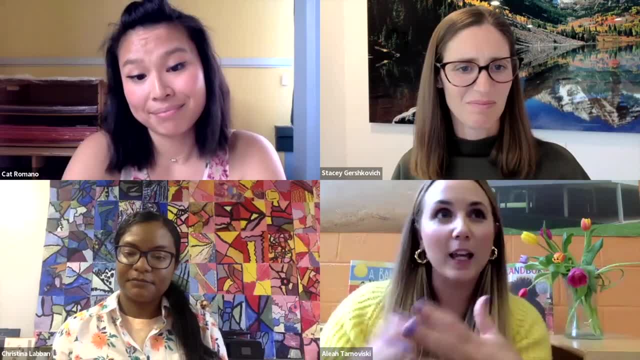 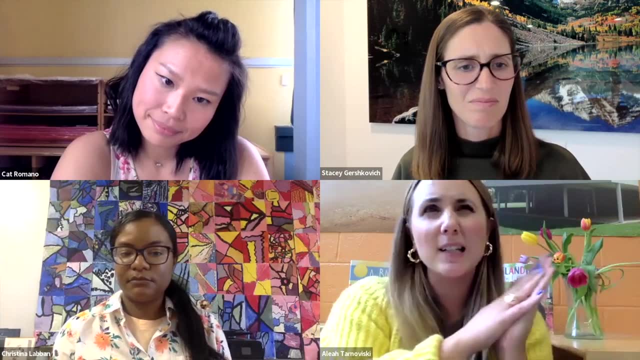 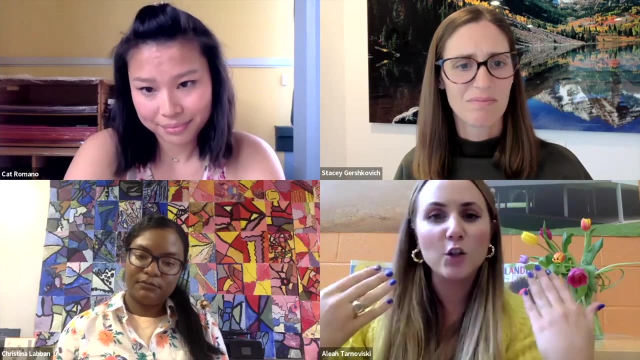 language learners. in addition to like recognizing our letters or counting things, something you can be doing at home is YouTube has, like, so many awesome read-alouds. so like playing read-alouds for them in English or having them listen to books on tape is so old like. 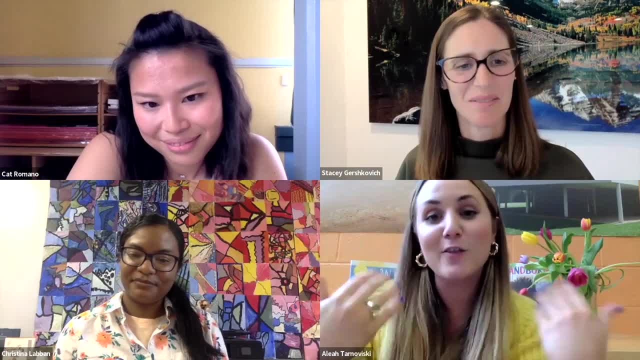 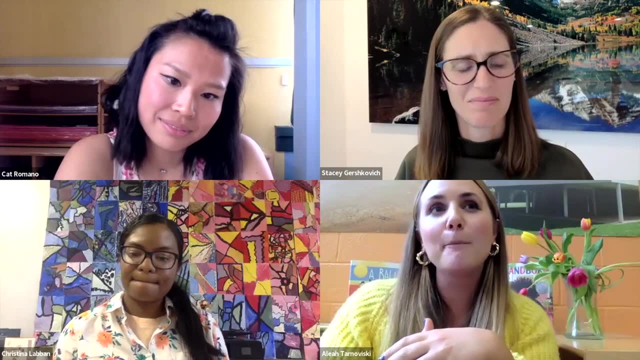 an audible of where they're hearing someone read to them in English. if you, or like a family member, can read to them in English, that's awesome. but just exposing them to the language it's a slow and steady start for them once they start kindergarten, but it's amazing. 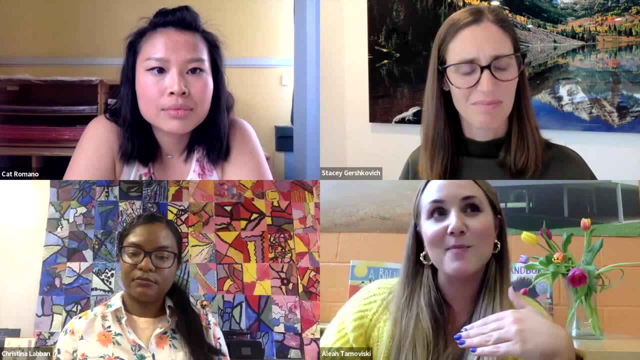 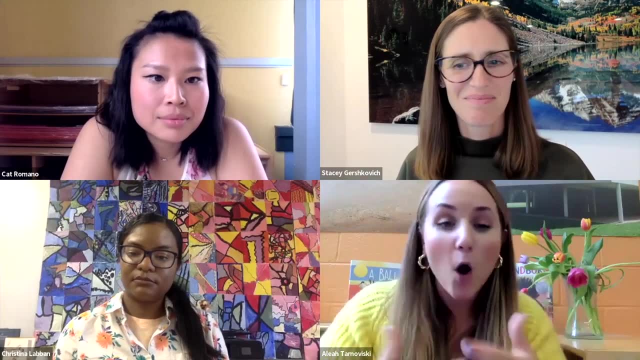 to see how much they grow like. I always tell them the story of my dad always talks about going to kindergarten. he only spoke Portuguese and he was like I was so confused and I And so I always tell that story in the beginning and I go. some of us are going to like. some of us are learning our like different languages. 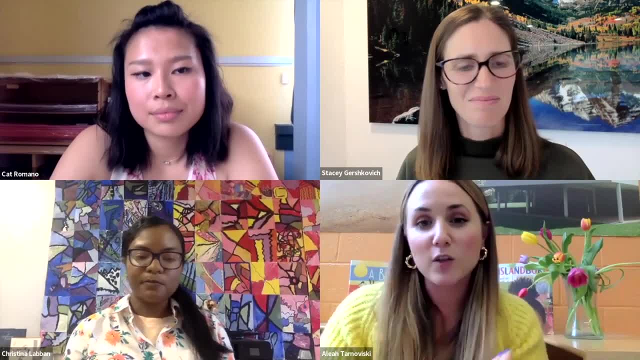 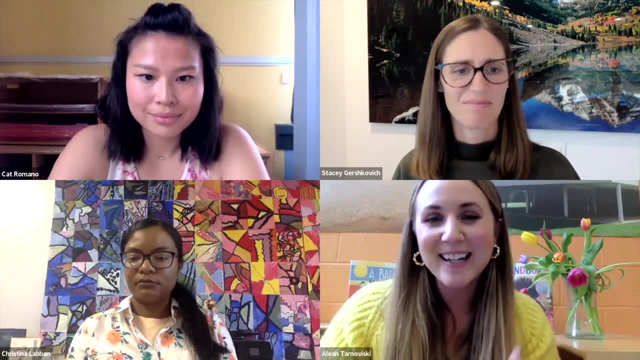 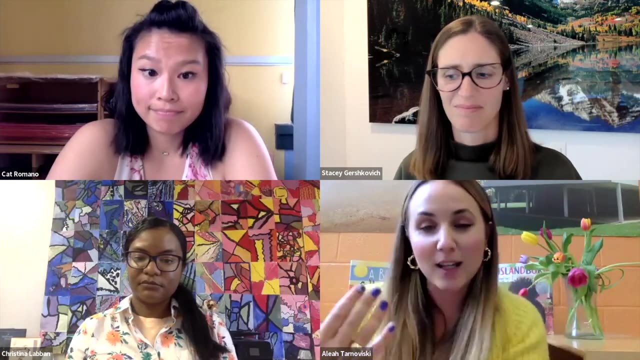 We're coming in. We might speak one language at home, We might be learning one language at school, But it just like enriches our learning community and they will. they will get there. It's going to take time, But the more that they're in that routine, the more they're sitting around their friends and the more they're exposed to that language, it will come. 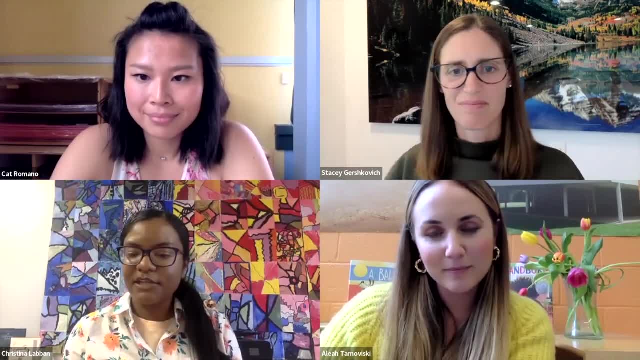 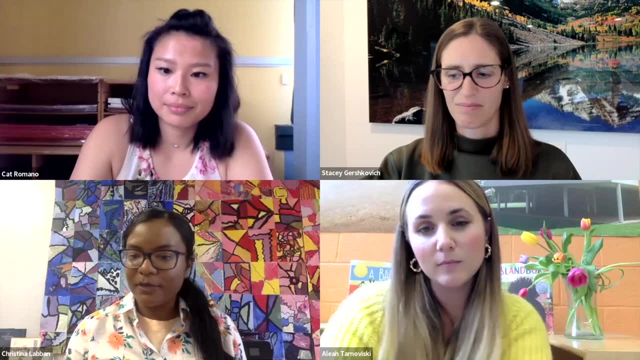 Yeah, And I would also say just keeping that open line of communication with the teacher, because if you feel like your scholar might need help in an area you know your child best, So definitely let us know and we'll do whatever we can to support them at school. 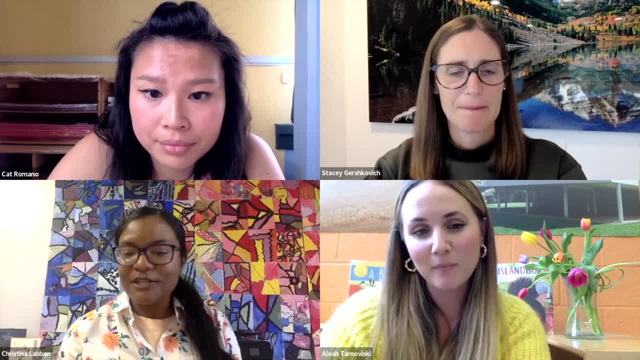 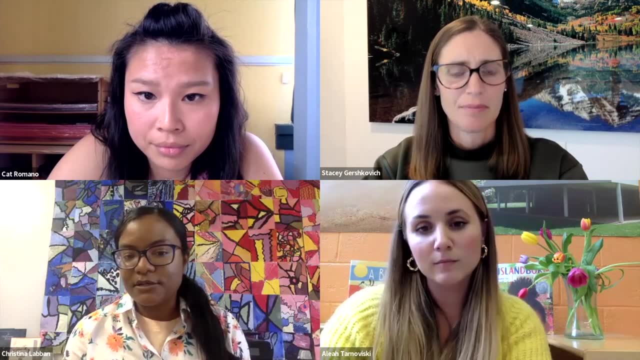 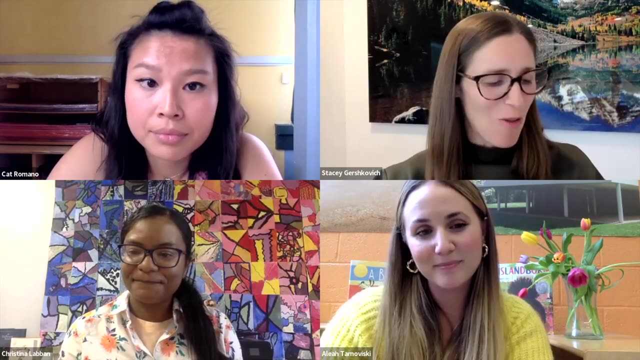 But it's definitely a continued partnership throughout the year. So always reach out to your teacher to see what other supports can I maybe get outside of school or inside of school. We're always here to help you. Yeah, that is always the message, and we want to always go back. So, Christina, thank you for adding that. 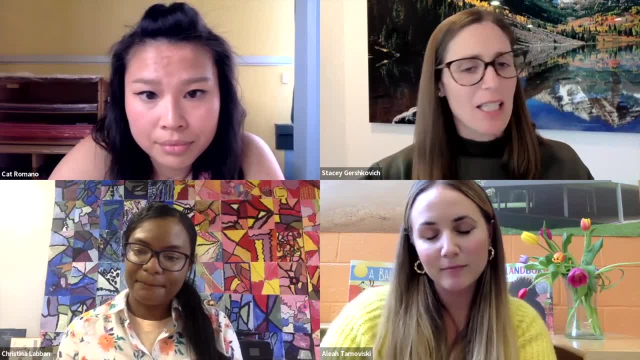 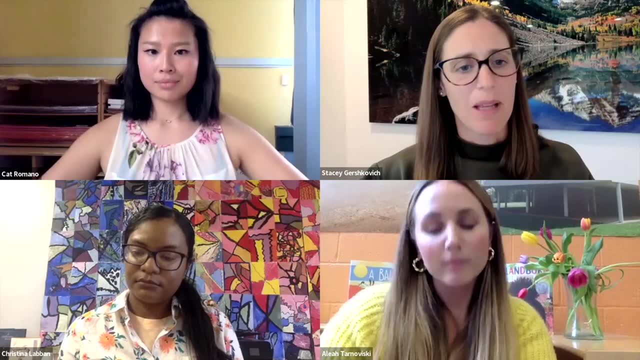 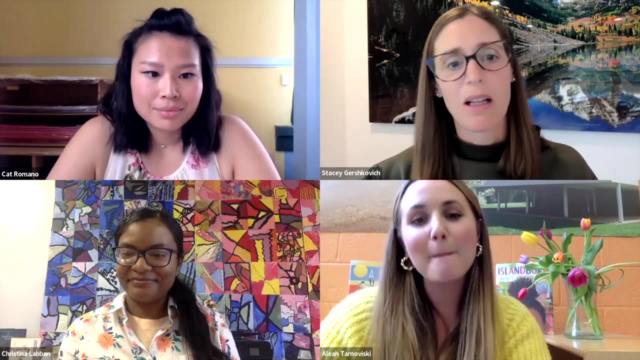 And I saw a question come in the chat earlier. but the expectation now is that you are reading to your child or someone is reading to their child, maybe an older sibling, maybe a family member, Maybe YouTube is reading to your child. You can Google a ton of read alouds and what's great is that they're all available. 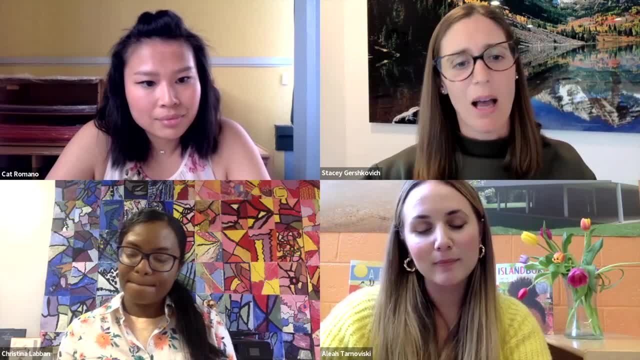 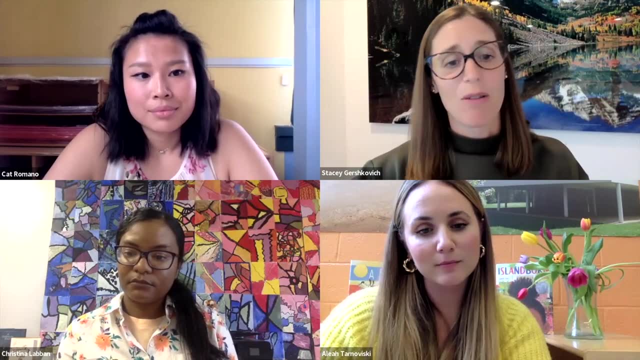 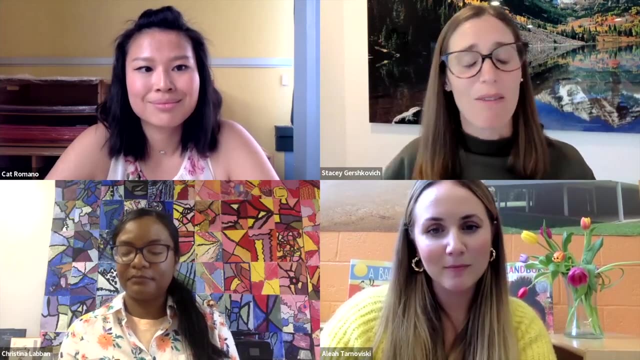 Your local library certainly has resources. There's obviously free apps that you can use that read books. I would also encourage families of English language learners to not stop reading in your home language. make sure you're also reading in that language as well. It's really great for children to hear both. 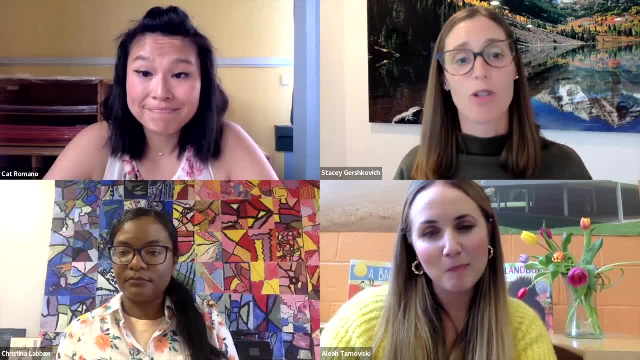 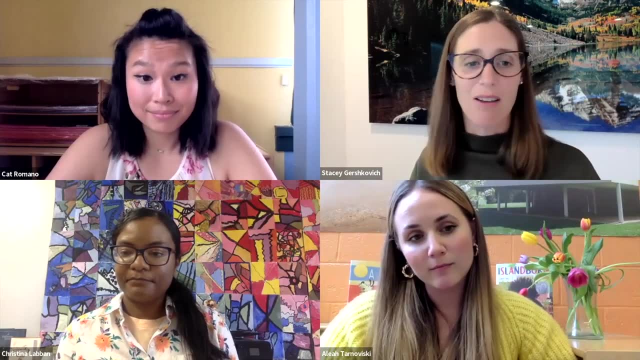 So read, expose your child to books. The expectation is not that your child is reading books to themselves at this time, although I know some kind of pre-K students can do that and want to do that. That's great, But now is not the time to pressure them. 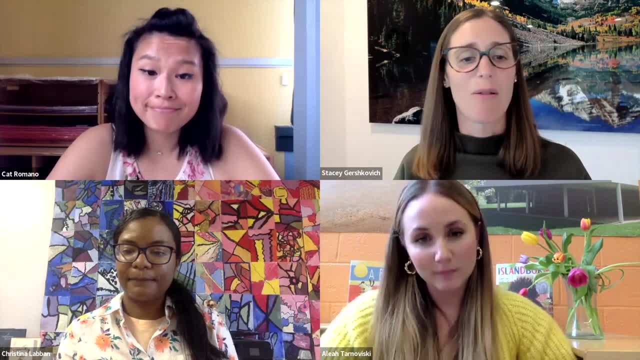 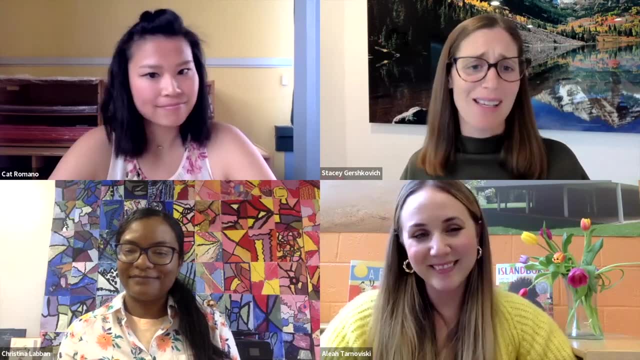 Yeah, But now is not the time to pressure your student to read independently. Right now is your time. maybe your child wants to flip through books. I always say you can read the pictures, right? My four-year-old's like I can't read. you're crazy. 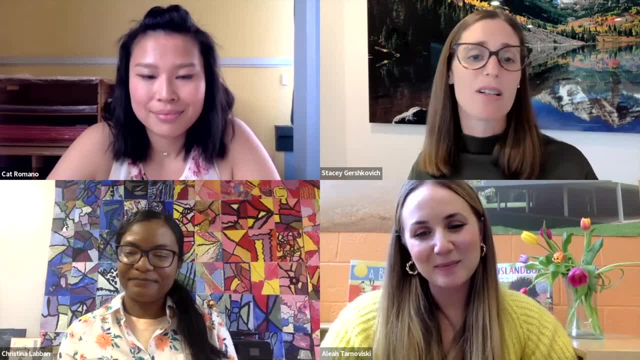 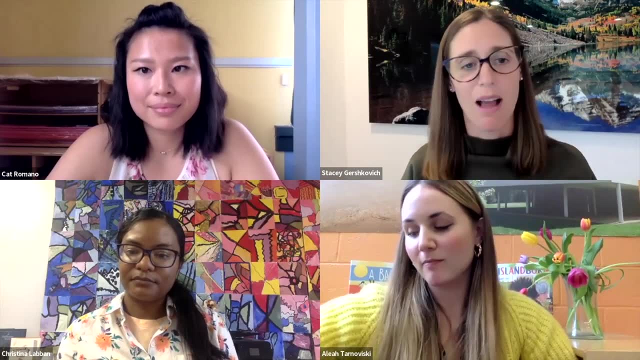 I said: well, you can read the pictures right. So giving them books that are familiar to them, that we've read a hundred times before bed, that they can go ahead and read the pictures, is a great way for them to get comfortable and own and get excited about reading books. 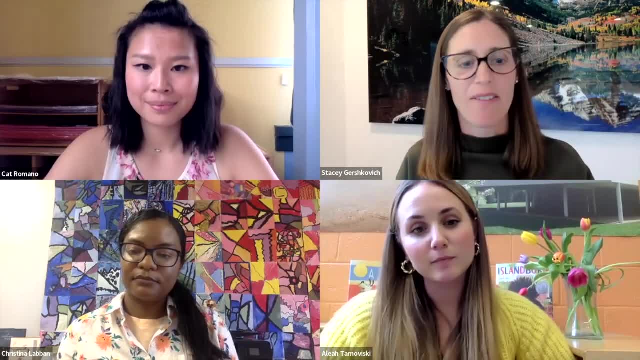 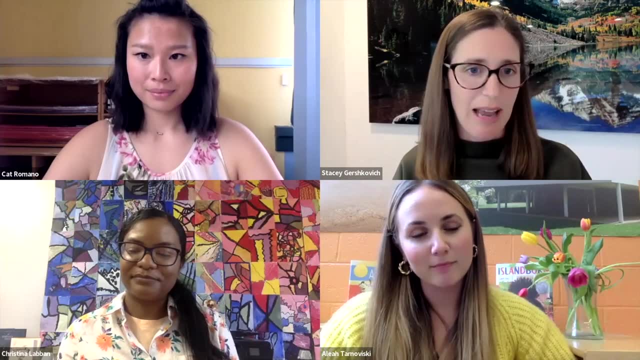 And we will put. We will share this later on, but we actually did an event on building a love of reading at your home a little bit ago, and so we can send that out in case anyone is interested in how you can develop that at home. 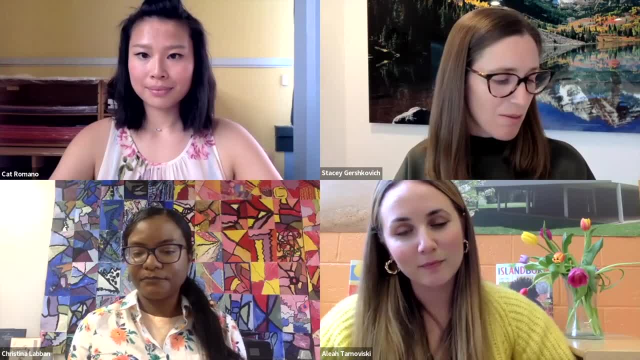 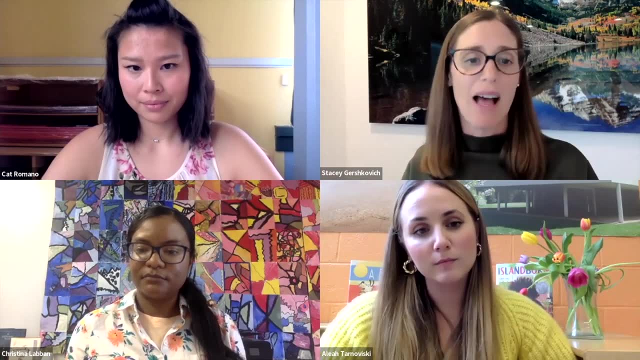 Okay, so we're almost out of time. There was a great question that we want to end with. Oh, before I do, technology. I know Aaliyah touched upon it. kids will have access to Chromebooks in school or to tablets in school, and they will be learning how to use them in school. 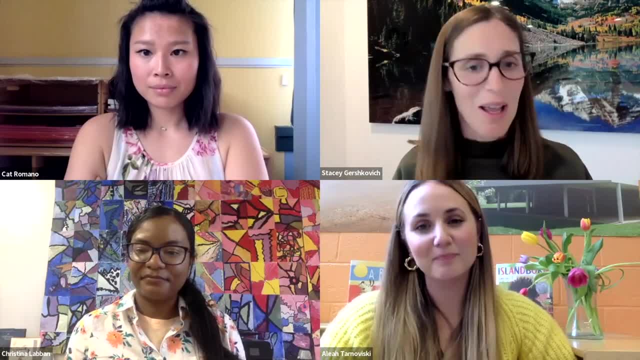 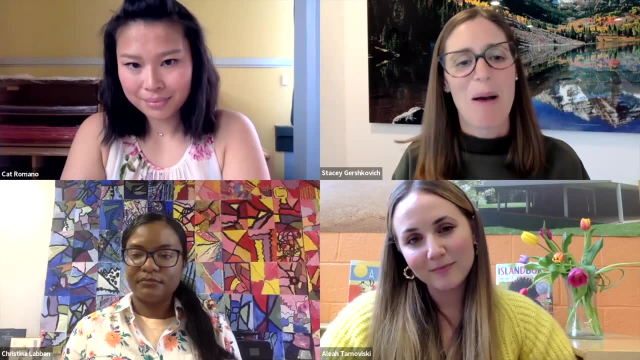 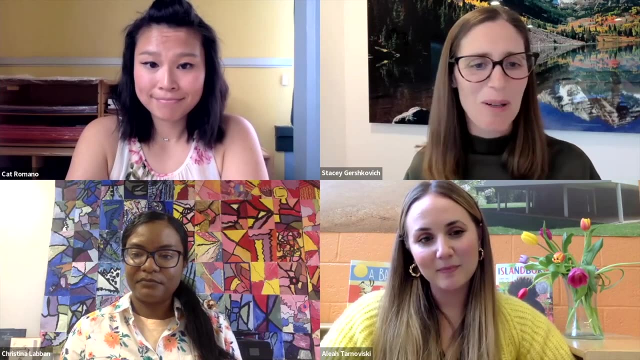 So yeah, That is definitely a part of their education. But we're entering kindergarten. I think we're really clear now that kids should enter kindergarten, excited about being in kindergarten and everything else will fall into place over time. But at the end of the year, where do kids leave? 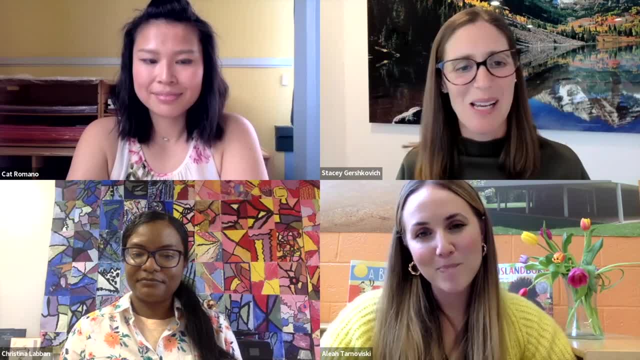 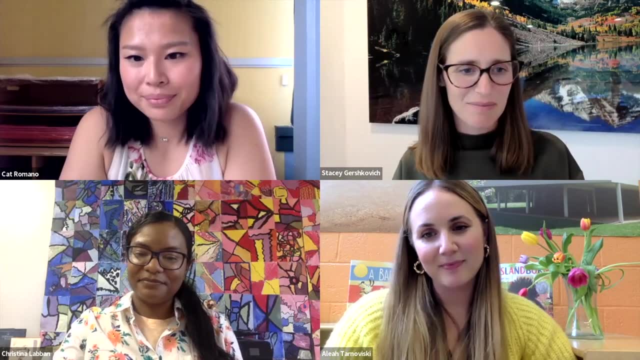 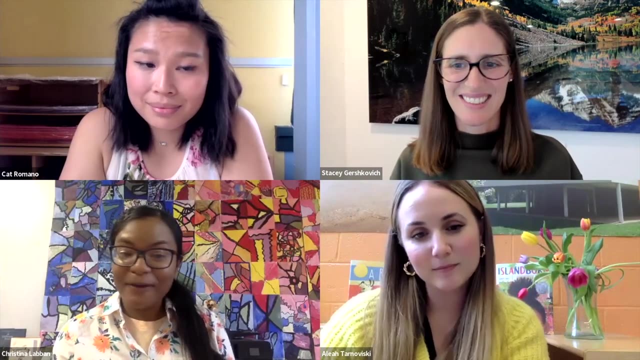 What are we looking forward to that, in one year's time, our little babies are going to be able to do when they're getting ready to go on to first grade? I'm amazed by how much my kids accomplished over the year. They now know how to skip, count by twos, fives, tens. 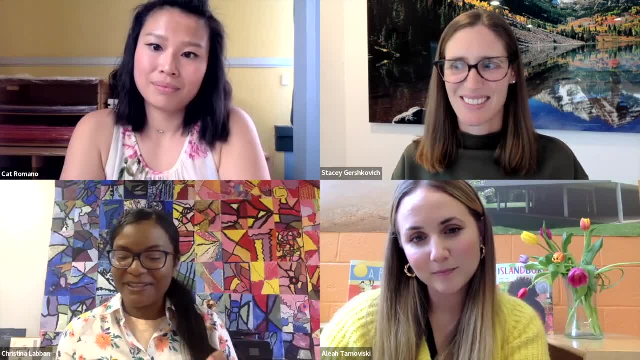 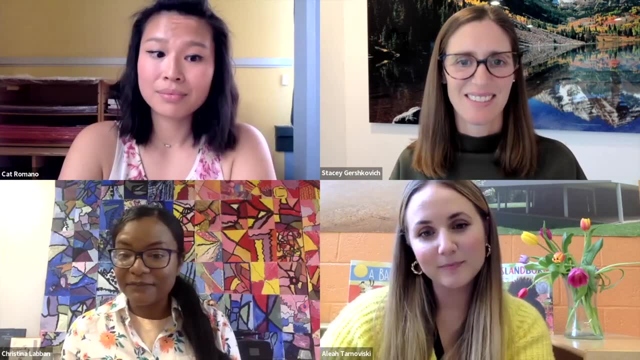 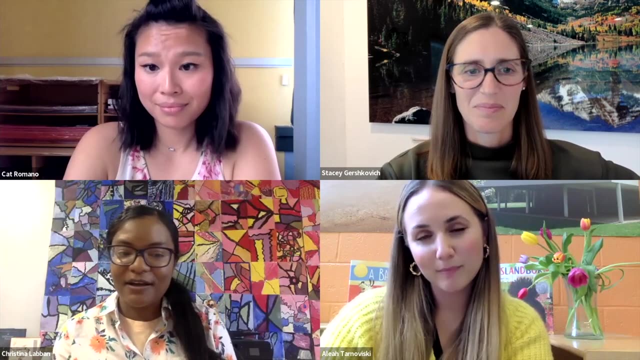 They know how to read. We start off in the beginning just learning about the alphabet and phonetic skills and things like that, But now we have kids who are reading level D books, level E books and beyond. They're excellent at mathematicians- just solving word problems. 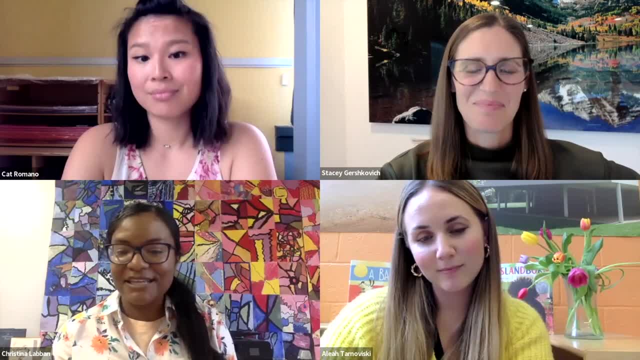 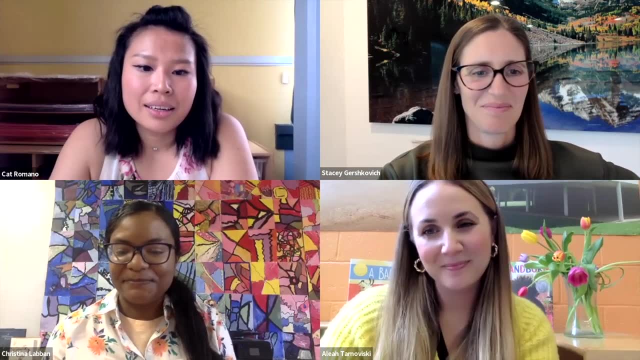 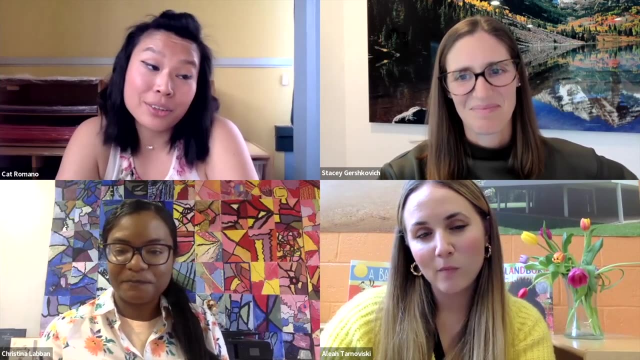 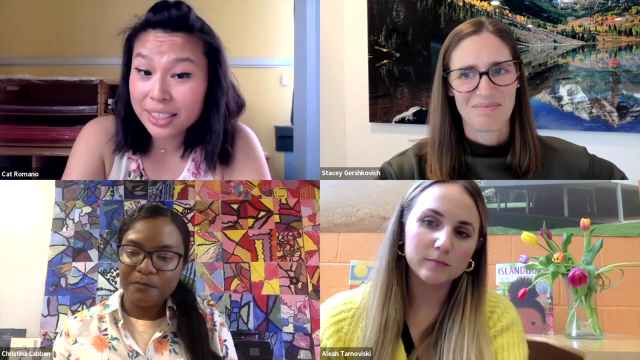 And just, they love doing science experiments, so they they've learned a lot over the year. um, yes, we, we do make a big deal about reading in kindergarten throughout the whole year. it's the conversation always come back about growing and learning more sight words. um, we use the Fountas and Pinnell level literacy system, so 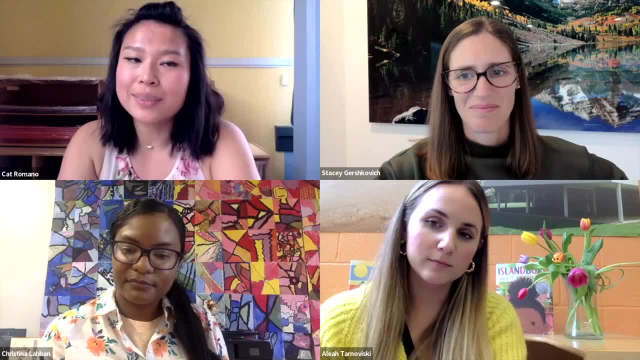 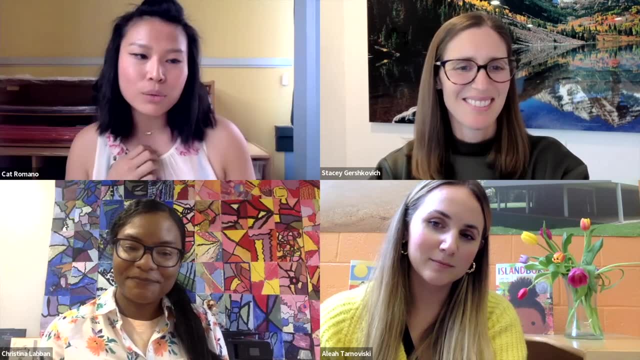 um in the like by the end of the year. we're all. the expectation is that our level d. but then our kids have just gone way past a level d and they're all like: I'm a level e, I'm a level f, and while to you that sounds like that, you don't know what that looks like on a page. but for level d's, 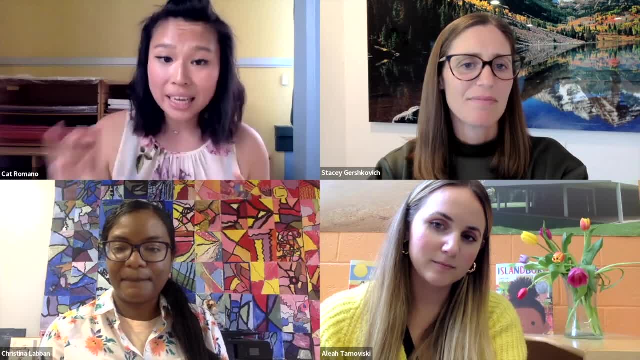 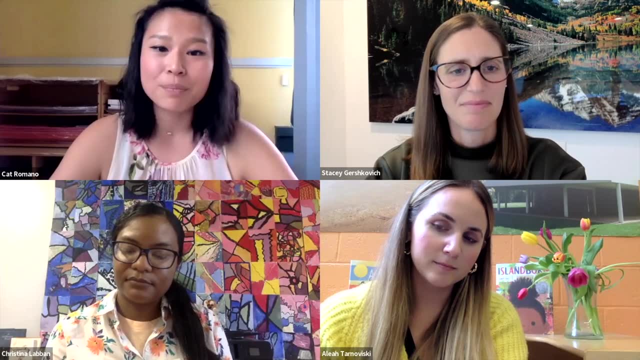 they know sight words, they know word endings, they can break down words, um, and they're just so authentically engaged in reading on their own. they don't want us to help them, they. they don't want us to tell them what the word is. they're just like: I can do it myself. I'm gonna do it by myself, just. 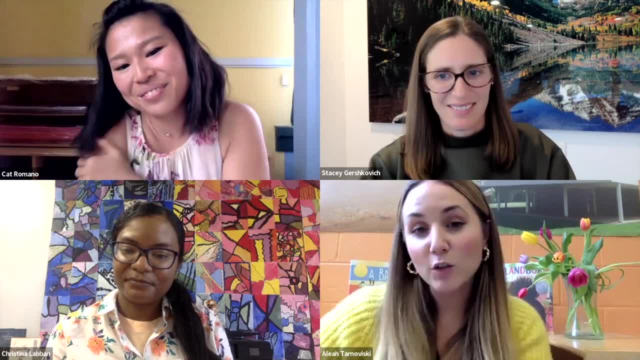 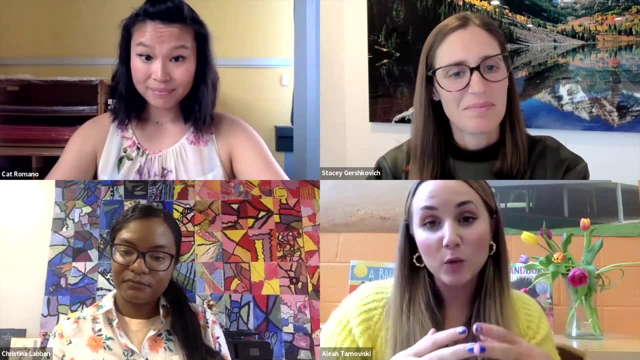 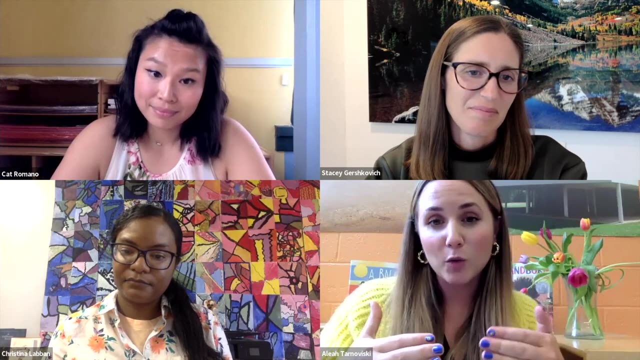 watch me. um, I also saw a question in the chat about, uh, how we teach reading, and Kat is touching on it. but, um, that's one aspect. so we have two parts of our day where we're really focused in small groups on reading, and the the first part of that day is called stepping stones, which is using success for 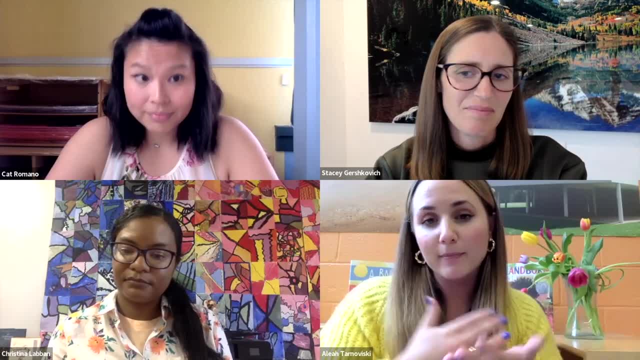 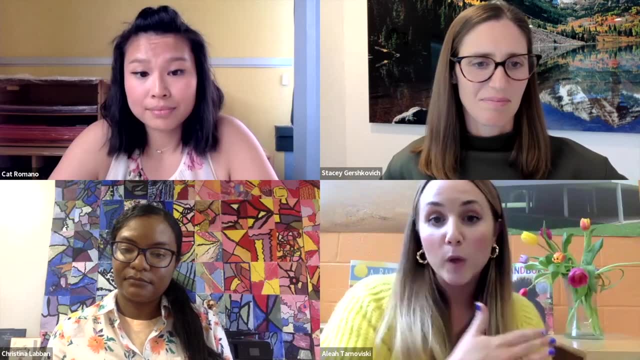 all curriculum to teach phonics and that is um science of reading based. so it's based on and how kids learn to read through sounds, through phonological awareness. so we walk them through that and then you start reading books and that part of our day is called guided reading. 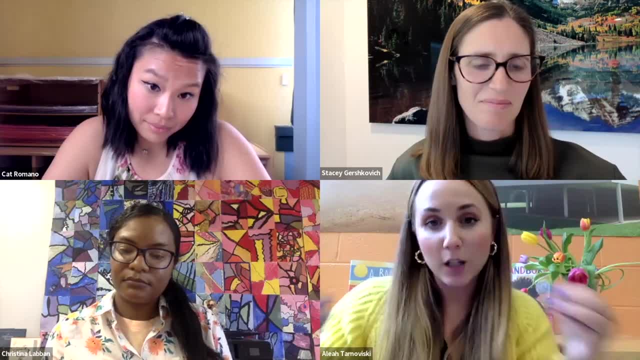 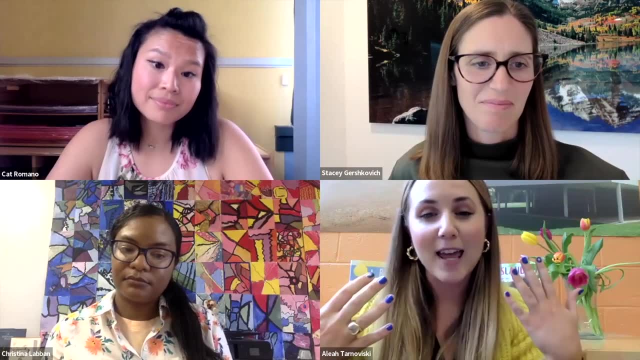 um, and that's where kids are grouped on, where they're at in their reading journey and they're reading books and they're really focused on comprehension and understanding characters and um cause and effect, things like that. so there's multiple parts in our day where we're really 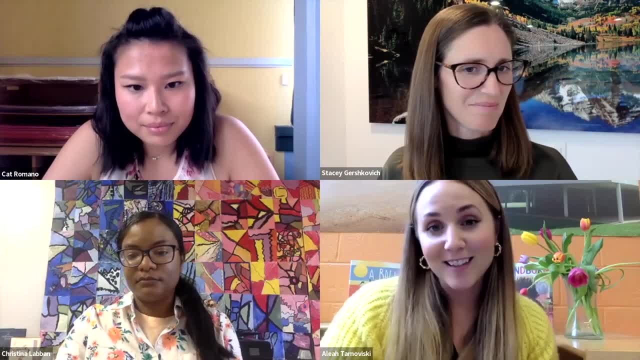 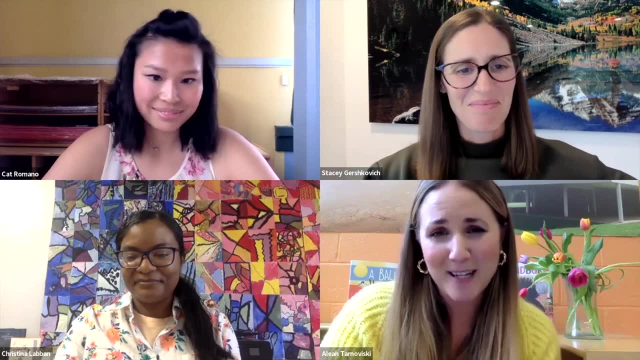 focused on reading. um, I echo everything that these ladies said about like. I look at them now. I'm like taking pictures of them for Mother's Day gifts and I'm like you're grown people, you're not babies anymore. like I have pictures hanging of them from the first day of school and I'm like 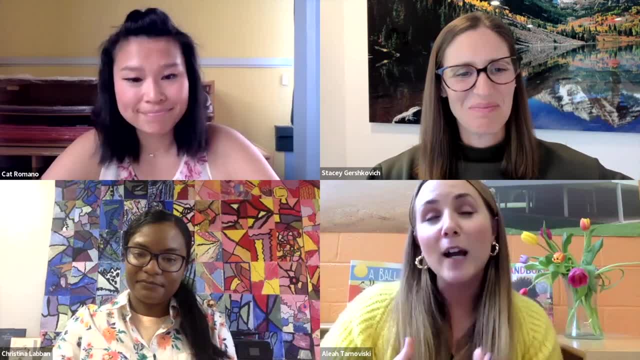 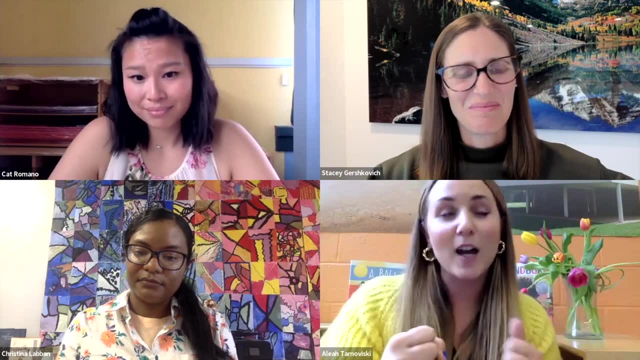 they're like real people, um, and they're so ready and I think what's so cool, um, as someone who teaches in a special education classroom? right so I have scholars with IEPs and I have um general education students. I also have kids who spoke no English when they came in, like they're all. 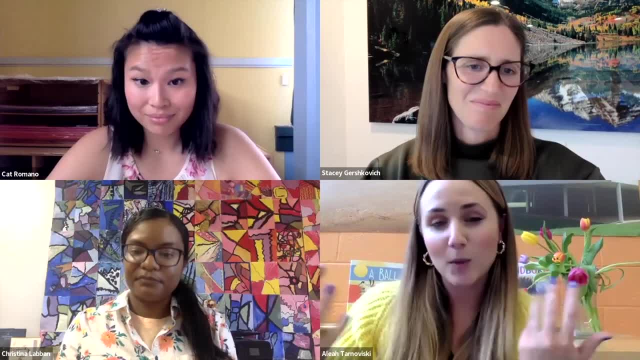 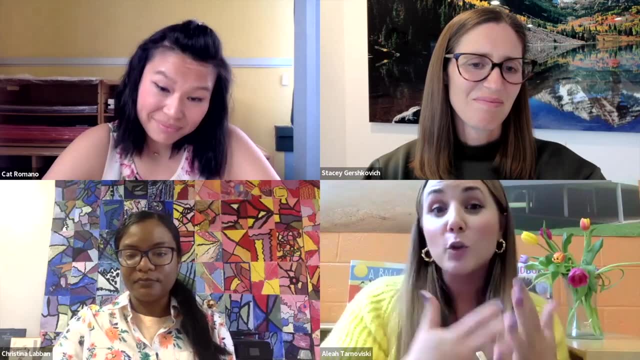 able to do these things that Kat and Christina are saying. they're all counting to 100. they're all counting by groups of 10. they're noticing things about place value. they're all reading um sentences, they know their sight words. they're able to write stories like that is. 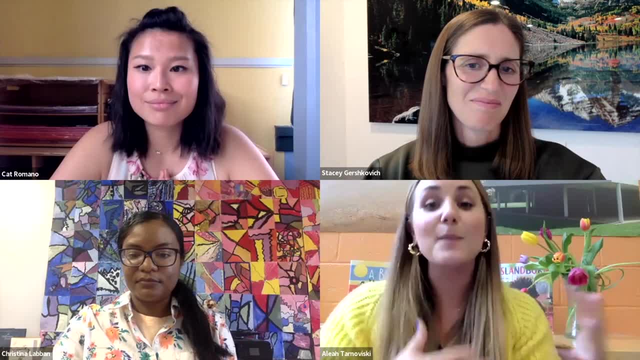 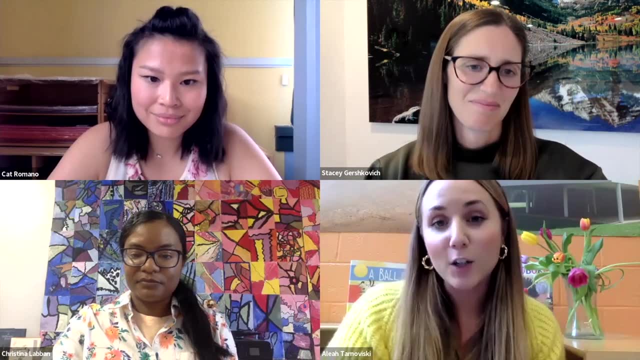 what I'm saying for all of our kids, and they all came at so many, came in at so many different levels, and that excitement about like watching that journey happen for kids is what's so amazing about being a kindergarten teacher and so, um, like hear what we're saying about where we're sending. 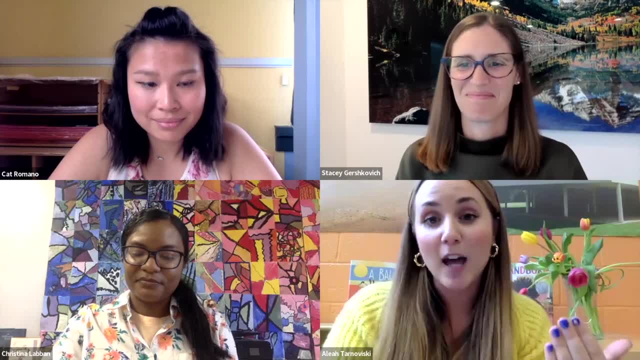 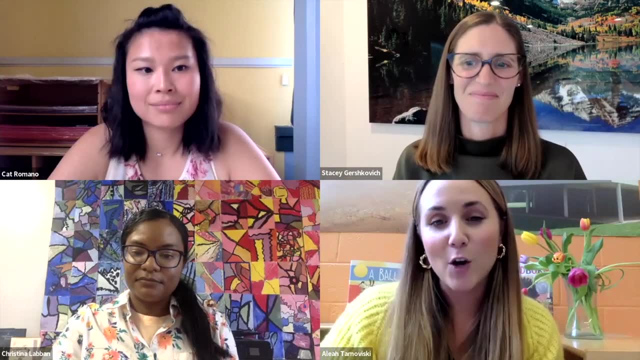 them like how we're sending them off to first grade and be encouraged that every kid came in at a different spot and they all got to where they needed to be and so many are beyond um and so they're all. they're all ready, yeah, and they're also all really independent now. 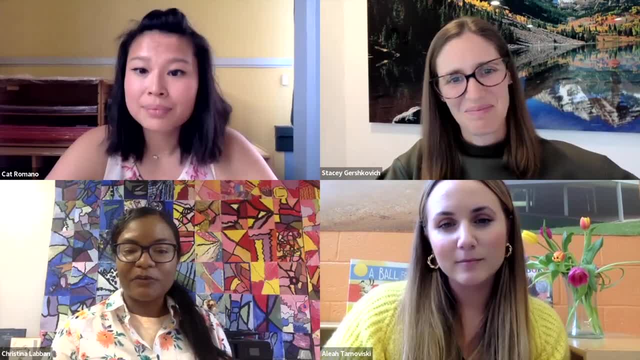 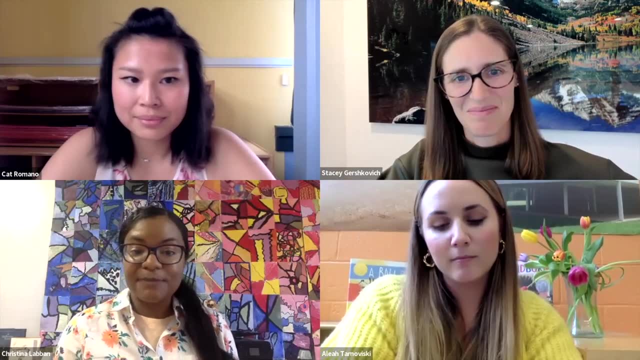 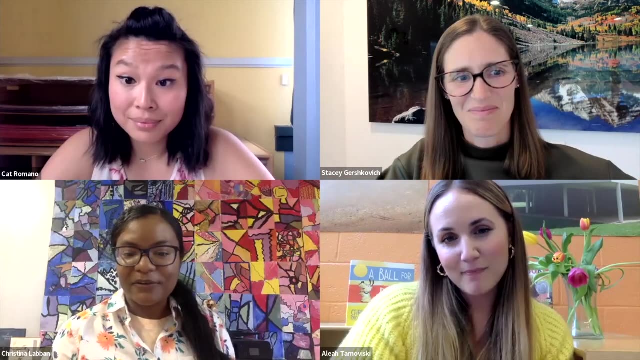 they can go do things on their own. um, they know our routine. they become little teacher helpers. um, they also are able to discuss and debate with each other now and speak in full sentences. so they're definitely, um, you know, grown so much over just a space of a year. yeah, all of this is so. 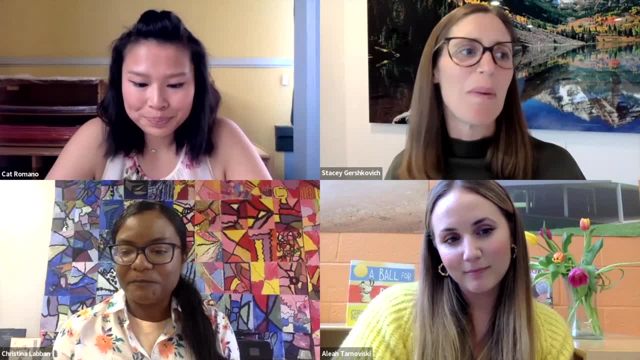 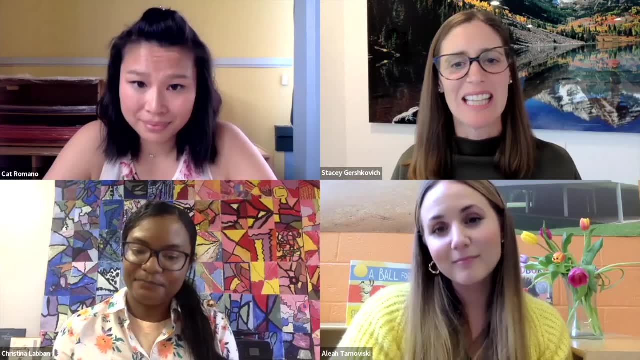 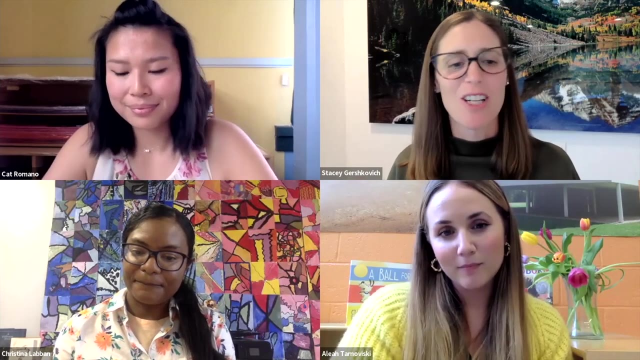 helpful. I think, yeah, the big takeaway that I hope everyone has, that I have for my own child, is that kindergarten is really the foundation and the goal here is to get our kids as excited as possible about learning. that is the purpose of kindergarten, because if our children are excited about learning,